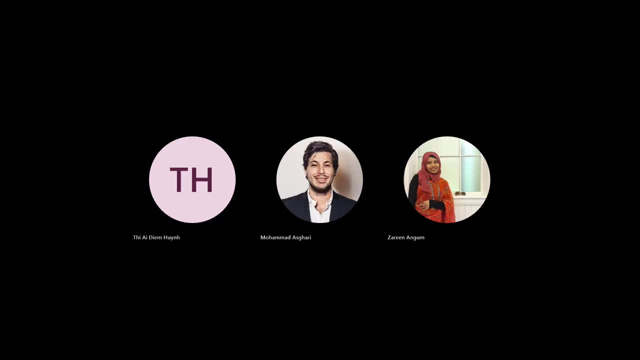 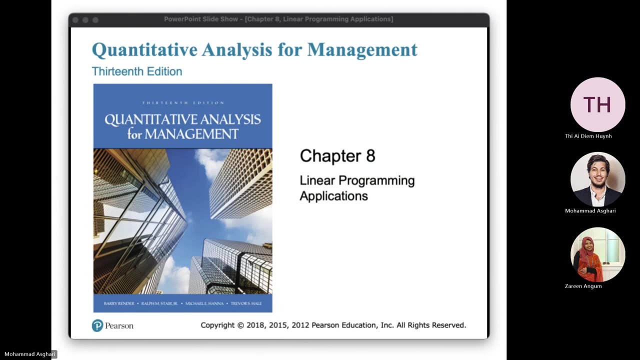 If you want to learn about linear programming applications, how can? whether we have them implemented to solve it, or graphical or corner points, so how we can apply them in real world problem, And this is the most interesting part, because solving is something that you can hire. 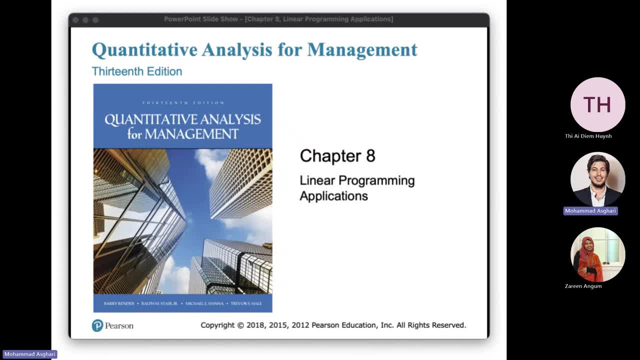 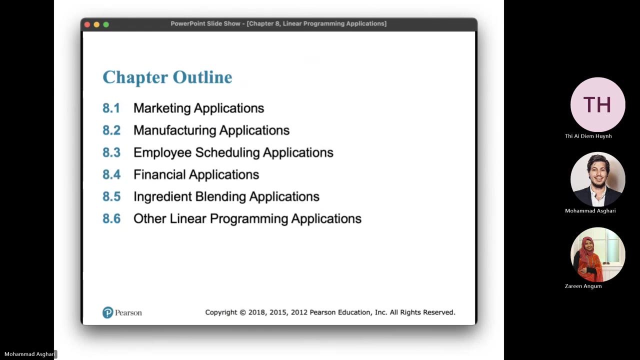 or use software to solve it, like Excel, MATLAB or any other software, But the art is modeling. Modeling is not something that a computer can do for you. This is your brain and that, if you use it, you should find a good application. 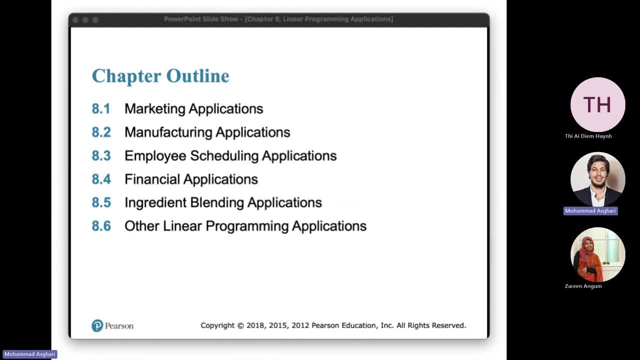 Okay. so there are lots of applications that linear programming can be applied, For example, marketing in manufacturing, employee scheduling, financial applications, ingredients blending and others. So ingredient blending looks a little bit familiar to you in manufacturing. So, if you remember, in the manufacturing case we were talking about the number. 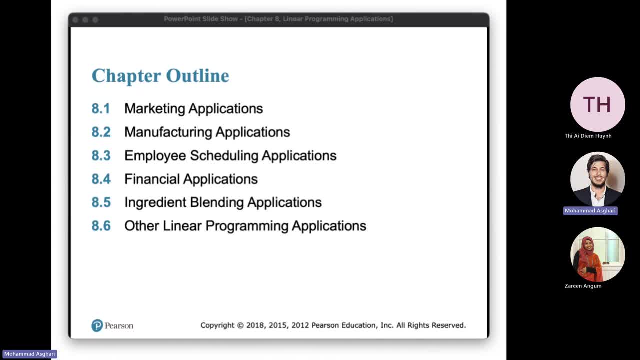 of tables and chairs, So how many of them should be made in order to maximize your profit? And in gradient you were thinking thinking about. you know different combinations of materials in the food, So how much you should buy from each component so that you know in total maximize nutrition of food. So we are familiar with these items. 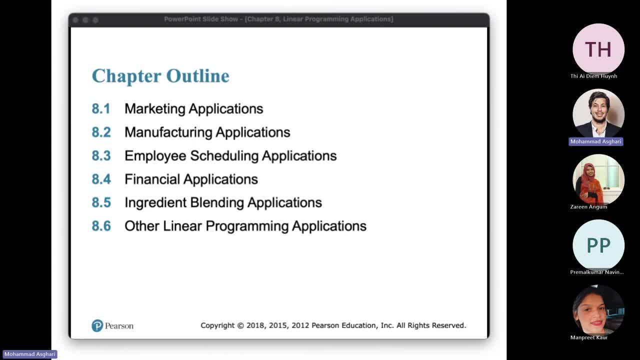 So we want to start from other types of models. Probably we will Skip this one Because you are already familiar with that. So we will start with marketing and then employee scheduling, financial a little bit, And we will try to review ingredients again because this is a very critical problem. 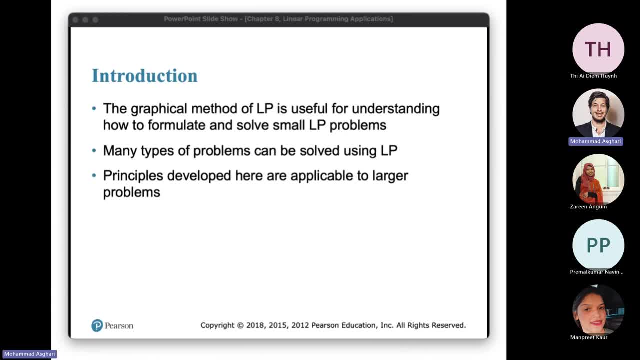 Okay, so definitely we cannot cover all of that in one session. What we are going to do is to do our best to learn as much as we can today. Introduction: The graphical methods of linear programming is useful for understanding how to formulate and solve small linear programming problems. 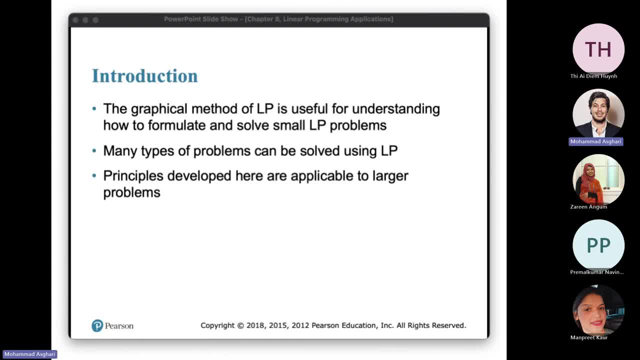 But many types of problems can be solved using LP or linear programming, So there are a wide range of problems that you can formulate using linear programming. So principles developed here are applicable to larger problems. So so far we learned how to do for small ones. 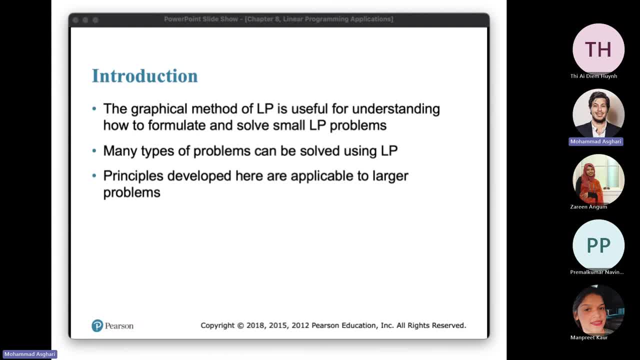 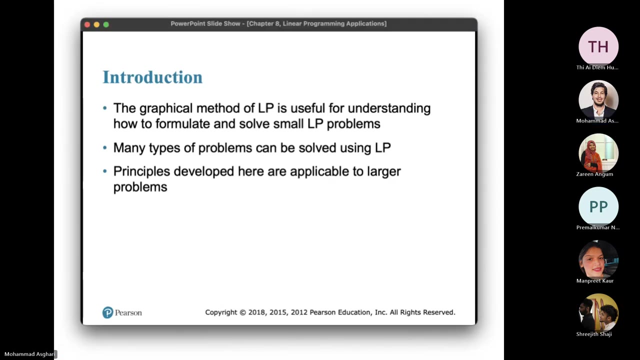 Now we want to learn modeling for large cases. So that's the idea, But don't get a search of larger. It's not much different because the concept is the same, Just a little bit changing that, you know, the number of variables and something like that can change. 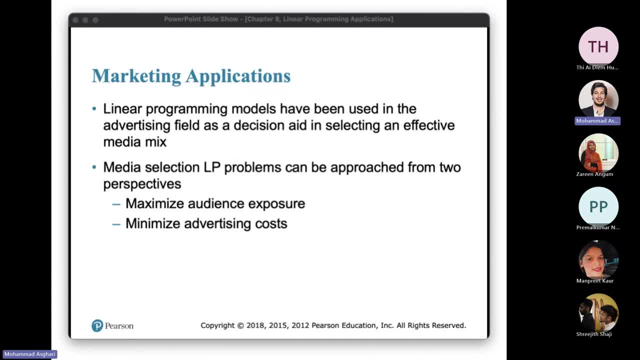 The first application that we want to cover today, Marketing application. This is one of the most fundamental applications of linear programming And you know they have been used for a long time in advertising and marketing environments. So what is the idea? So the idea here is that we have several tools or advertisement methods and each of them has a kinds of cost, a kinds of audience. 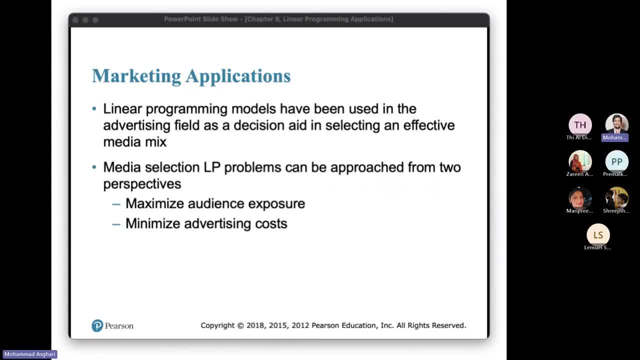 Okay, For example, if you use newspapers or certain type of people, maybe older age, they really like to read newspapers. So there is a certain number of people who are reading newspaper and advertisement. newspaper has a certain cost. The same, you know, may go with radio. 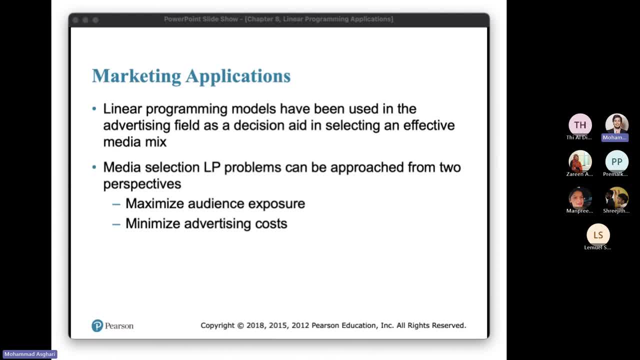 There are certain type of people who likes to listen to radio, And that's also came at a cost. or maybe certain type of people watch TV at different times of day. So, as you can see, there are different types of tools for advertisement. So what is the goal in marketing application of linear programming? 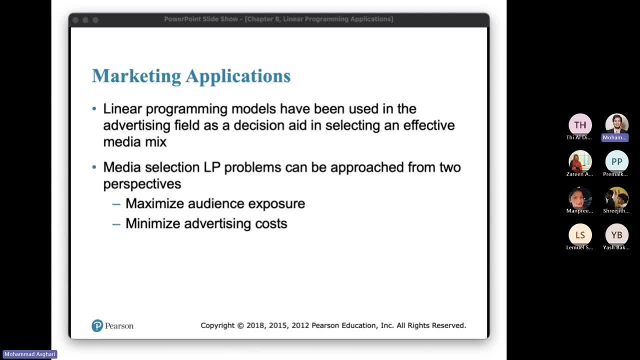 We may have two totally different objective functions, As you can see here. The first one is the maximum maximization of audience exposure And second one is the first one is try to maximize the number of people who want to watch or read or listen to advertisement. 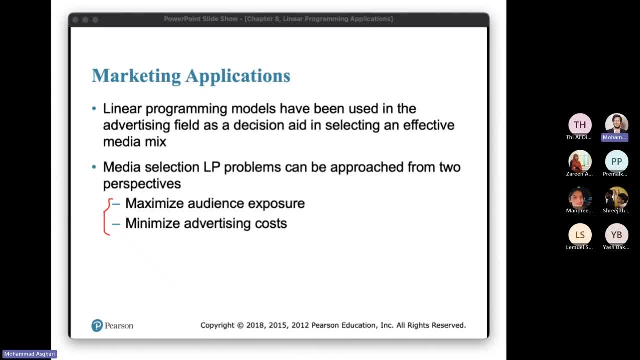 So maximize the number of people. That's the first objective. What is the second objective? that in marketing application we may use? Minimization of advertisement. cost. So Radio cost You. So radio cost You. searching amounts: newspaper the same, TV the same. 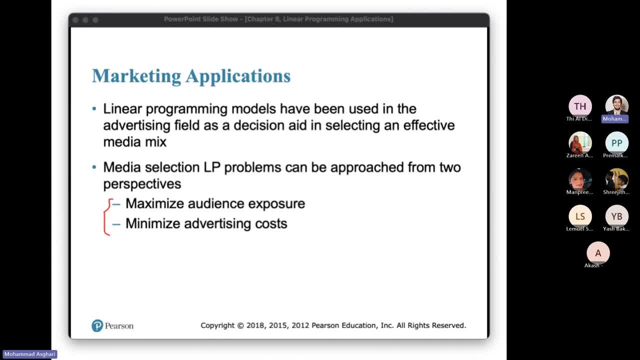 So how can we minimize the total cost of advertising? Two totally different. Can we use both of them at the same, But not in this course. So we cannot use both of these objective functions in one model in this course, But in real application sometimes can use several objective functions as well. 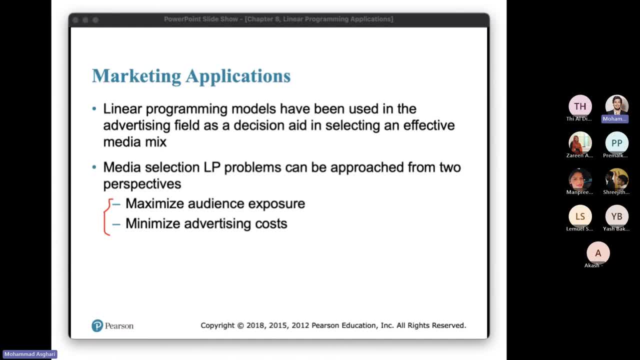 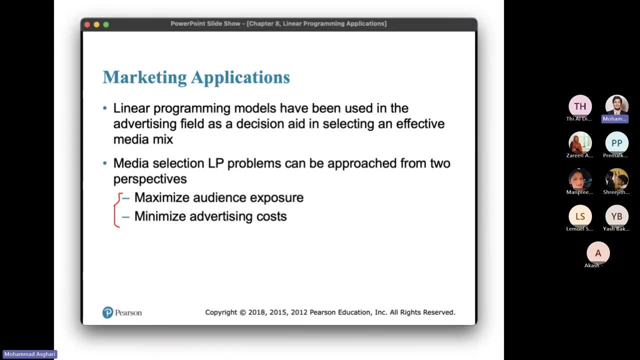 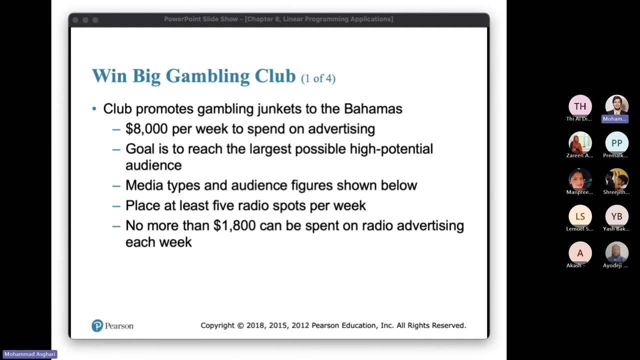 So the problems that we want to solve here are using either this one- Maximization of audience exposure- Or this one, Minimizing advertising cost. Not both of them, Okay. So let's see, There is a company of gambling club. 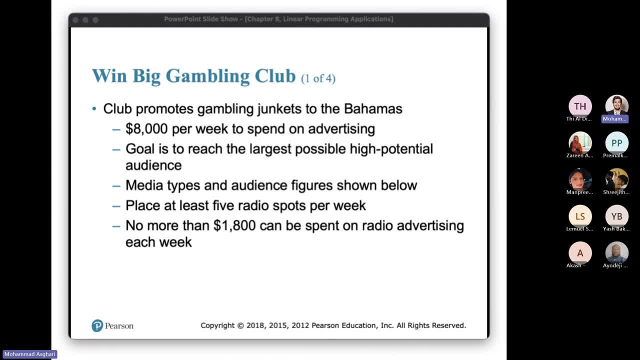 So gambling club promotes gambling junk Junkets on Bahamas. So they have a budget of 8,000 per week. Okay, So this is the budget that they consider for advertising. This is the maximum that they can spend And the goal is to reach the largest possible audience. 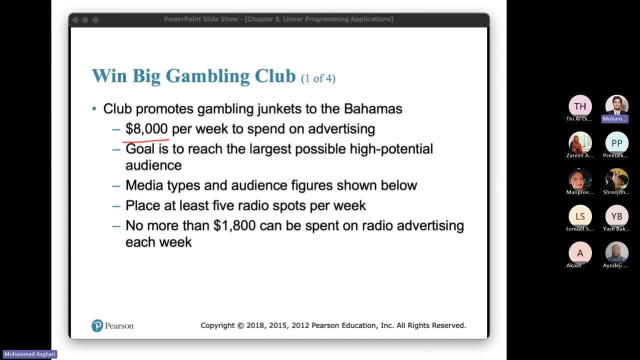 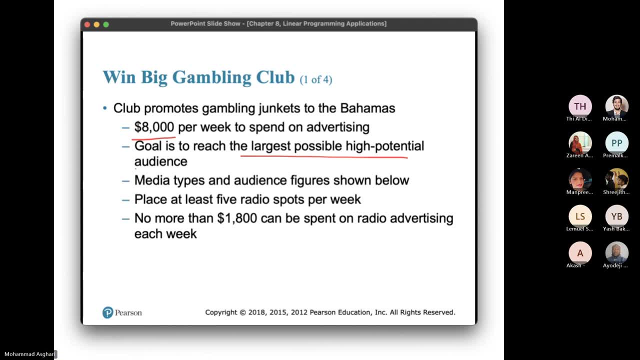 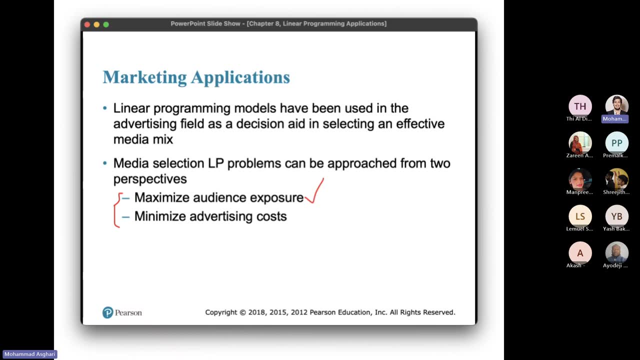 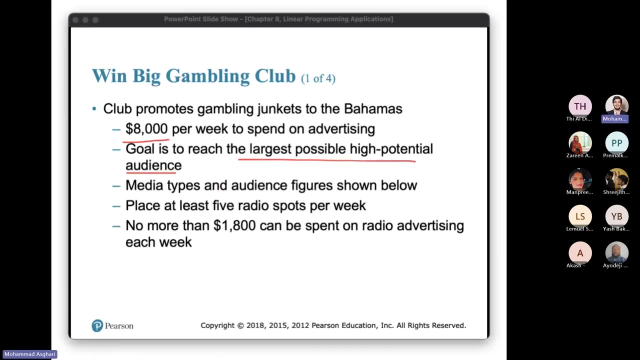 Okay, So, if I go back, The largest possible audience. As you can see, They are trying to address this one, This objective function. They're trying to maximize the number of audience. So we found that the objective function is maximizing audience exposure. 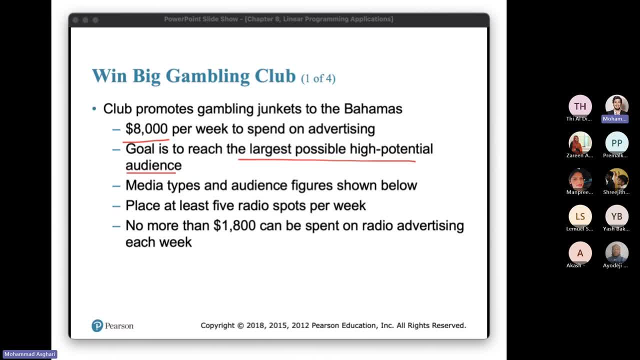 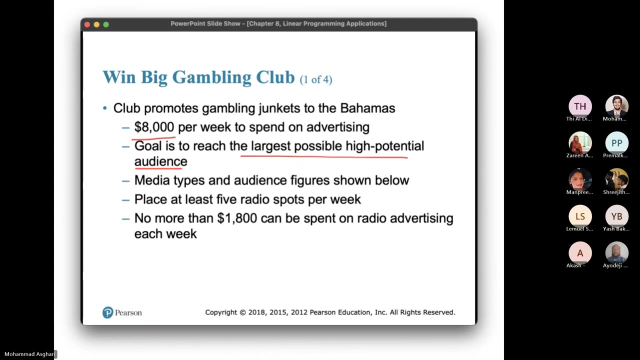 Okay, There are different media types and audience, as shown in the next slide, So there are some conditions as well. We need to meet them. What are these conditions? Place at least five radio spots per week. Five radio spots We are talking about at least. 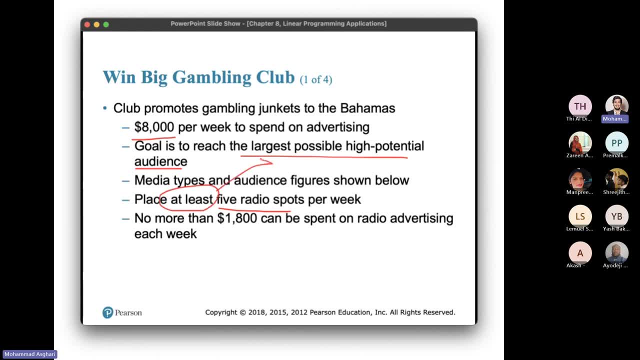 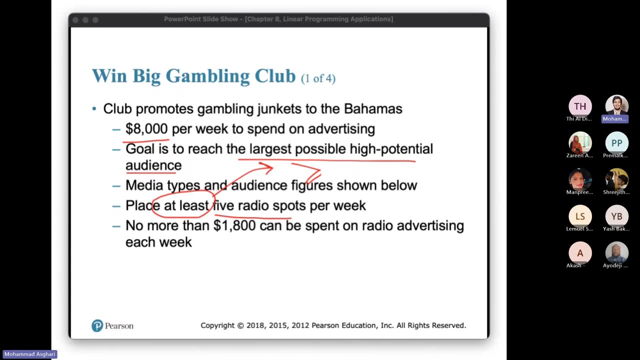 So we have to use this sign That must be greater than or equal to this sign. Okay, And So it looks that the manager has decided to make sure that at least five radio advertisements are placed To put To make sure that certain type of people are listening. 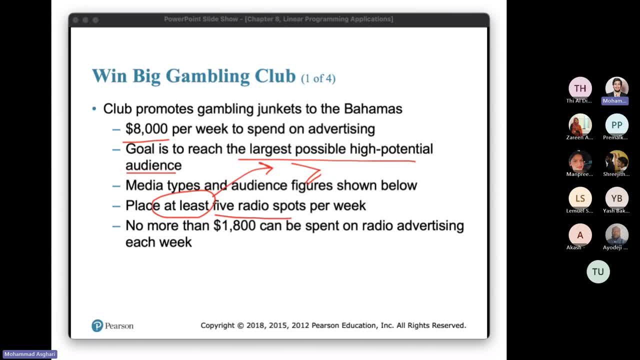 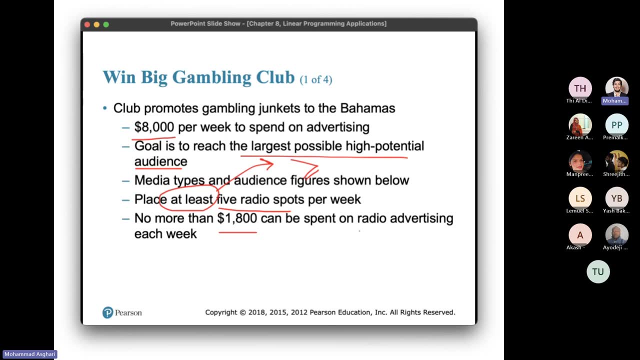 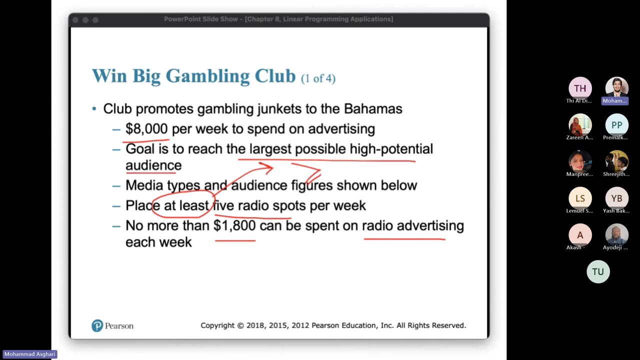 Okay, So this is the first one, The first condition. What is the second condition that manager wants us to do? No more than 1,800 can be spent on radio advertisements Per week. Okay, So a minimum of five radio advertisements. 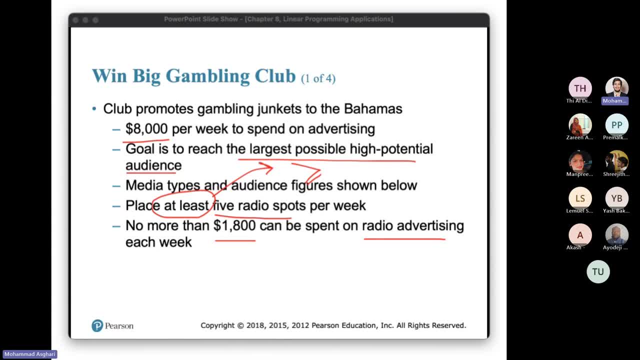 And not more than 1,800. Per week. So two different conditions, And both of them Are related to radio. When we are talking about conditions, These are, You know, Constraints Actually. So you know What is the objective function. 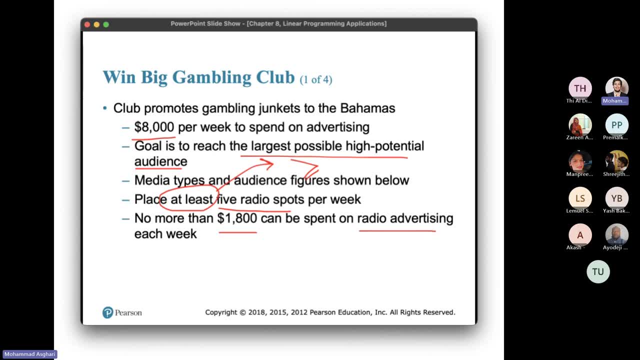 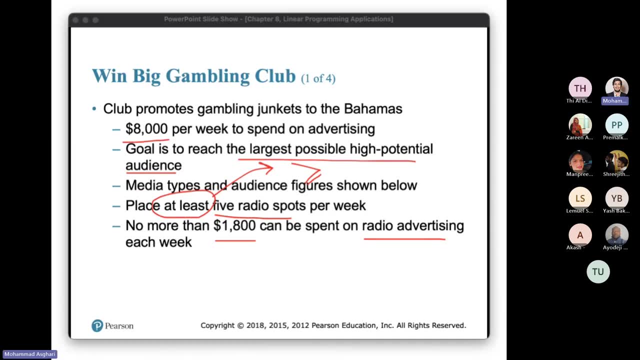 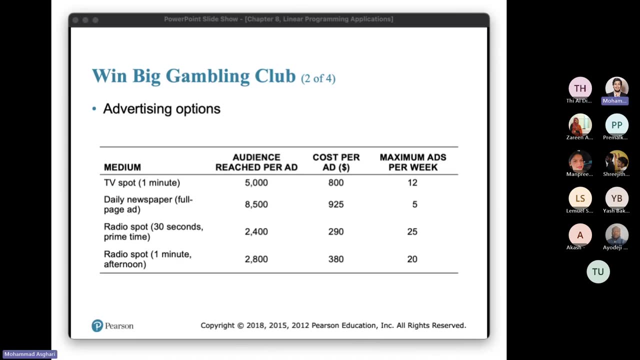 The maximization of the number of audience And what is the Constraints. Okay, So Let me Show you The table. Let's see how To model it. Before going there, We should see What is the table. 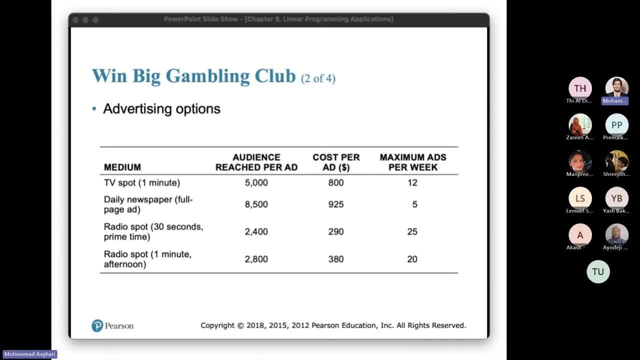 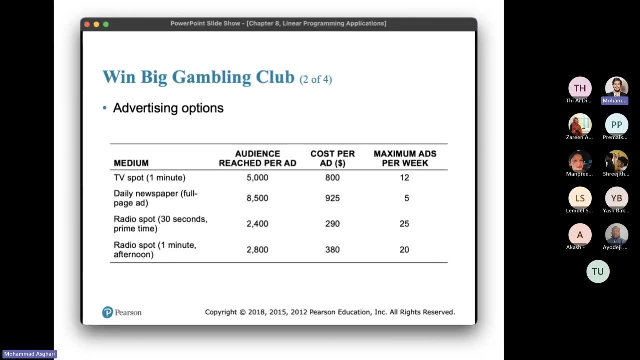 That is talking about. This is very interesting. First of all, You see different mediums, Different advertisement tools. You may use TV Spas One minute. You can see Different mediums Here For different Options For advertisements. 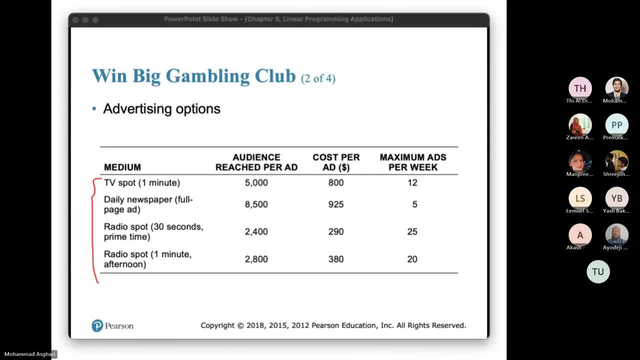 You may use Daily newspaper, You may use Radio spot Which is In prime time Radio spot, The last one Which is In afternoon. Okay, And each of These Four Different Media Have Different topics. 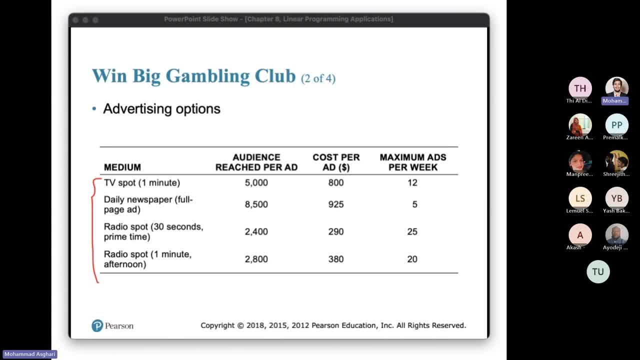 For Radio: Okay So. So You have Different types Of Audience. Okay So TV, Normally Each time That You Advertise On TV. So The Five Thousand People, 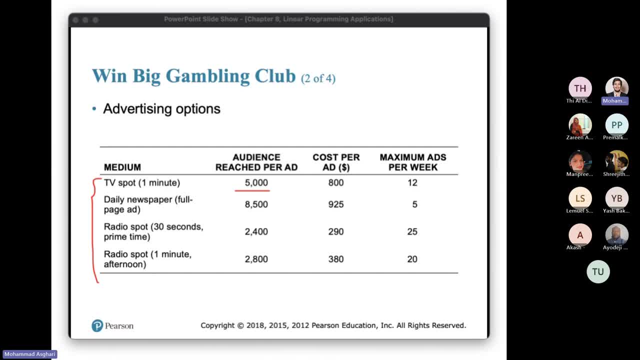 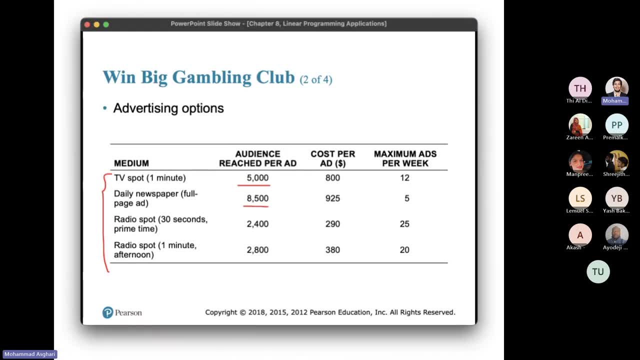 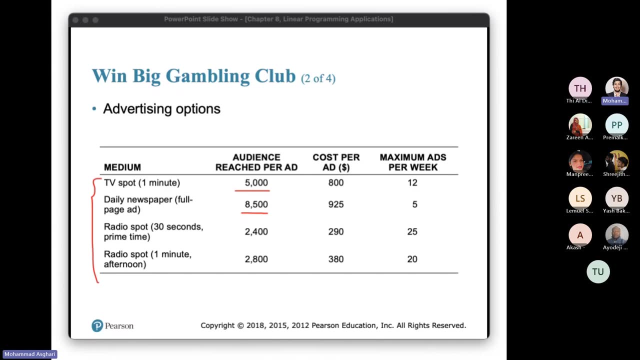 Watch It And When You, Each Time You Advertise On Newspaper With Your Advertisements So You Can See The Number Of Audience In Different. 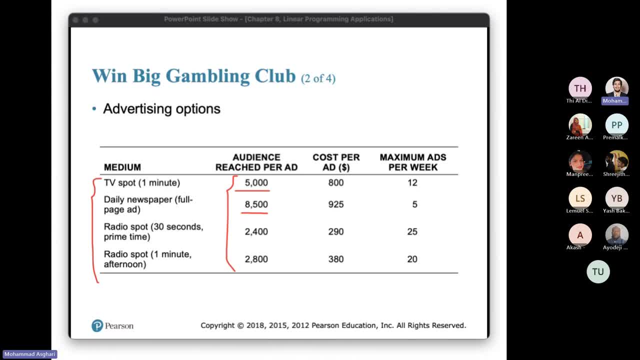 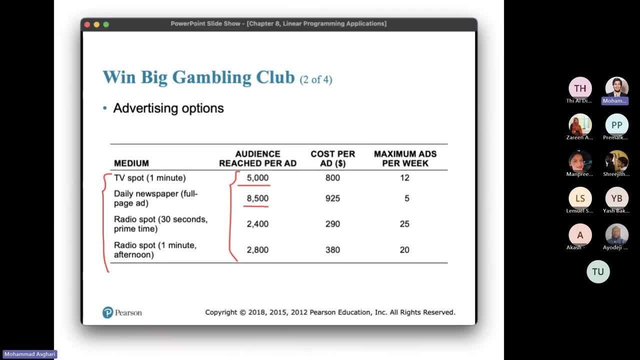 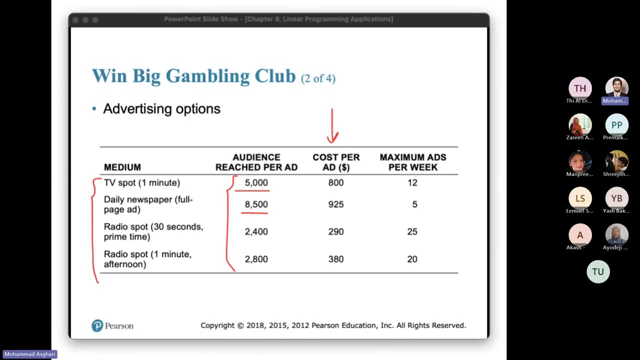 Media. And So And Look At This Column, This Column Talk About The Cost, This Column: Each TV Cost You Eight Hundreds, So A Newspaper 925.. 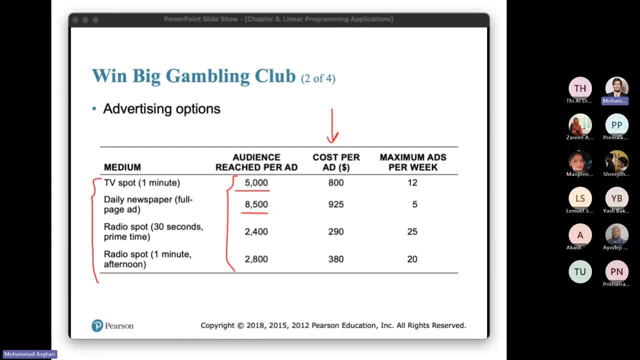 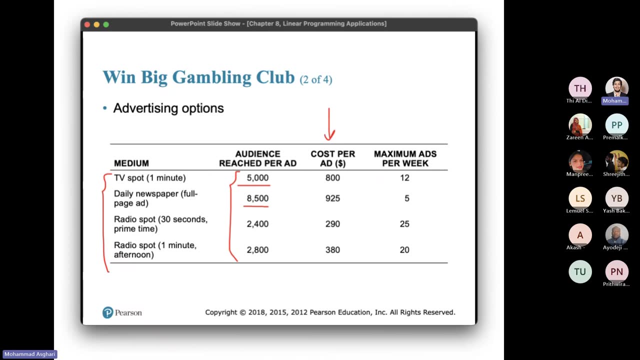 Up To The Last. So There's A Limit In The Last Column. You Cannot Put All Of Your Money On Daily Newspaper. You Can Act. 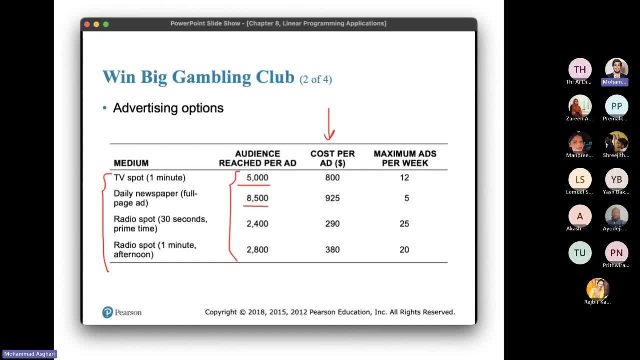 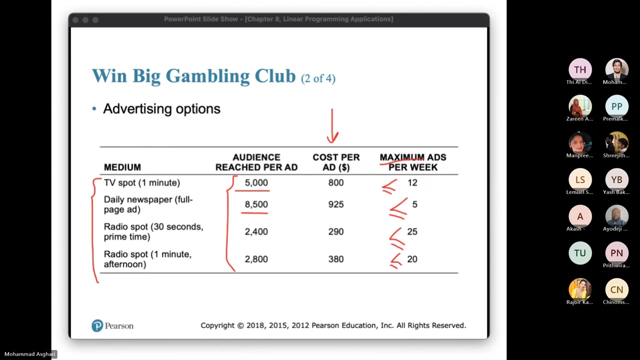 Maximum Pay For Advertisement On Newspaper Less Than Or Equal To, But We Are Talking About The Maximum. We Should Use This, Okay, Remember So We. 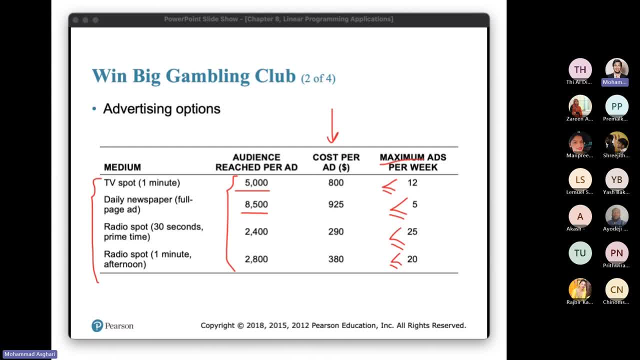 Understand The Problem. This Is The Process. What Is The Next Step? I Want To Model It. Do You Have Any Step To Model It? To? 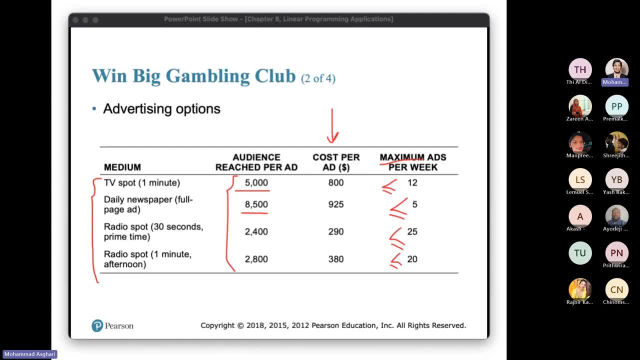 Write A Mathematical Model For That. I Remember Chapter Seven. So The First Step Is Understanding The Problem Completely. So Okay, I Guess You. Decision Variables. 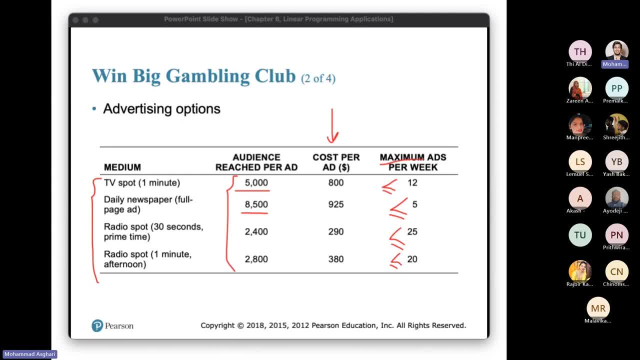 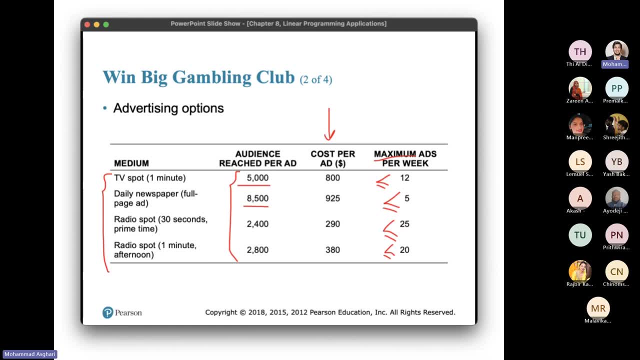 Okay, So This Decision- Variables- Should Be Decided At This Moment. We Can Decide This Variables In This Way On This Place. Can This Define? 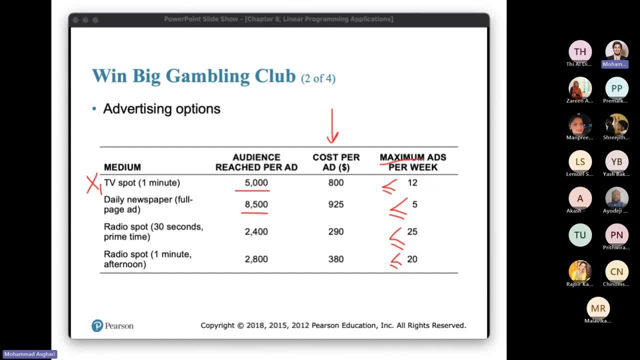 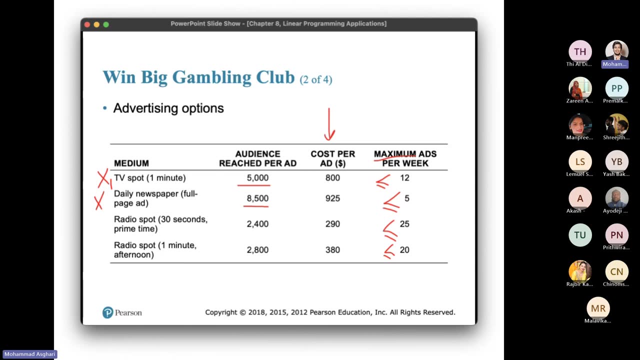 For Decision: Variable. This Is The Number Of Times That You May Use TV Spot Okay TV As Advertisement, So It Could Be X1.. 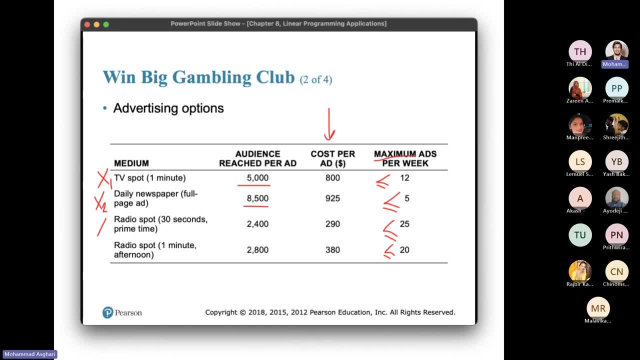 And X2.. The Number Of Times, That's You, Are Defined. As You Can See, We Have Two Radio Spot Here, But One Of Them Is 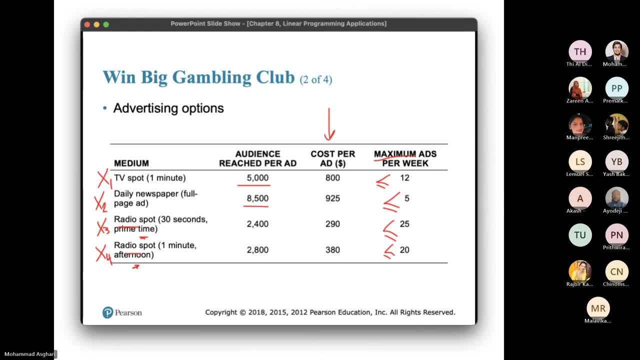 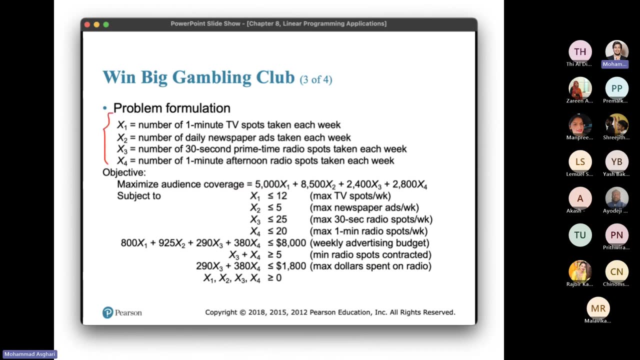 Prime Time And Another One Is In Afternoon With Different Number Of Audience. So Each Time You Advertise On TV Spot X1. To X4.. 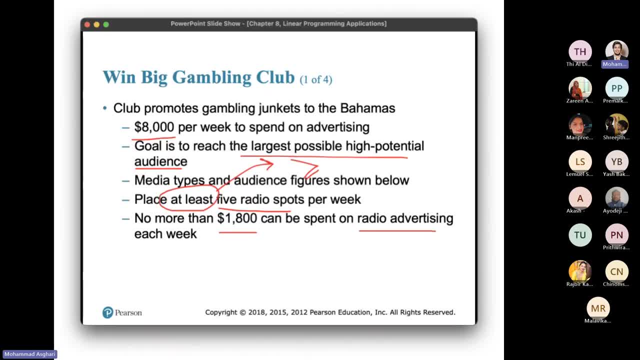 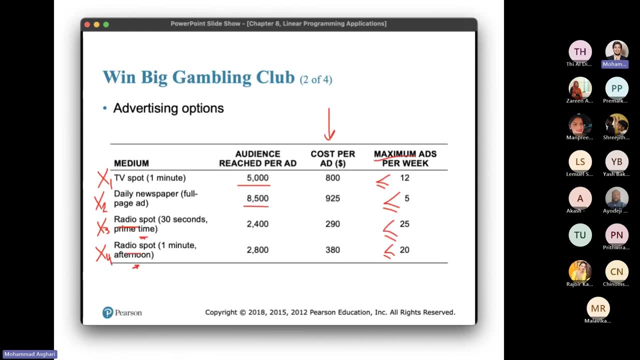 So The Next Step Is Writing The Model. We Should Write The Objective Function. What Is Objective Function On TV? Five Thousand People Watch It. 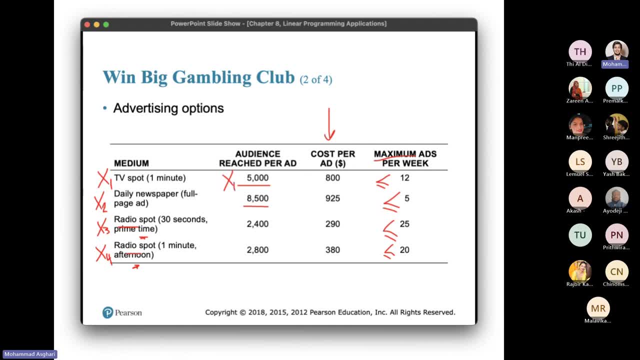 So We Should Multiply The Number Of Times You Advertise On TV. Multiple Five Thousand The Number Of Times You Advertise On The Objective. 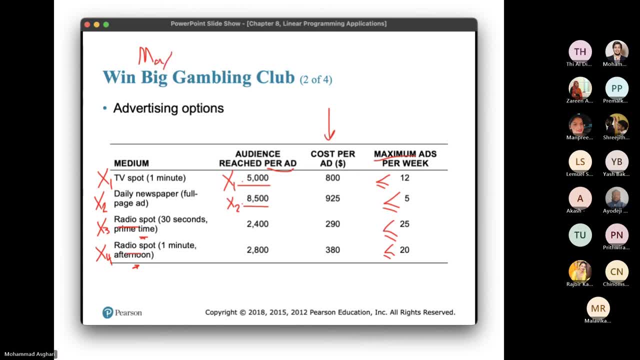 Function In This Way. Maximize Of There. It Is Equal To Five Thousand Multiple Less, To Thousand Eight Hundreds Multiple Expo. So We Have The. 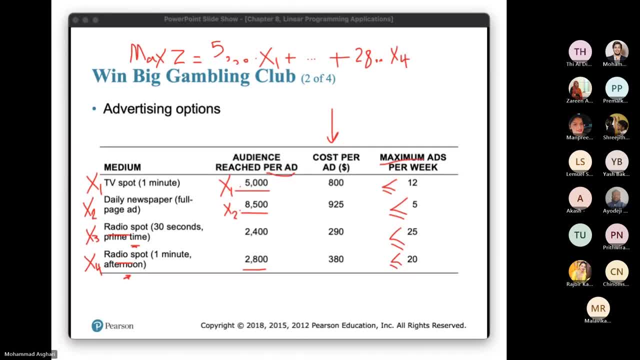 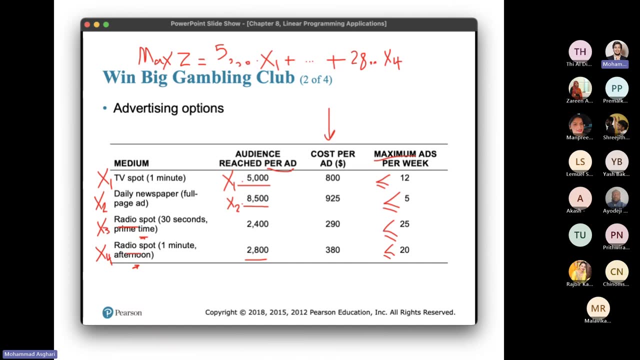 Objective Function Of Times, We Have Some Conditions That We Should Make. First Of All, The Number Of Advertisement On Each Medium Can Not Exceed. 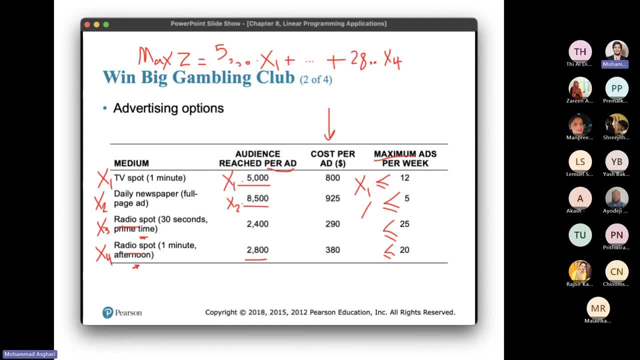 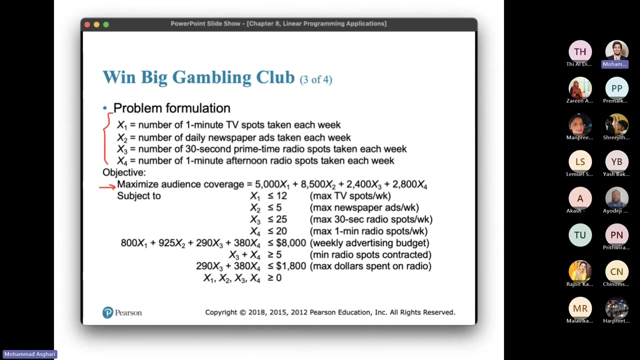 From This Number, The Last Column. So, As Same As For Other Media. So And So. This Is The First Type Of Constraints You Can See. 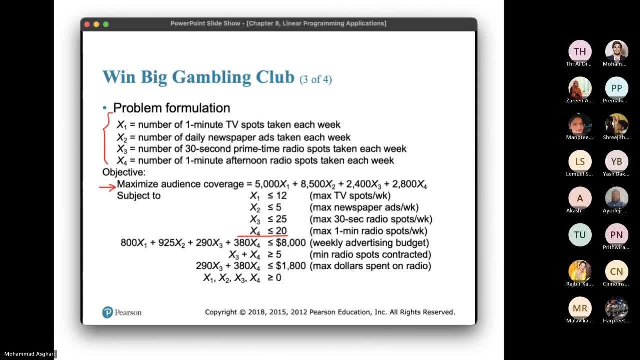 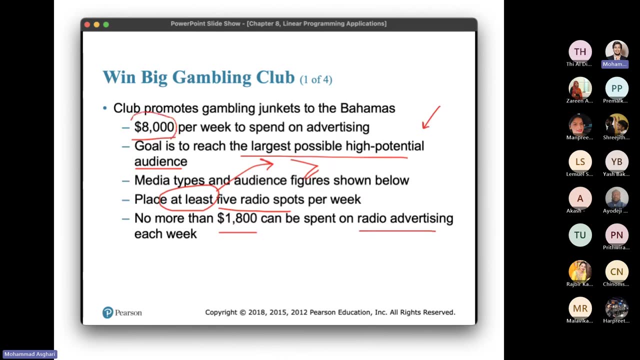 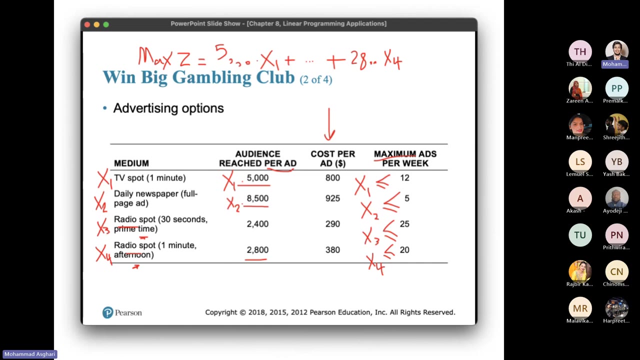 This Is The Objective Function And First Constraints, So Limitation On The Next One We Have. Do You Know That We Have A Budget Of? 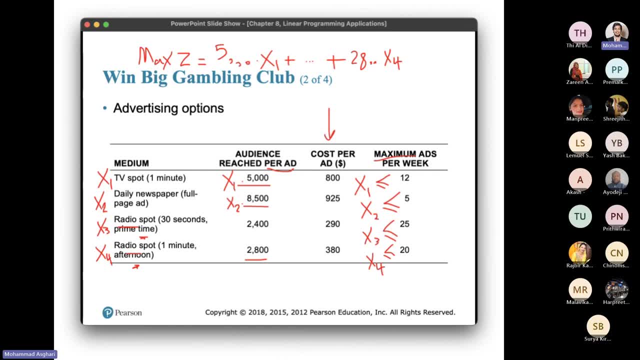 Eight Ten Thousand Per Week. Advertising In Each Medium Cost Us. Each Advertisement Cost Us On TV And Each Advertisement Eight Hundreds The Number Of Advertisements. 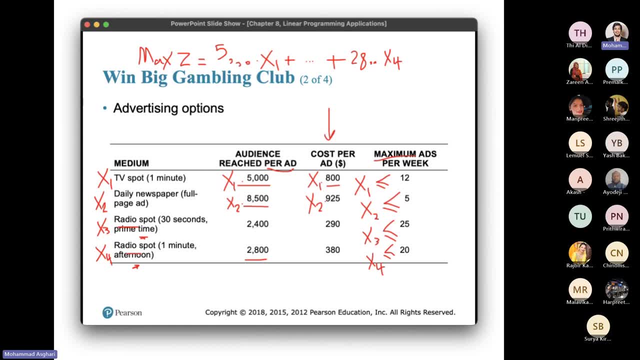 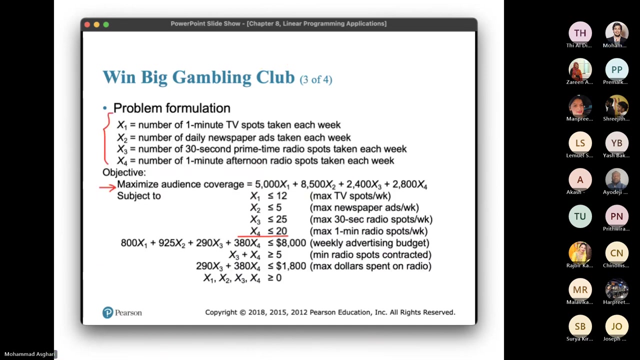 On On Newspaper, As Same For Others. If You Get A Summation Of Them, They Must Be Less Than We Have, So We Cannot Exceed. 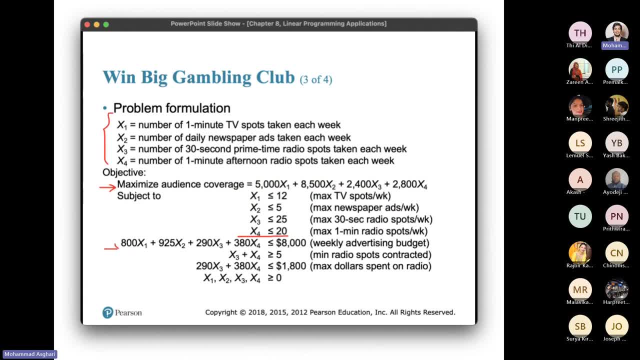 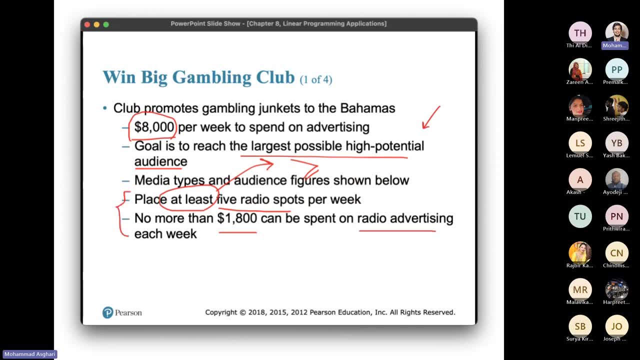 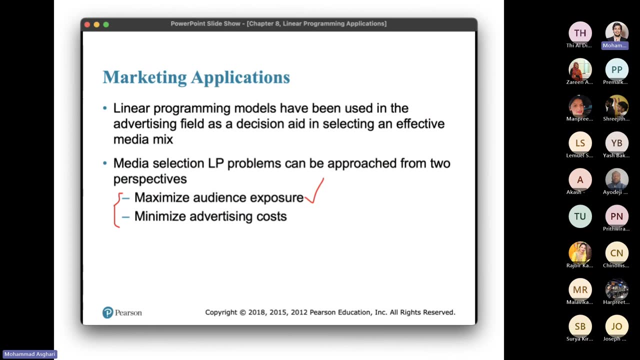 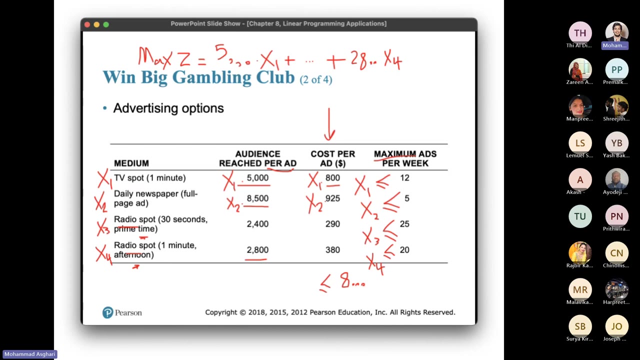 This Number. As You Can See Here, This Is The Maximum Budget We Have, And We Have Two Conditions As Well. As You Know, We Have 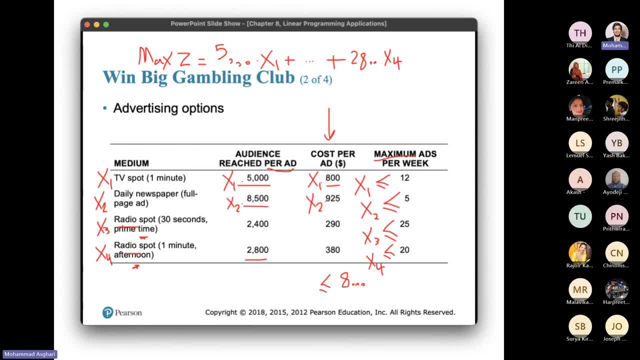 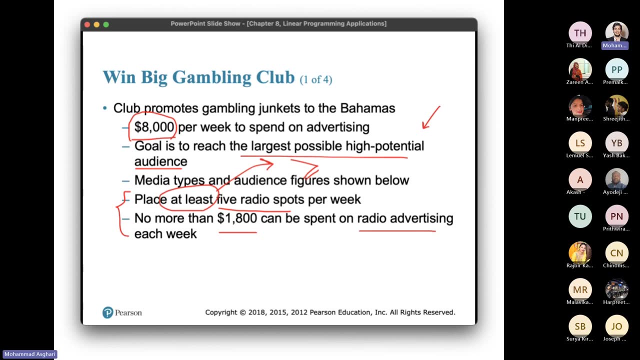 A Lot Of Advertisement Campaigns: The First Campaigns X3. Radio Spot In Prime Time And The Next Campaigns Radio Spot In Afternoon. So 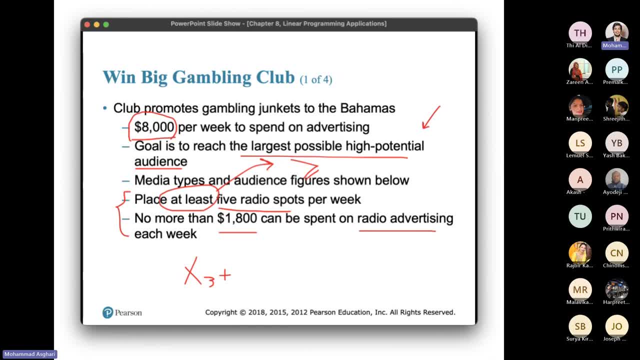 They Must Be At Must Be Greater Than Or Equal To Far. The Number Of Advertisement On Radio Must Be At Least Far, And This Is 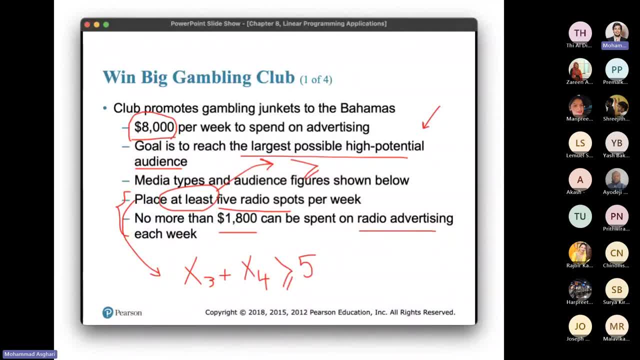 This Condition, So The Next One. No More Than So, We Have To Multiply The Cost To These Variables. These Variables Show Us The Number Of 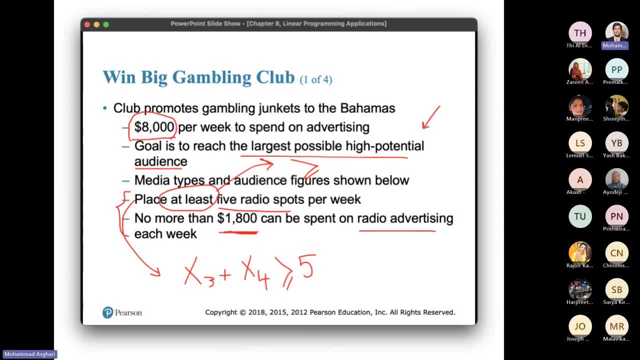 Advertisement: The Number Of Times You Advertise On Each Median. So The Number Of Advertisement Is Less Than Or Equal To Okay, When We Are. 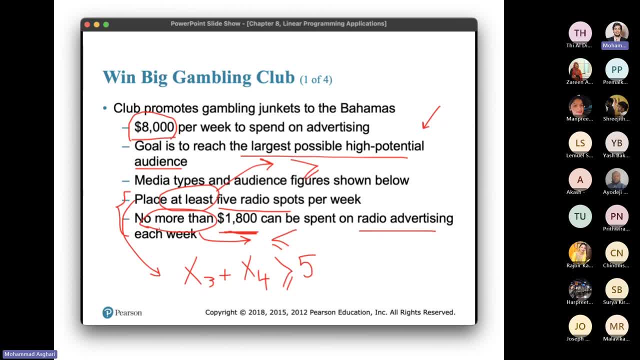 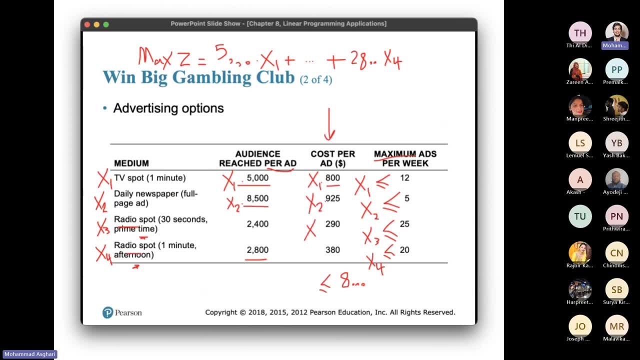 Talking About. At This, You Should Use This Sign. And When We Are Talking About, No, What We Are Talking About. What We Are Talking About. 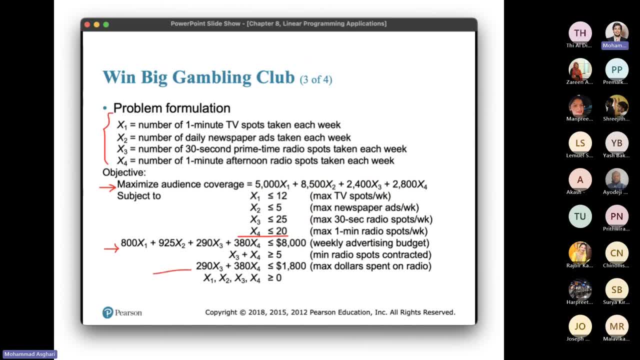 This Is Less Than Or Equal To Eight One Thousand Eight Hundred. As You Can See The Cost Of This And After Writing All Constraints, You 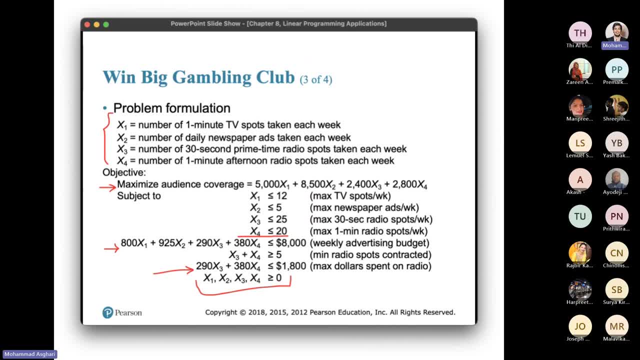 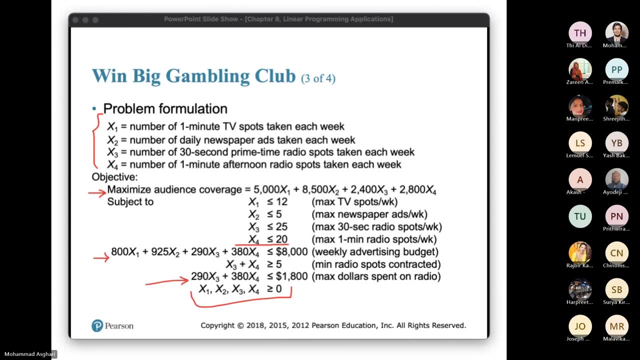 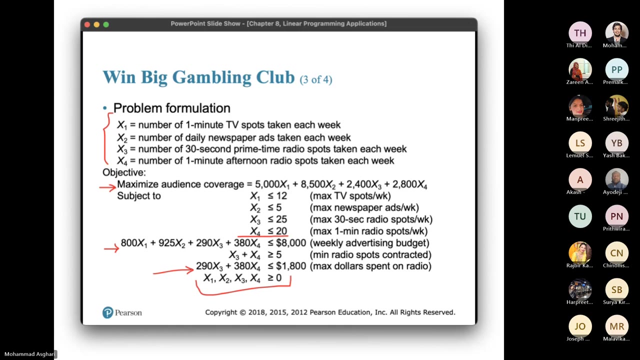 Have To Add This One, Non Negativity Constraints- At The End Of The Model. So This Is The Model. Any Questions? So Far Nothing, I said. 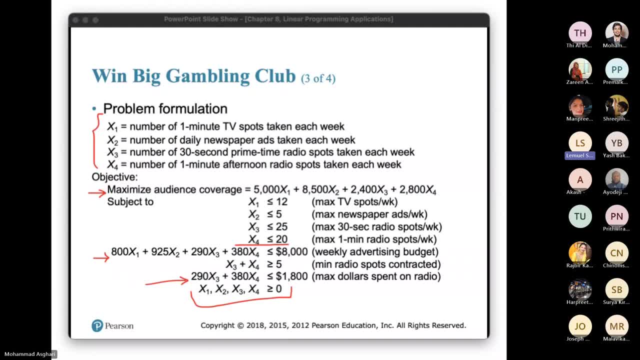 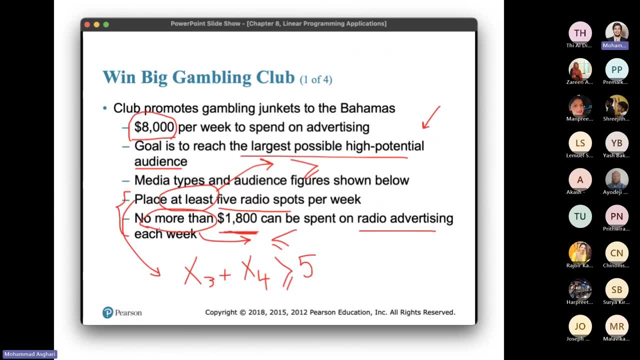 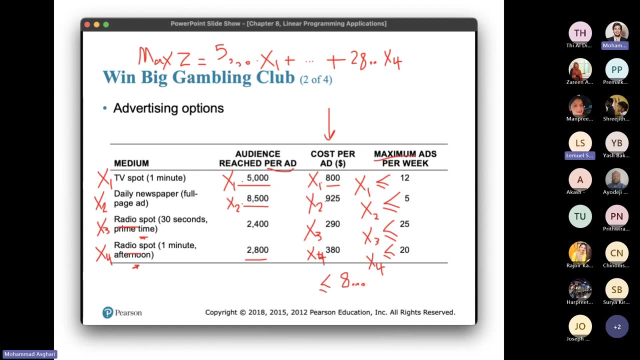 Hey, God, Yes, Is It Necessary That We Have To Have Use All Types Of Mediums Of Advertisement In This Problem? So We Have Some. 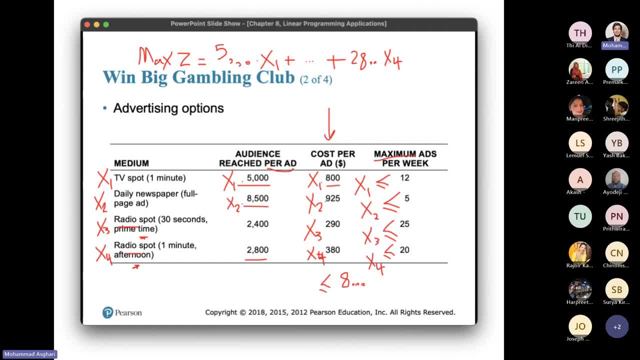 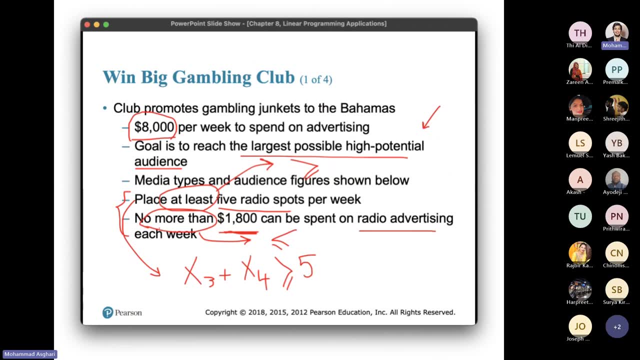 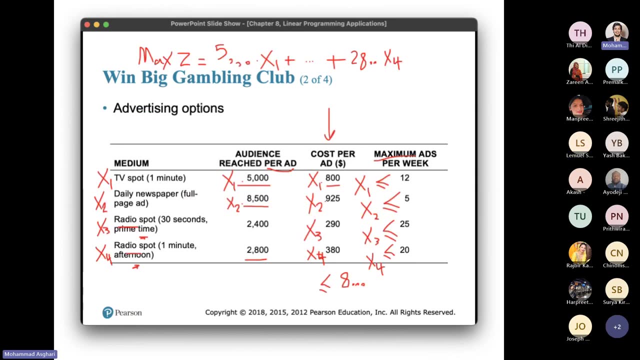 You Have A Budget And We Are Trying. This Is The Goal: Maximize The Number Of Audience. And You Don't Have Any Idea At This. 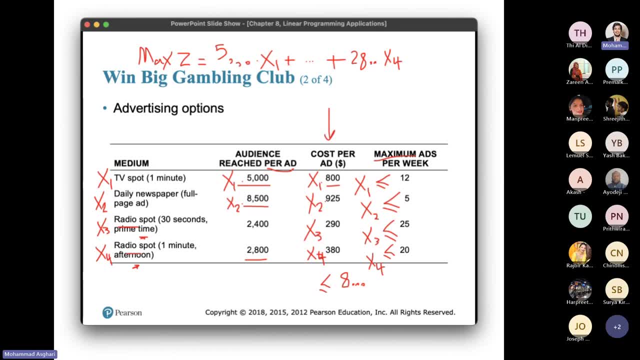 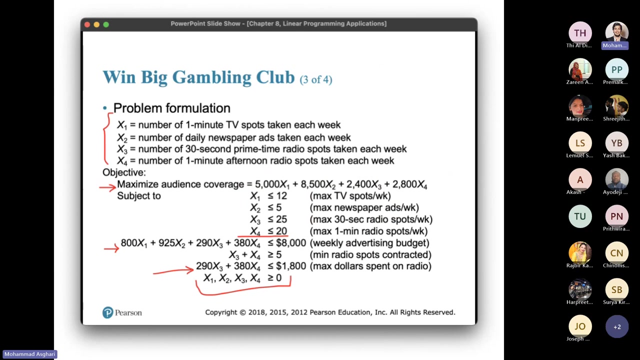 Moment Before You Saw The Model. You Can Pay For Each One. You Cannot Put All Of Your Money On TV Or Newspaper Or Radio Spot. 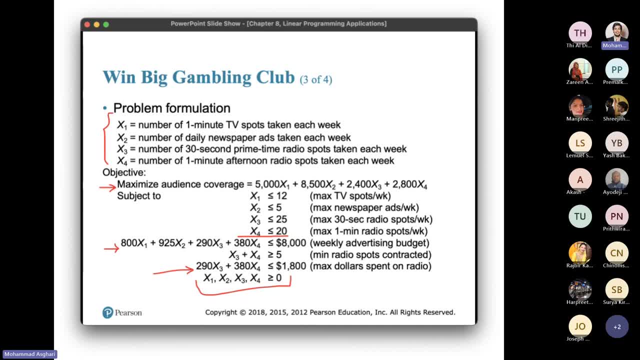 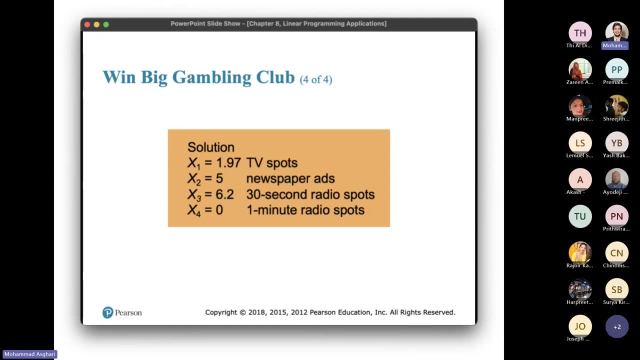 So You Should Consider All Of These Constraints And The Model You Can Solve, The Model You Can Reach To These Numbers Is: One Did The. 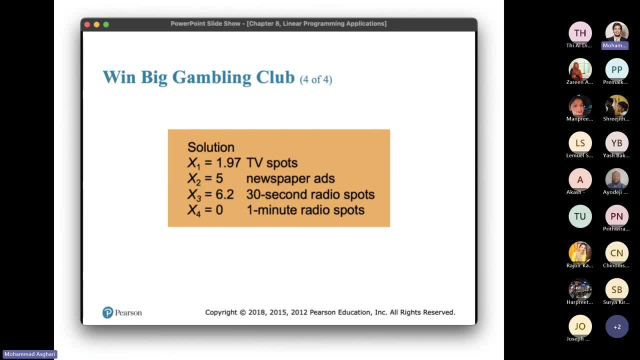 Number Of Times You Should Advertise On TV One. Point 97. Is Too Hard To Solve The Problem. This Is Linear Program Models And, As 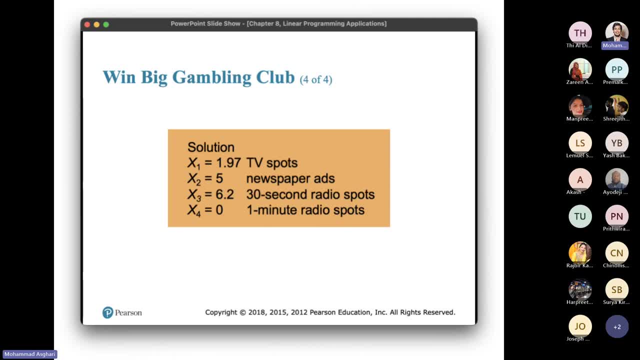 You Can See, We Have More Than Two Decision Variables, So Cannot Use Graphical Or Corner Points. After Solving The Model, You Reach This Number. 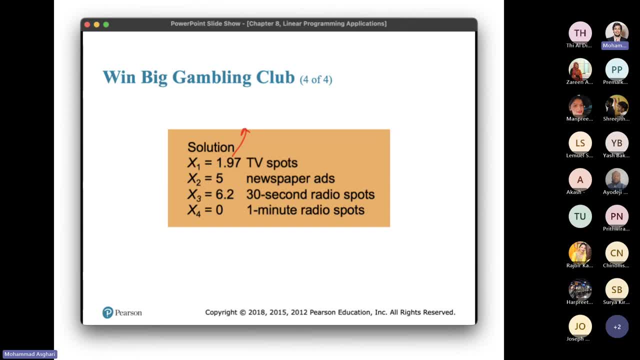 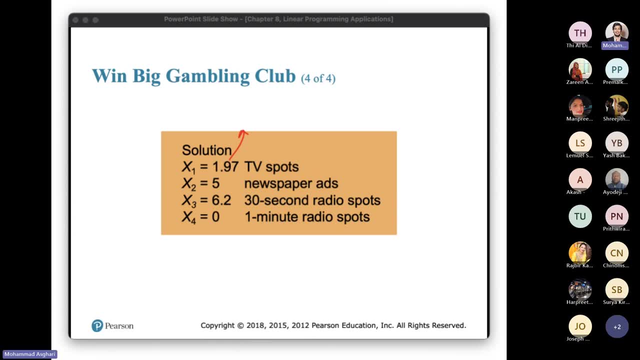 But What That Means When You Have So In Next Session We Use A Different Type Of Models, So So That Is A Variable. So In 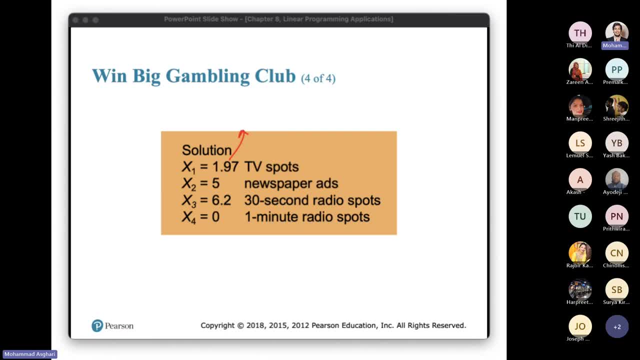 Real World. We Don't Use A Variable. That Can Be, You Know, Get A Real Number. Or Right Here You Can See One Point One. 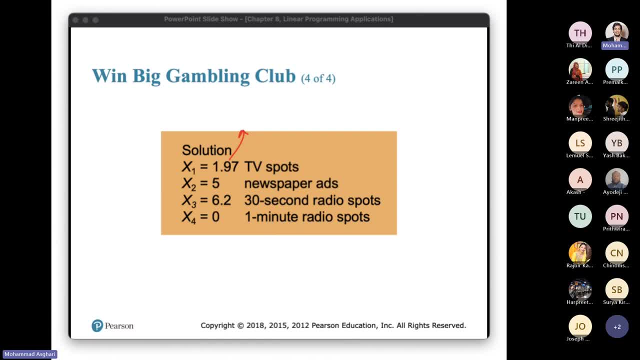 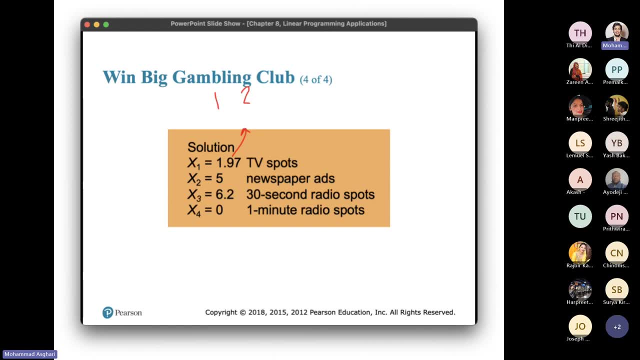 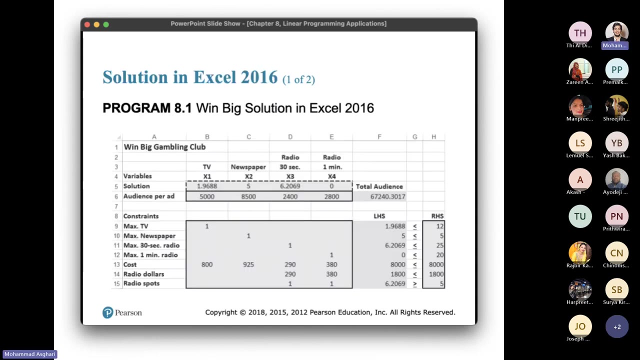 Notice Heads Up. Okay, In Integer Programming We Can Just Use For Example This Number One. This Variable Can Be One, Two, Three Or Any Number. 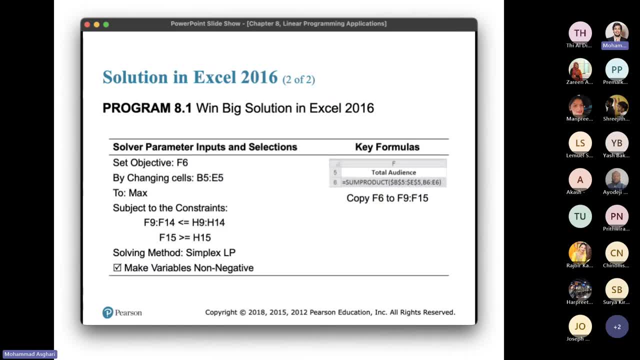 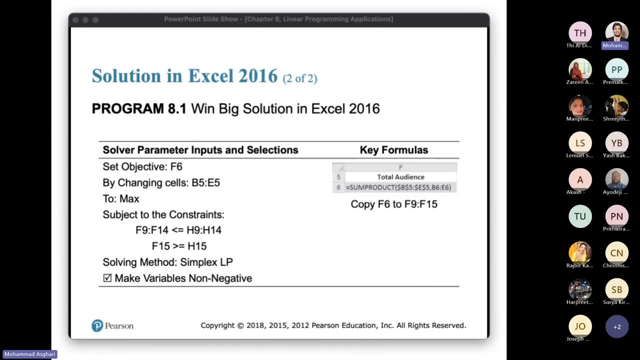 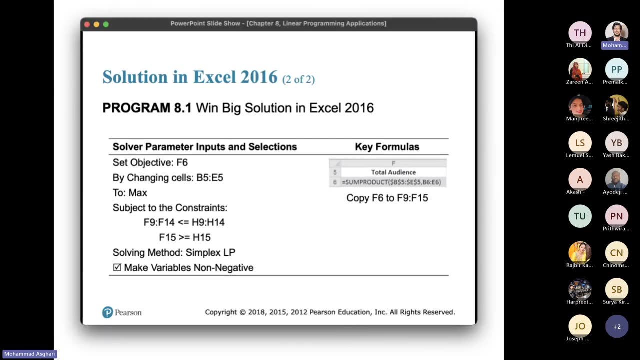 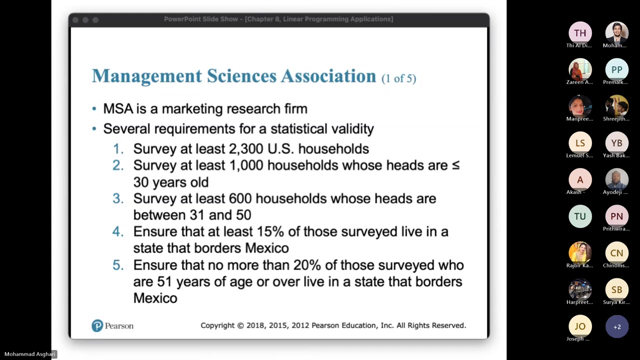 It Can Not To Solve The Problem. This Is Not Or A Scope, And We Are Not Going To Spend So Much Time At This. So 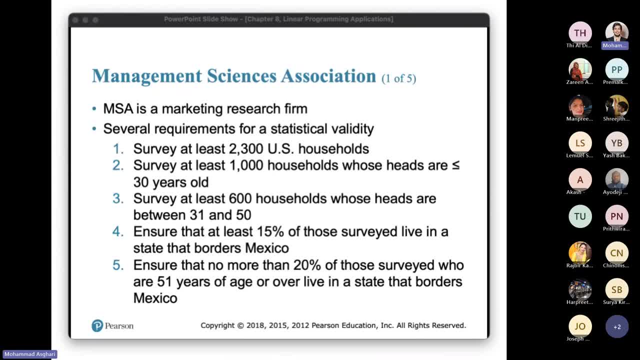 We Want To Solve Another Marketing Problem. So It Is A Marketing Research Firm. Several Requirements For A Statistical Validity. Okay, So It Says Requirements. 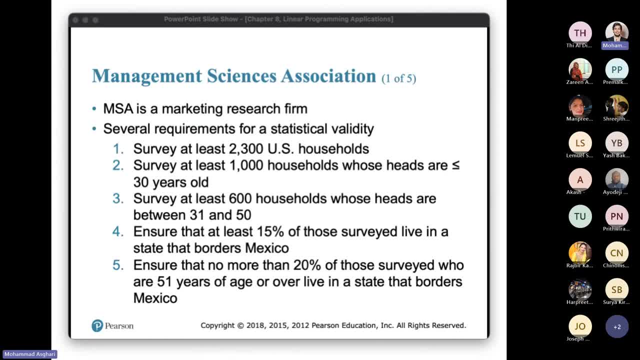 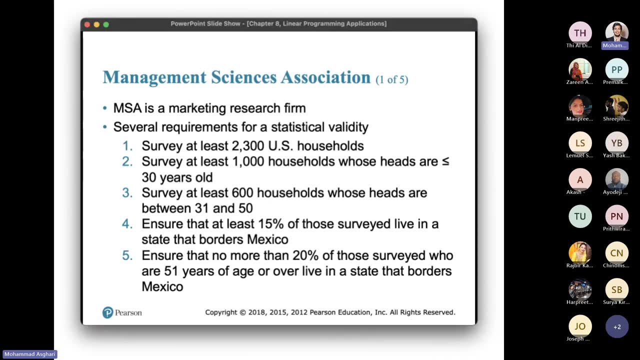 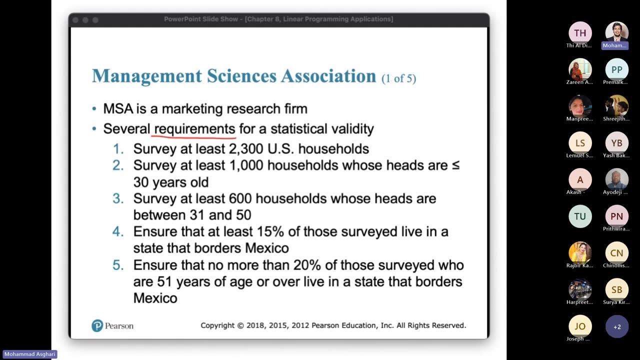 Conditions- Minimum, Maximum, So These Are All Rated To Objective Functions. So Constraints Are A Kinds Of Constraints. So When We Are Talking About Requirements, 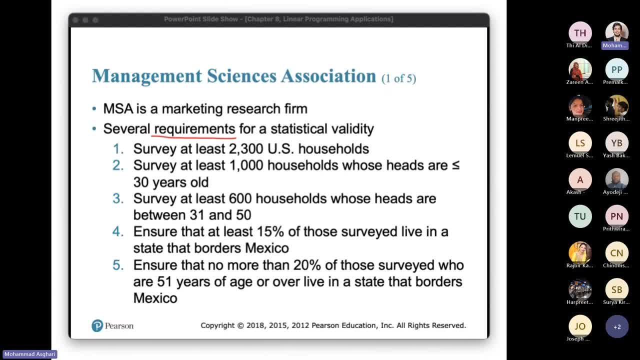 So Let Me Read This And The Comments. It Is All Something That Limits Us Either From The Entire Community Or From The Entire Community. So 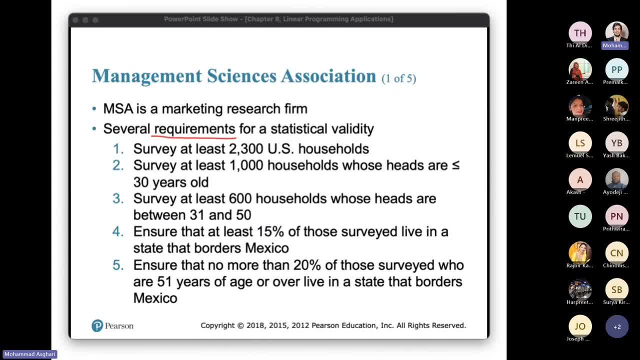 They Need This Company, This Marketing Research Company. They Are Dealing With People And Survey And Asking People About Their Opinion, To Do Some Surveys. 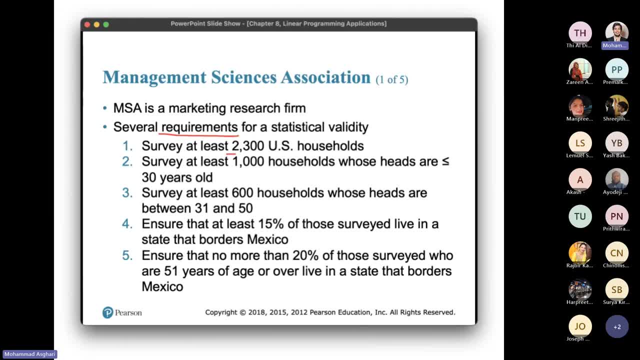 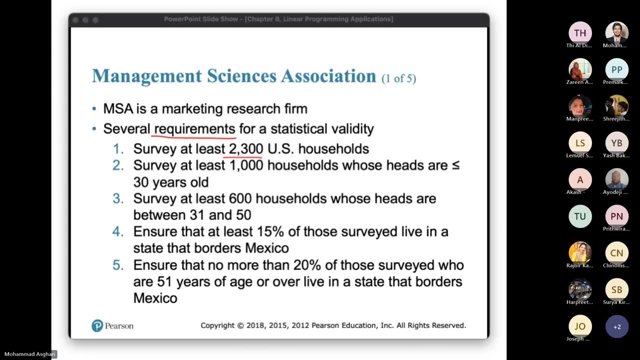 And In Their Surveys They Need To At Least Contact 2,300.. United States Households, People And The, So That's One Of The Constraints. 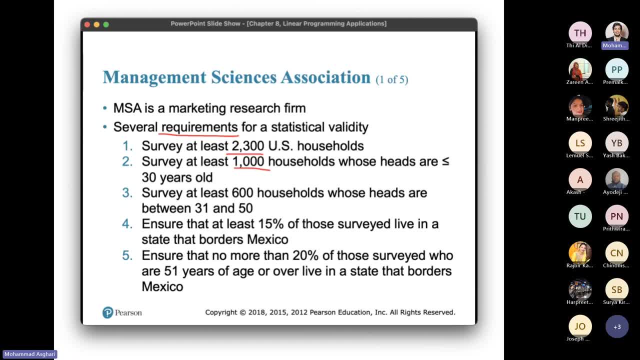 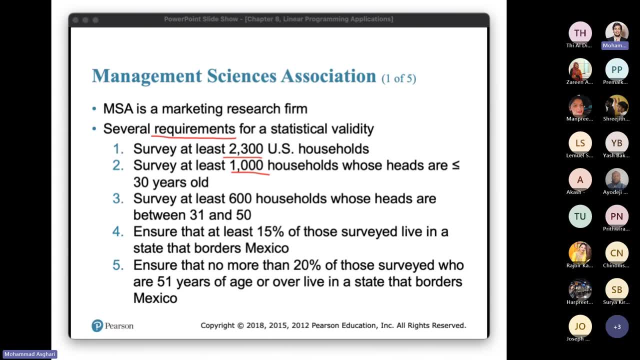 The Next One Less Than 30. Years Old. So It Looks That They Are Contacting People And Surveying People From Different Ranges Of Age. 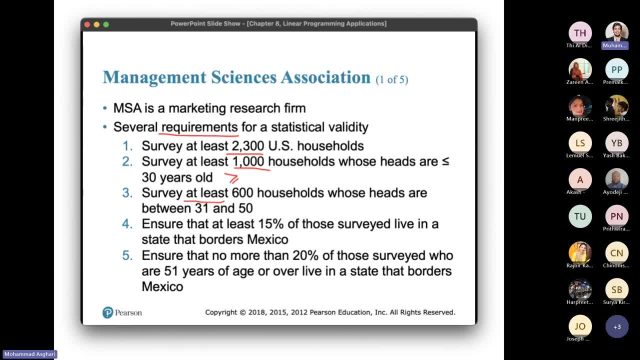 And Then At Least, When We Are Talking About The Households Whose Heads Are Between 31. Years Old And 15. Years Old. So There, 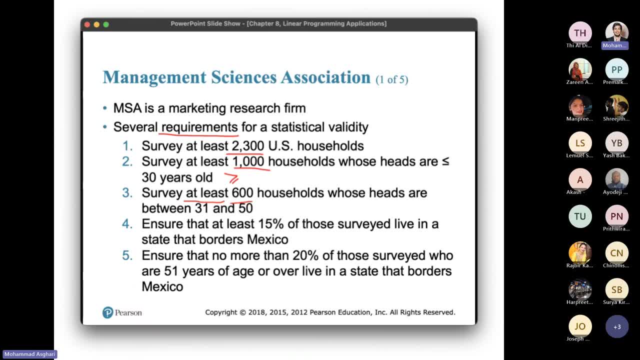 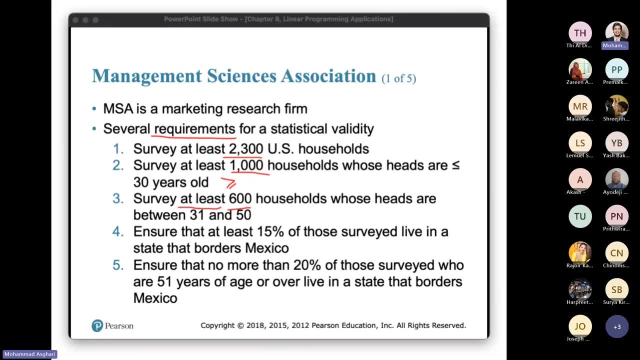 Are Two Different Types Of Counseling, And Number Four And Four Ensure That No More Than 20. Percent Of Those Who Are Surveying, Or 15.. 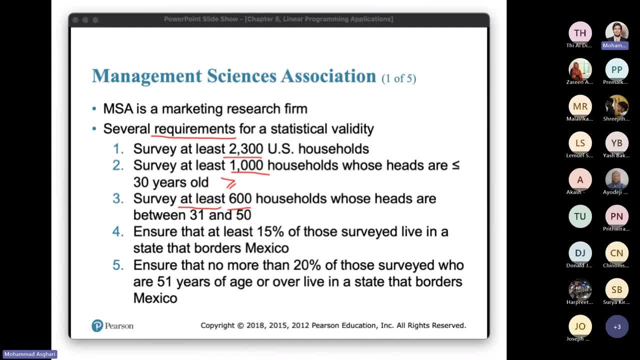 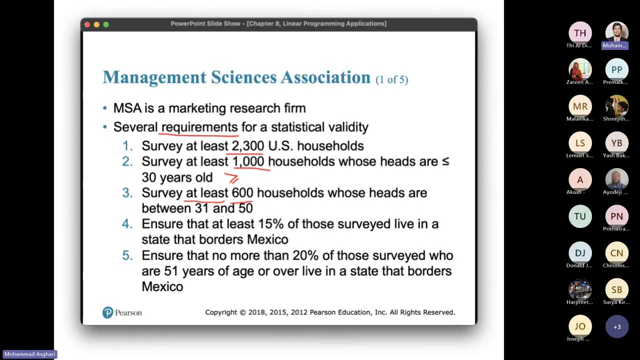 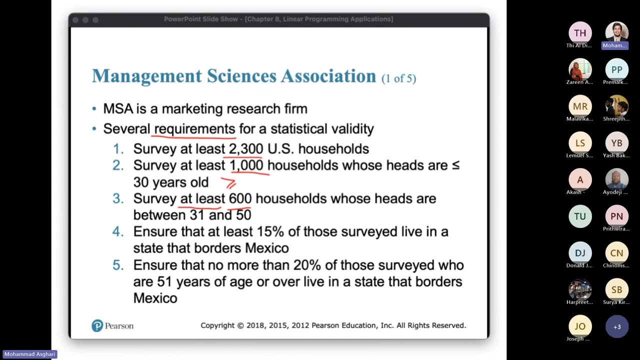 Years Old And Or More, And The Next One, Number Four, Ensure That No More Than 20. Years Old And Also They Are Living In. 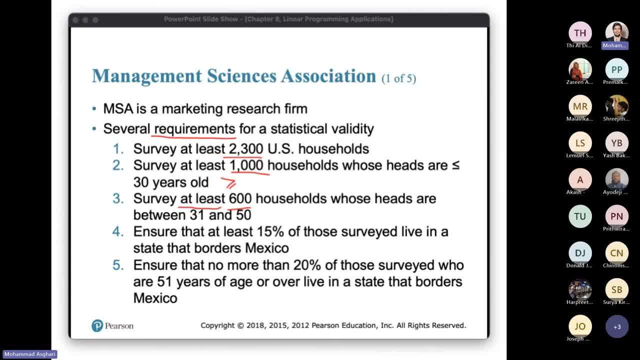 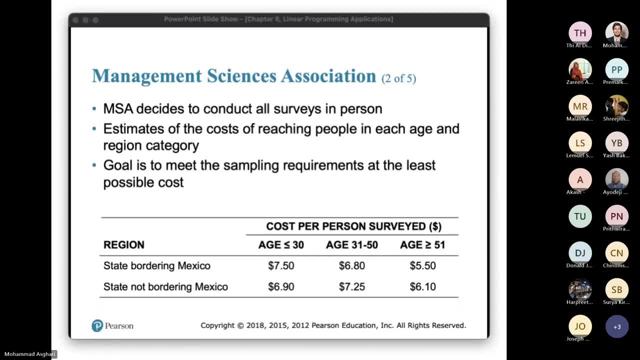 The State Close To Mexico Border. So We Came Back Again To This Constraint And Formulate One By One: Okay, So Initially, So As We 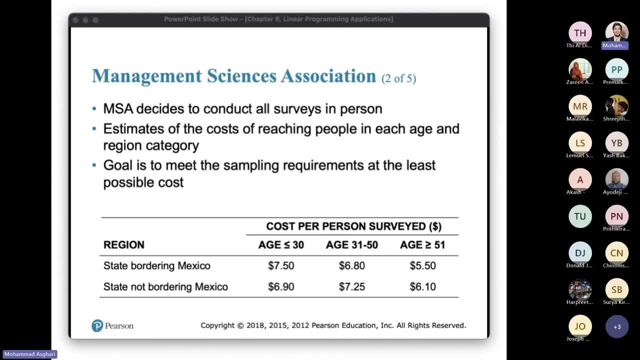 Can See, We Have Different States And They Are Divided Into Different Types Of Estate. It Says A Border In Mexico, So These Are States. 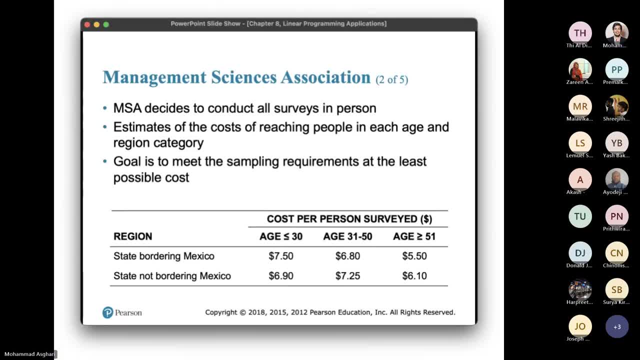 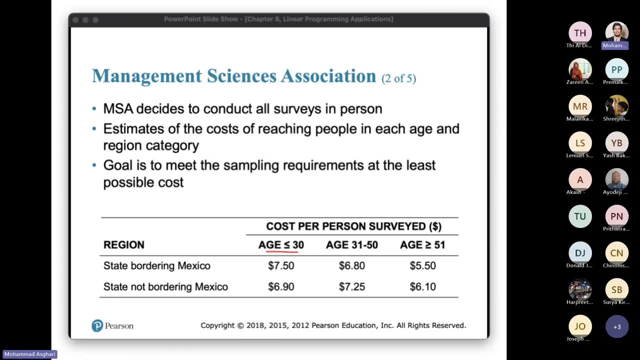 Close To Mexico And The State Of Mexico, So A Family That They Had. They- Their Head- Is Less Than 30. Years Old, If Family. 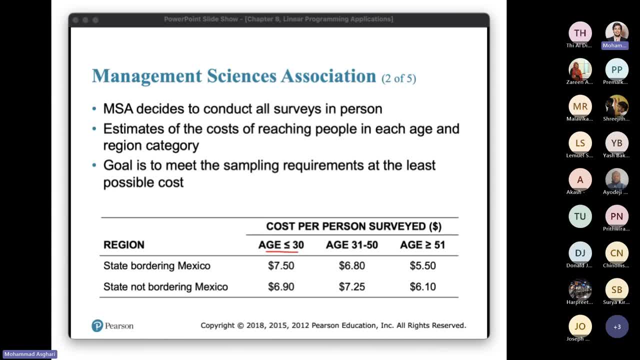 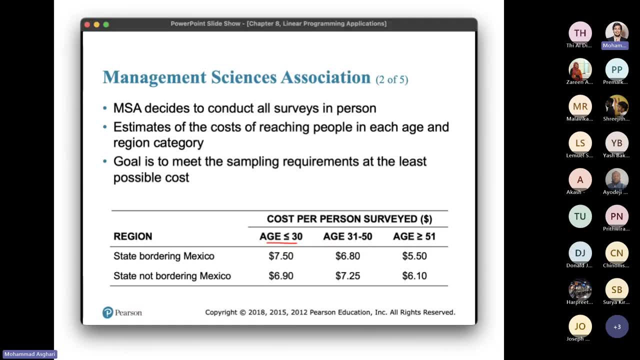 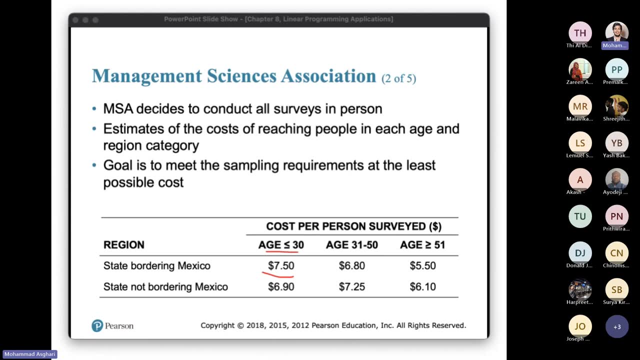 That Their Heads Is Between 31. And 30. Years Old, So How Much We Should Pay For That Survey It Cost Cost Us Seven Points. 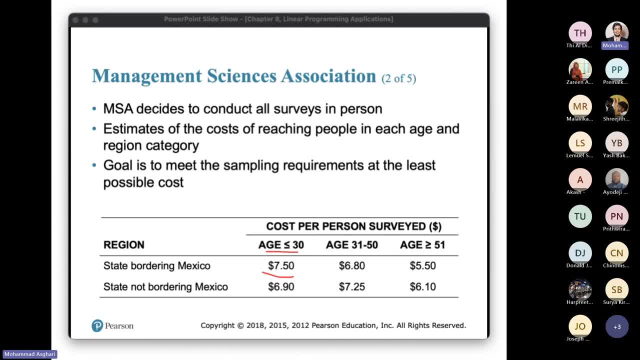 Five Dollars, Okay, And Look At That Survey It Cost Us. And Look At In This Case This Represents A Survey That The Cost Of Solving That A Family, A Head, Is More Than 15., 51. Years Old And They Can Consider This Cost As Incentive. You Have To Pay. 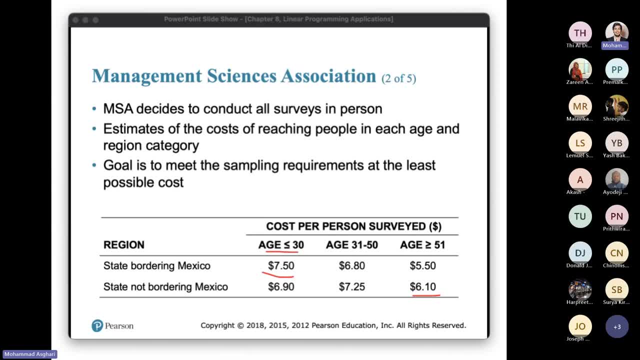 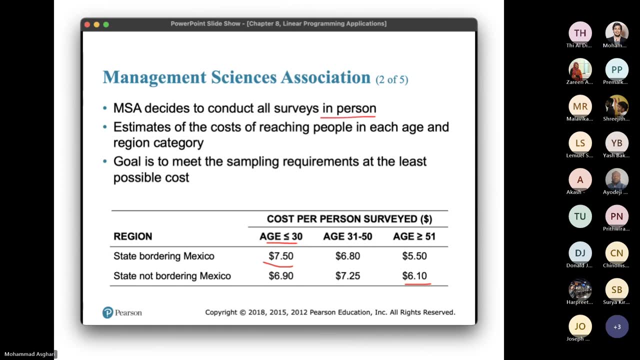 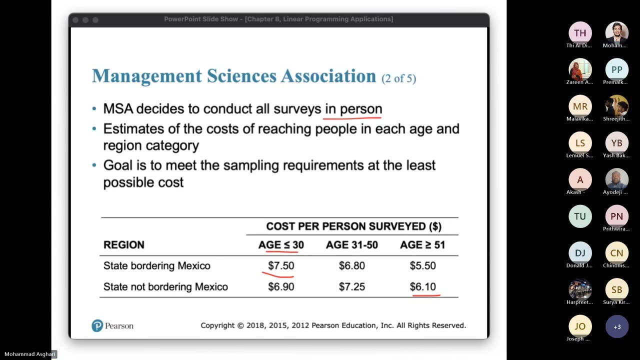 To This Type Of People. So This Is All About The Cost. So What Manager Wants These Manager Wants To Meet The Cost Of Reaching. 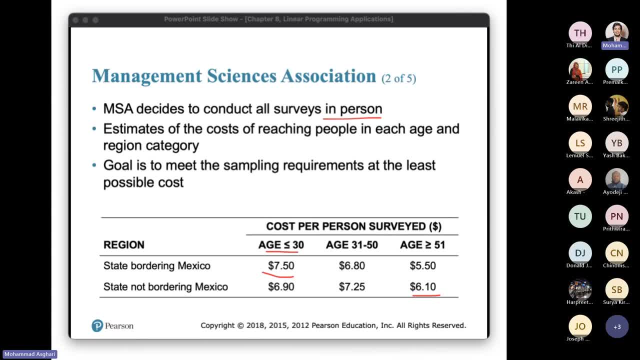 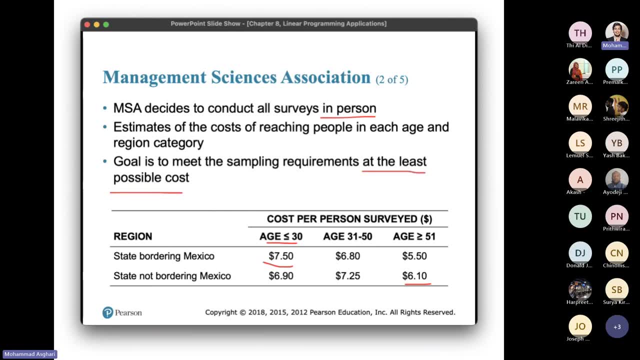 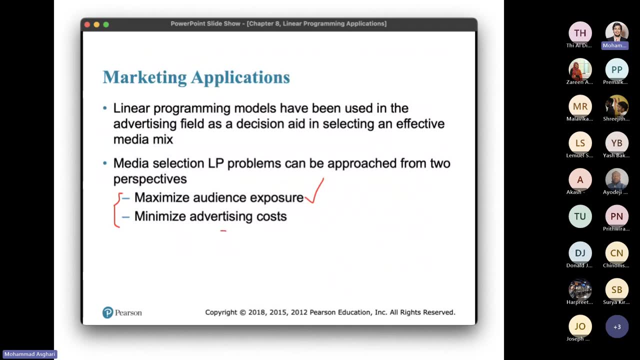 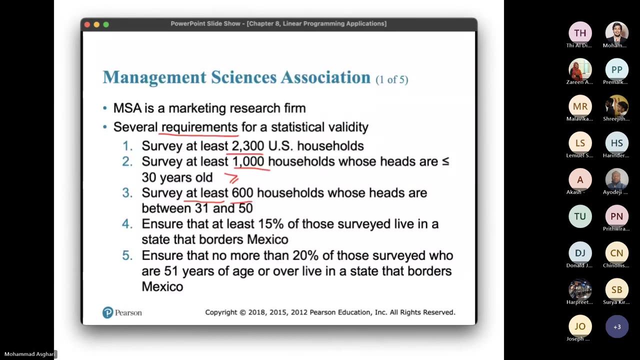 People In Each Age And Region. Goal Is To Meet The Sampling Requirements At Least Possible Cost, At Least Possible Cost When We Meet People. So 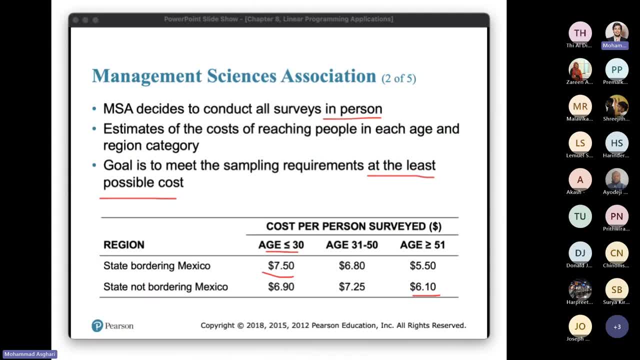 We Know That. What Is The Objective Function? We Should Minimize Our Cost. So What Is The Next Step? We Understand The Problem. We Know. 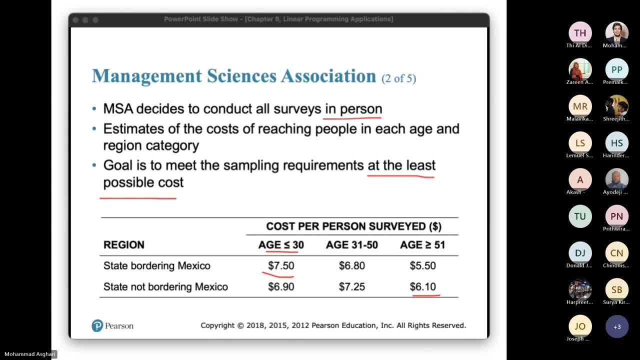 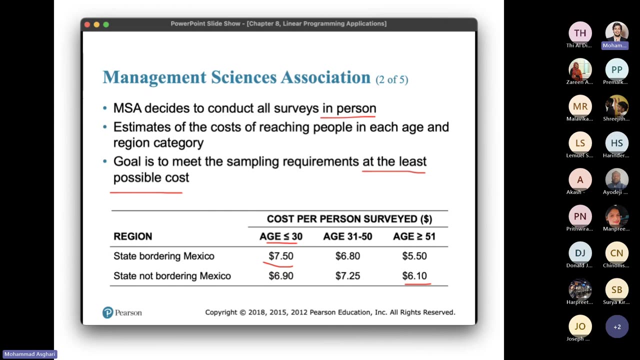 That We Have A Decision Writers. We Need To Define How Many Number Of Decision Writers. We Need To Define How Many Number Of Decision Writers. 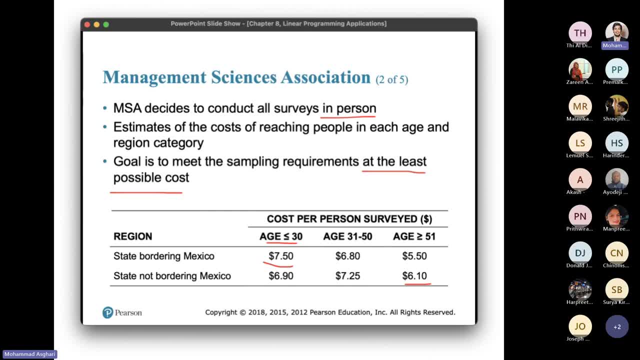 We Need To Define How Decision Writers. It Is Better To Define Decision Number Six, Decision Number X1. To X6.. Okay, So I Can Assign. 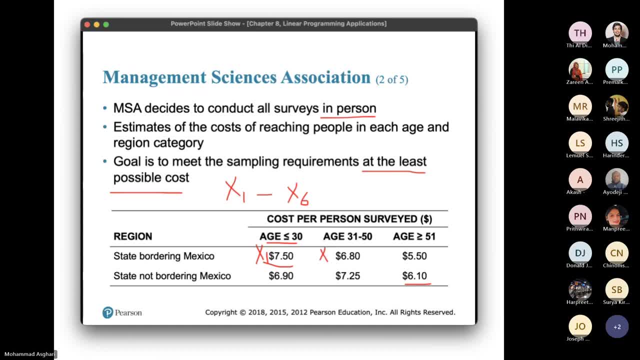 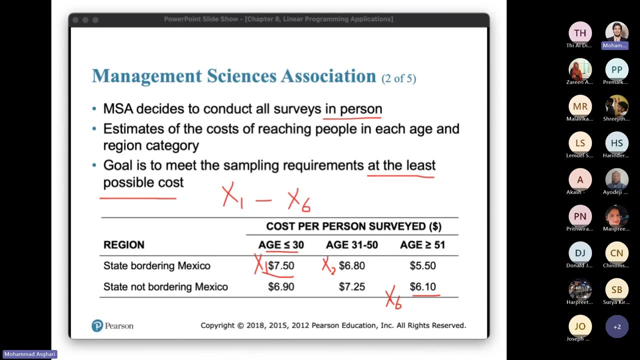 X1. To This And X2. To This One. X6. x to this one, so uh and uh. so. x1 represents the number of people that we need to survey from a family. uh, less than 30 years old and they live in a state border- border in mexico. and x2. 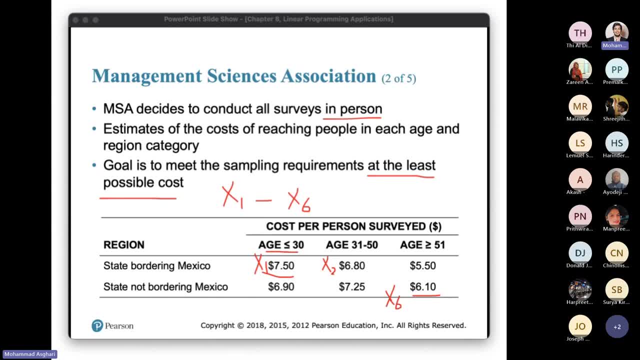 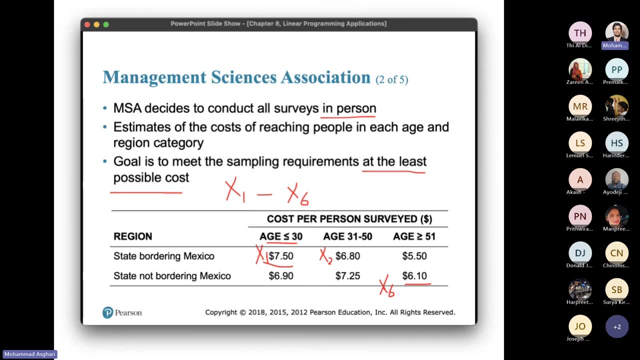 is the number of people um, their head is between uh and 30 years old and 15, and uh, they're living close to mexico border and x6 is the number of people we need to survey, in that they they are more than 15, uh, they have more than 51 years old and they are not living. 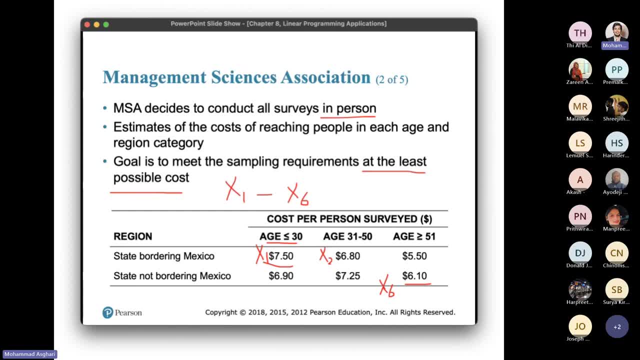 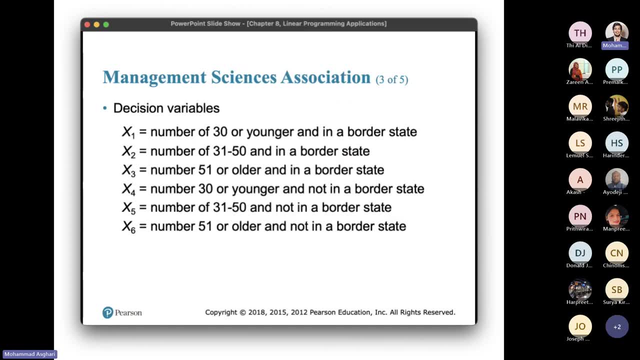 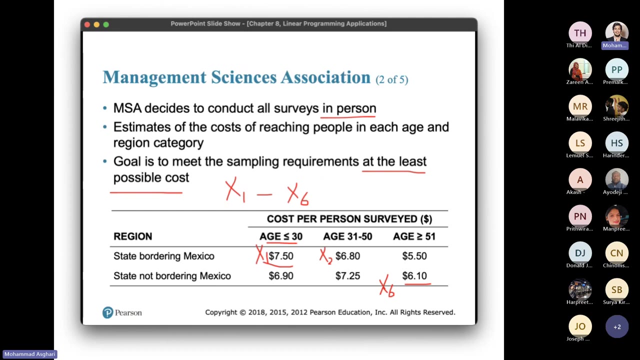 close to mexico border. okay, so if you define six decision variable, you can write the model much easier. okay, so you can see all decision variables in this slide, and so now we are able to write objective function. so what is the objective function? we should, uh, meet outcome. 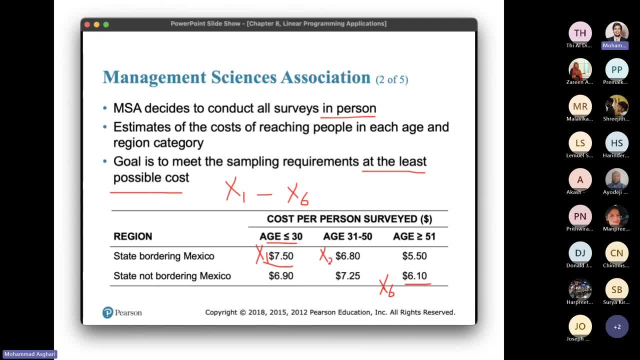 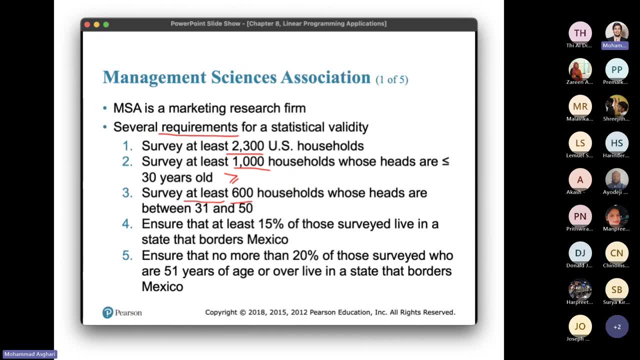 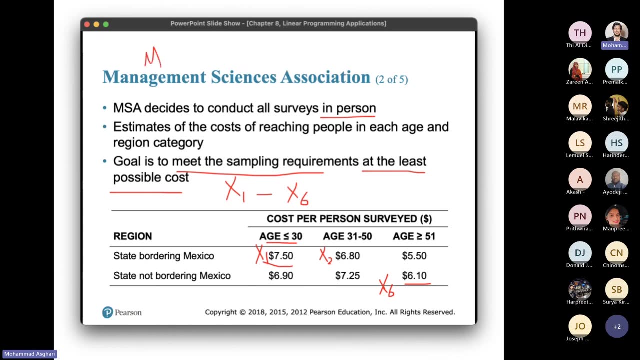 we should meet all requirements, we should consider all constraints with at least possible cost. we know that what is the constraint and we can write objective function here. let me write objective function here: uh, minimization of zip equal to what is the cost of uh each uh people. 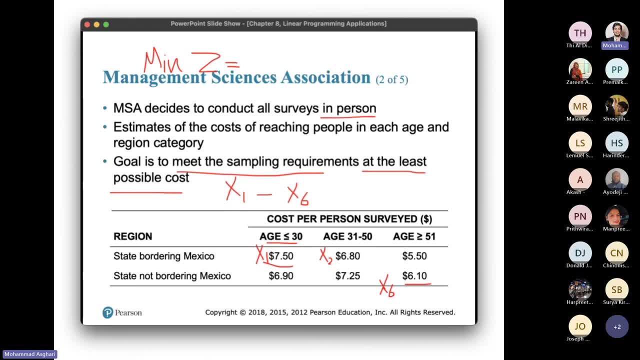 you saw way in this age, less than 30 years old and close to mexico, cost us 7.5, and x1 shows us the number of people in this category. you should multiply the cost of each people in this category to the number of people small. 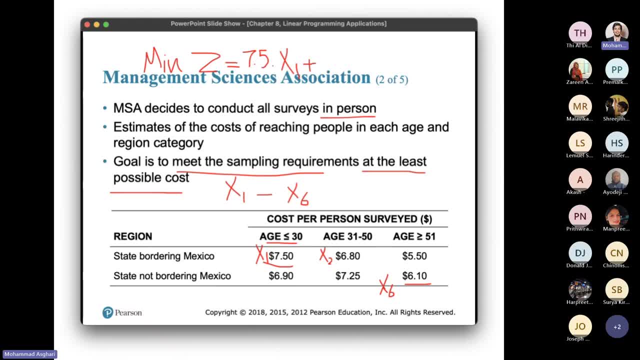 plus define the decision variable step, including the suitable model. so what are you going to need to draw here? you simply have a slicer solution. i'll give you theestic year testing, so this doesn't require students, but i also want students to draw Yayy. 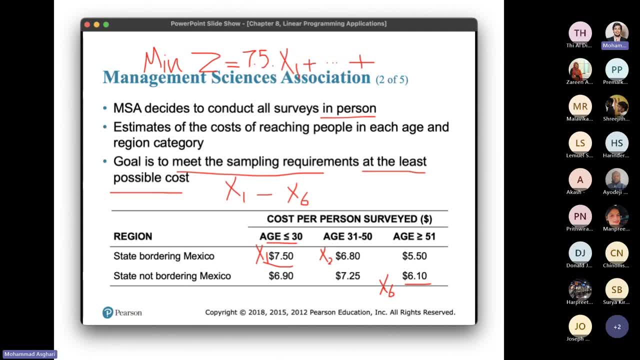 Hopefully you enjoy what you裰 and see that this uh is a very useful and powerful way for алion TO whether you give or reject grading. oh, list of analysis: how do we organize? lets see what parts of that structure of the okay to have and what points support thatu. 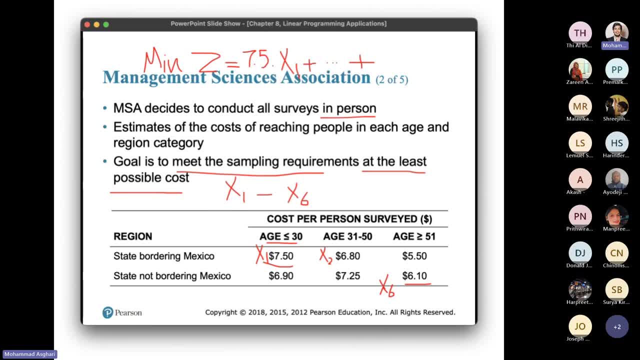 traveling in different parts and reach different optimal solutions. And the last one: the cost of people, their age is more than 51 years old and living in the Kelo-2 Mexico border, and to multiply the number of people in this category. 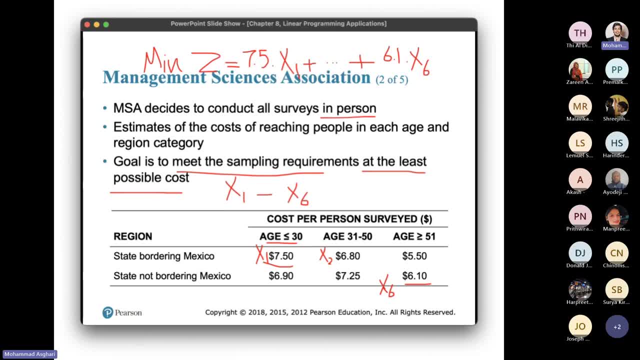 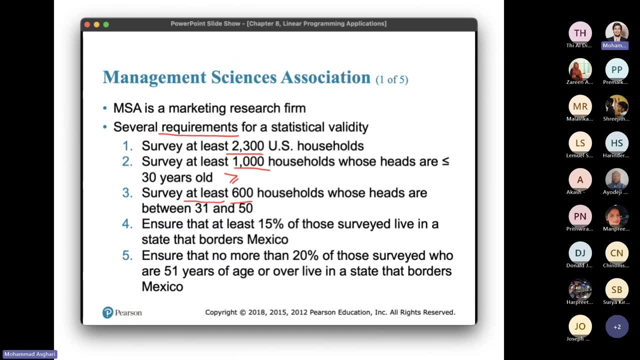 So in this way you write the objective function. This objective function tries to minimize the cost of survey, but at the same time you should meet all constraints. What are the constraints? Let's see and write them one by one. The first one survey at least 2,200 US households, so we should survey at least this number of. 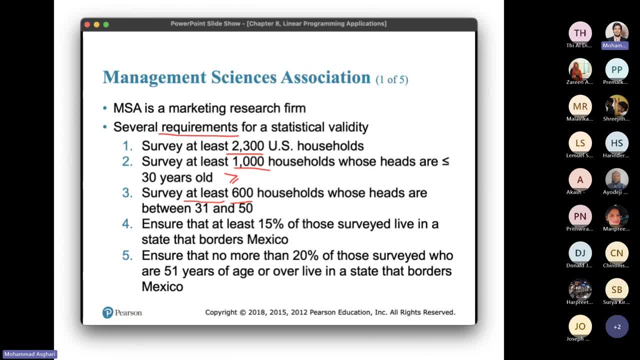 people. How we can write the number of people we surveyed. how we can write them: X1 plus X2 plus X3. Plus X3 plus X4, plus X5 plus X6. If you get a summation of all of them, this equation shows us the number of people in. 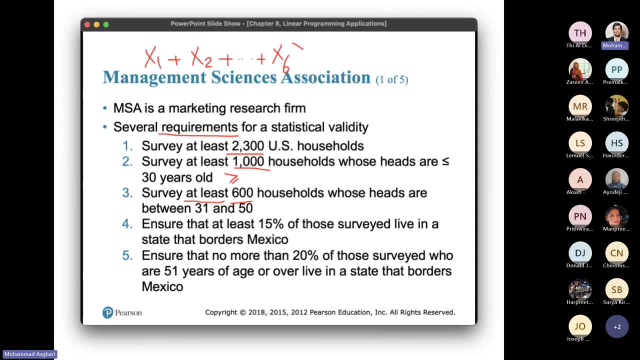 the survey. That must be at least that when we are talking about as this, we should use this sum greater than or equal to 2,000.. Okay, So the number of people, the survey must be at least this number. If you have any question, please break me and ask your question. 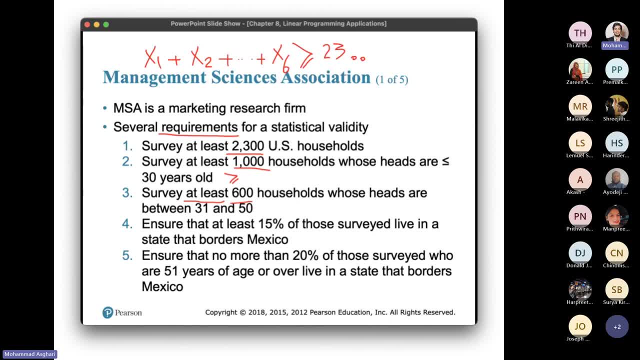 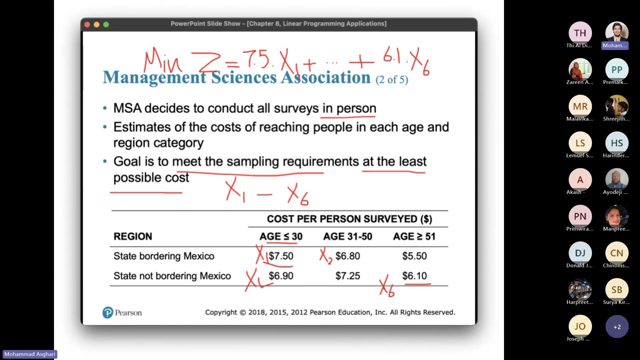 The second constraint survey, at least 1,000 households whose heads are 30 years old. So the people whose heads are 30 years old, less than 30 years old. X1 and X4 shows us the number of people whose heads are less than 30 years old. 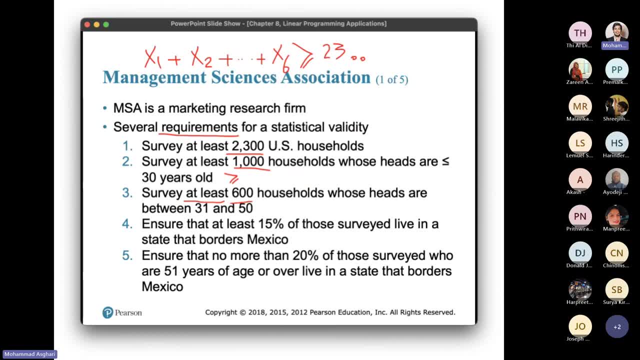 So this constant says us the- let me write it here: If you get a summation, Okay, If you get a summation of X1 and X4, they must be more than or equal to 1,000. Okay, So the next one. so we are at least 600 households whose heads are 30 years old. Okay. Okay So the second constraint survey: at least 1,000 households whose heads are between 31 and 50 years old. Okay, So the second constraint survey: at least 1,000 households whose heads are between 30 and 50 years old. 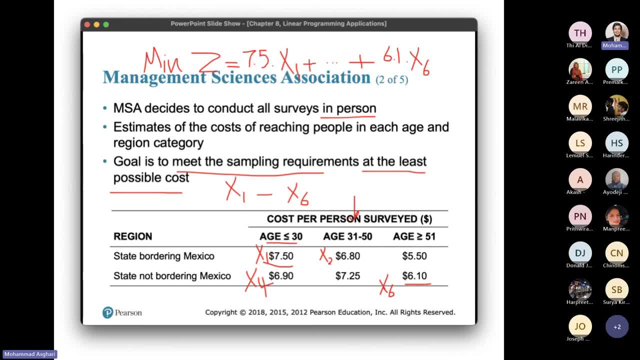 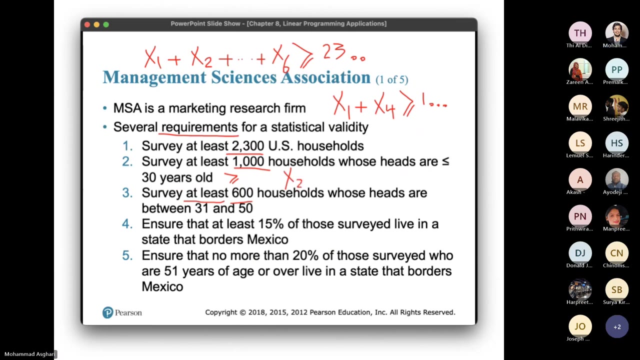 So these people- we are talking about these people in this category, X2 and X4, show us the number of people whose heads are between 31 and 50.. Okay, So X2 plus X5 must be greater than or more than or equal to 600. 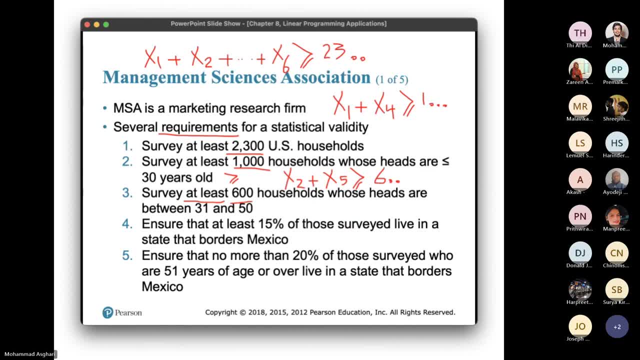 Ensure that at least 50% of those surveyed when we are talking, those surveyed. how many people surveyed this number? This is the number of people surveyed in this problem. We don't have. We don't have any idea right now. After solving the model, we can reach how many people you surveyed. 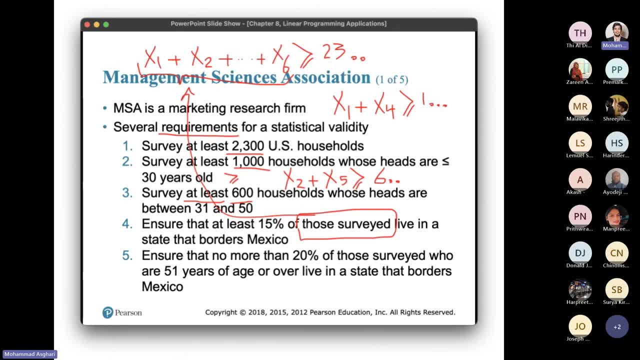 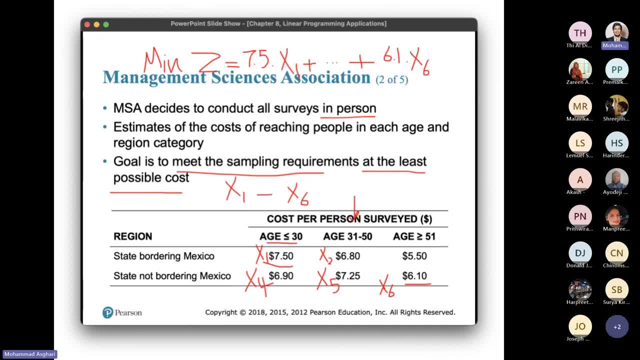 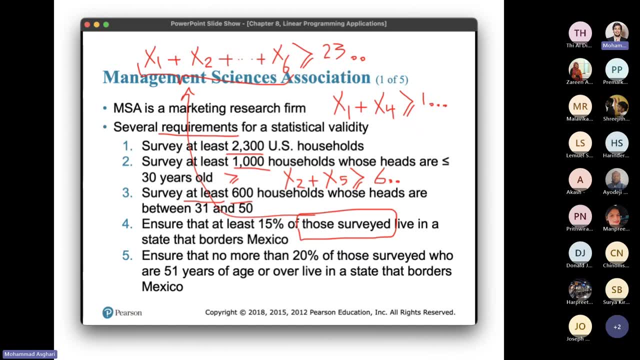 So which variables indicates states of the people? Yeah, So the one that, Which one that Leads the people to living in Leads the people to living close to Mexico in these states. So X1 to X3, these constructs. 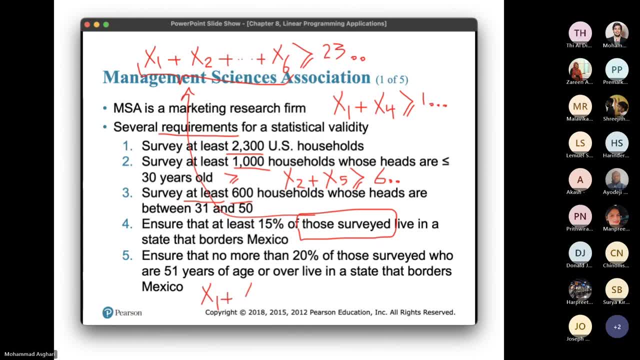 astronaut before here: X1 plus X2, greater than equal to 50%: 0.15 x1, x plus x2 plus x3 plus x4 plus x5 plus x6. all of them who solve it? this is constraint number 4. 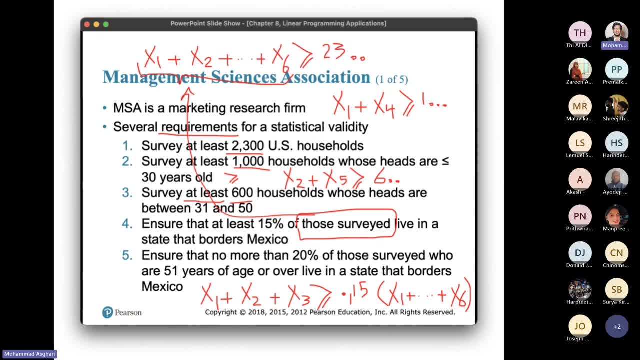 the number of people live close to Mexico border x1 to x3 must be at least or greater than 50% of those solve it. people solve it x1 to x6 and the last constraint ensure that no more than 20% of those who are 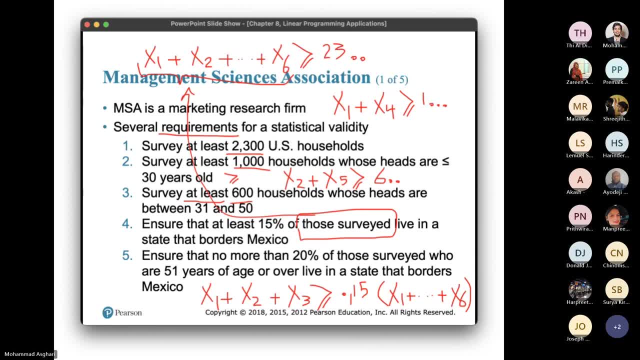 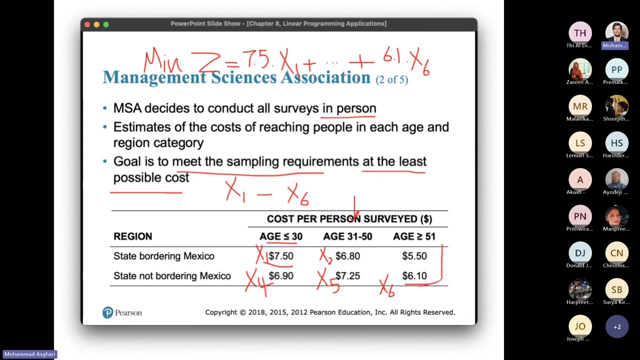 50 years of age or live in a state that borders Mexico, when we are talking about no more than we should use this sign so that borders on. this constant says that the people in this age- 15 years old- in this category is 5, is 2 and. 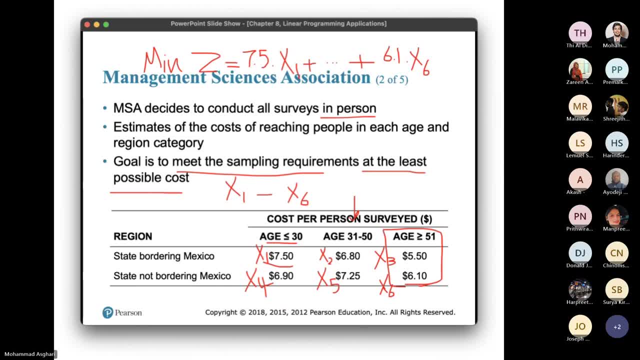 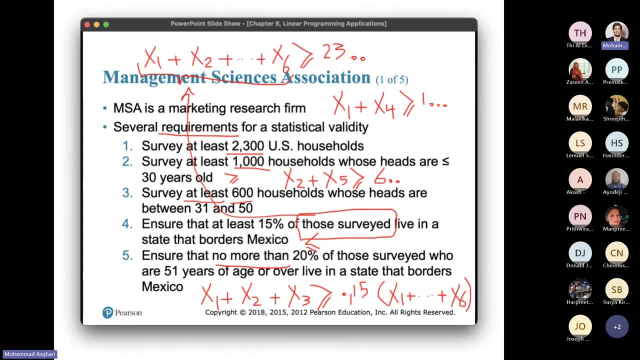 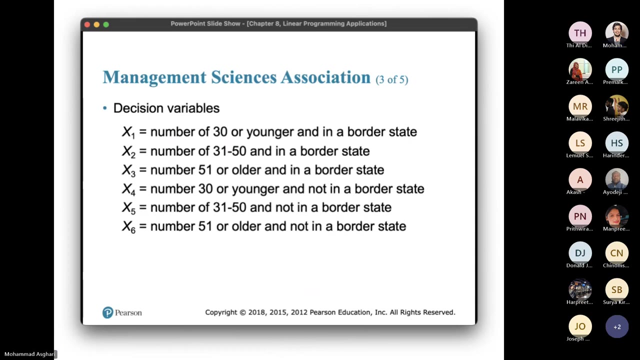 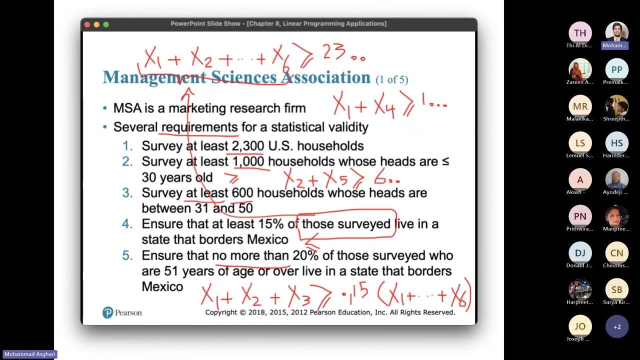 is 6, must be must be greater than or equal to 20%. let me check to make sure that, yeah, the people who um um, um, who their age- their heads are more than 50 to 100 years old- must be and they are living close to. 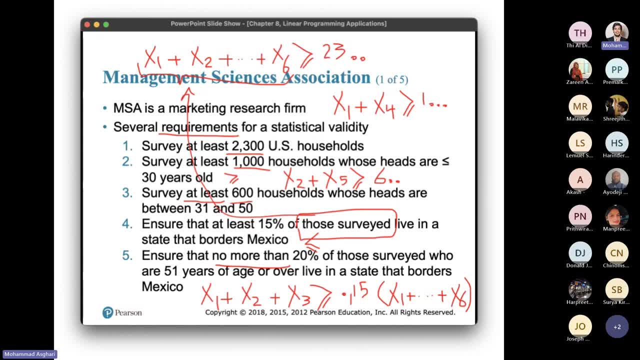 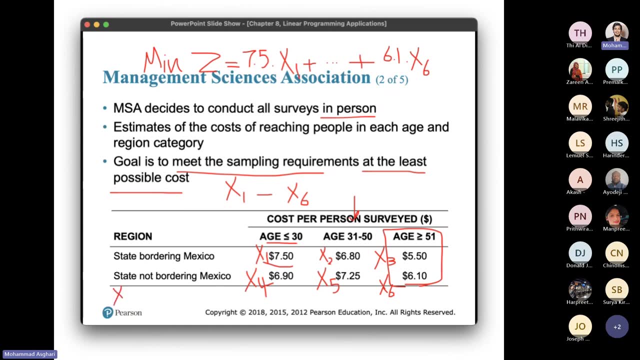 Mexico border must be less than or equal to 20% and have this age. they are more than 50- 51 years old. if we write this constraint here, x3 the number of people they are living uh close to Mexico and have this age we are talking about. 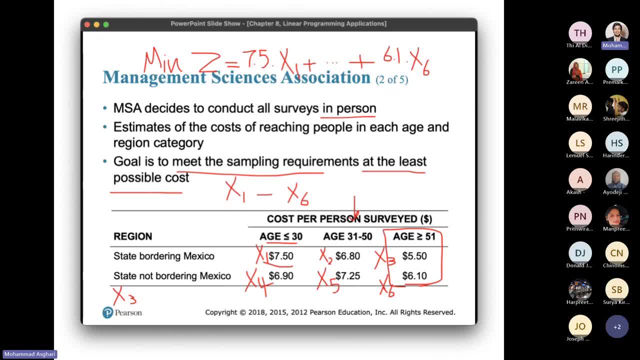 this category in this age must be no more than, less than or equal to 20%. 2. uh, all these people have age more than 51 years old. x3 plus x6. this is the last constraint, um constraint we have. okay, so any questions? so 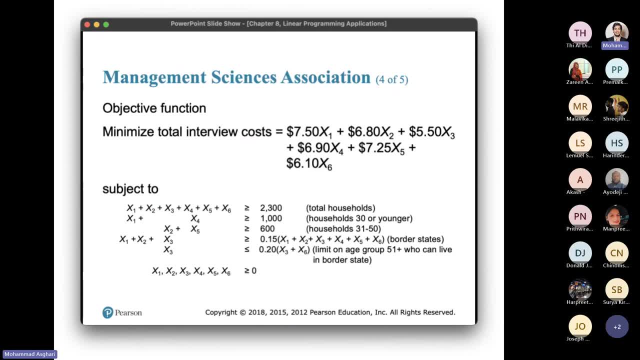 far. in this way, you can write the object function and all constraints in this way. after that you need to add non-negativity constraint at the end of the model. so any question, nothing. the last, the last constraint- i didn't understand it- the um x3. 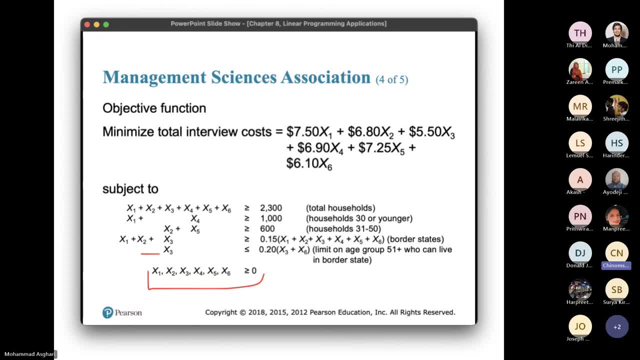 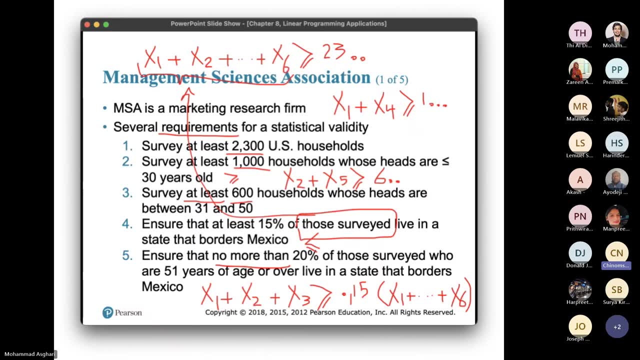 um no more than 20% of the people surveyed. i thought the people surveyed was x1 plus x1 plus x2 plus x3 plus x4 plus x5 plus x6. um, why is it just only x3 and x6? these people, these are. 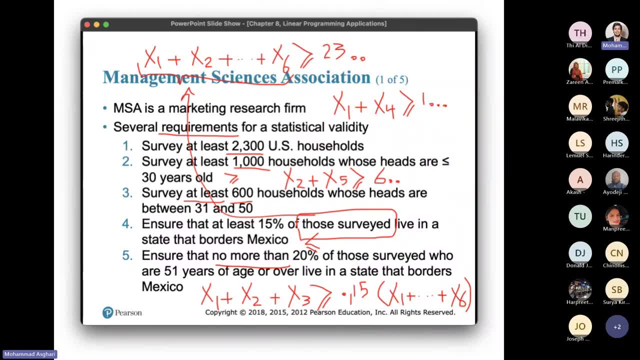 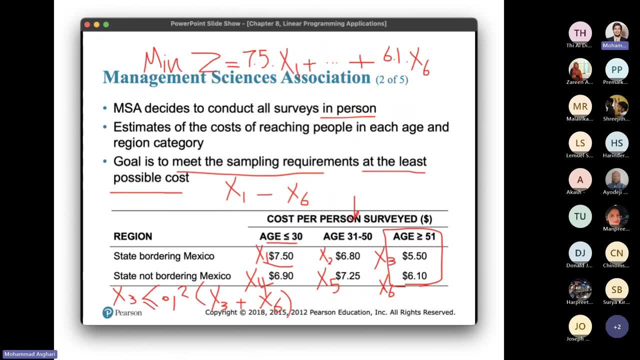 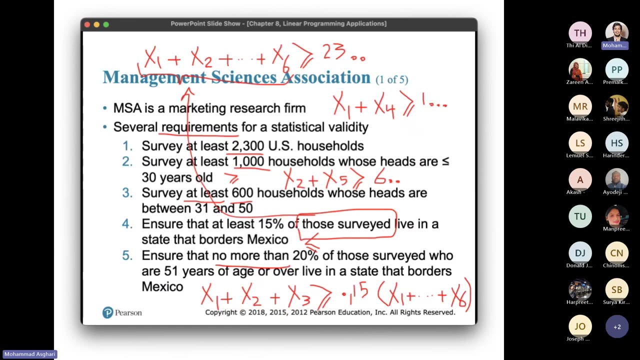 constraints, uh, this constraint um says about that uh, the people in this category, those surveyed who are 51 years old of age, uh, so you can see this category, uh, x3 and x6. okay, so, or live in a state that uh borders mexico, which one of 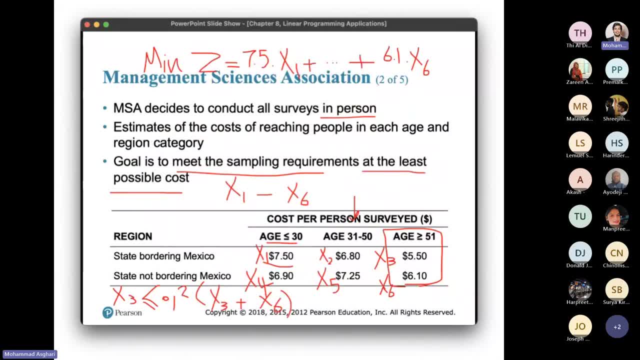 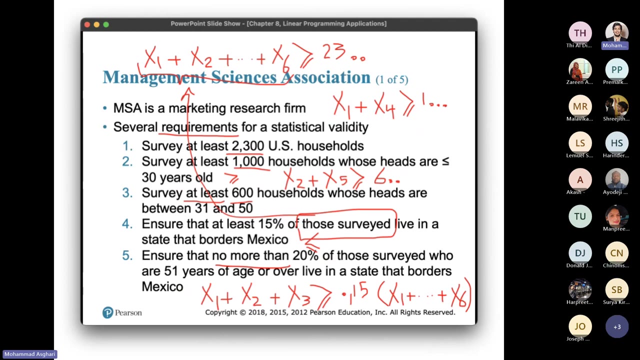 these x3 and x4 uh lives uh. which one of these people lives in a state close to mexico border? this one, that x3. so this constant says that these people- the number of people- lives close to mexico border and have a age more than 51 years old. 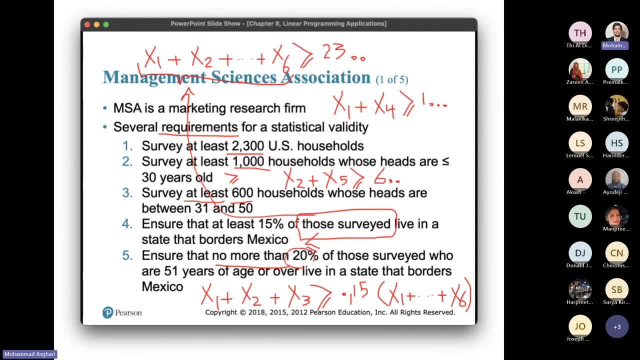 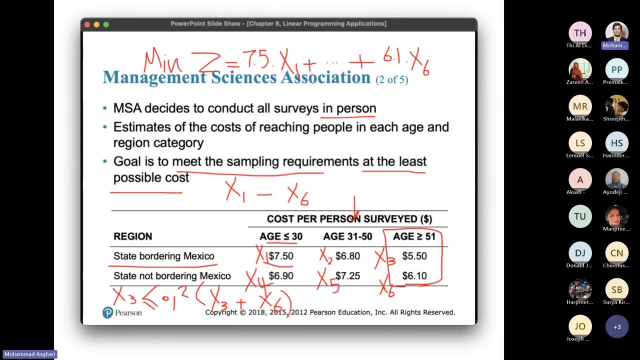 must be less than or equal to 20 percent of those people surveyed or age in this range. the number of people surveyed in this age: x3 and x6, you can find that. so the number of this type of people must be less than or equal to. 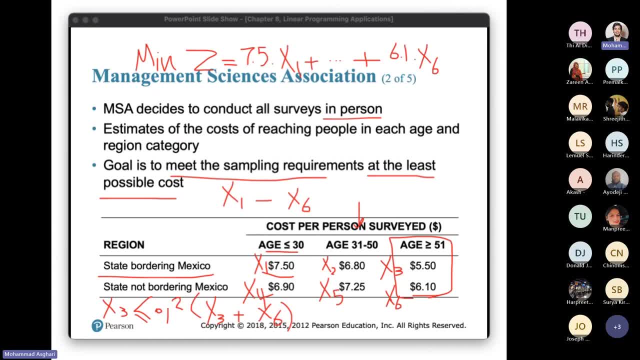 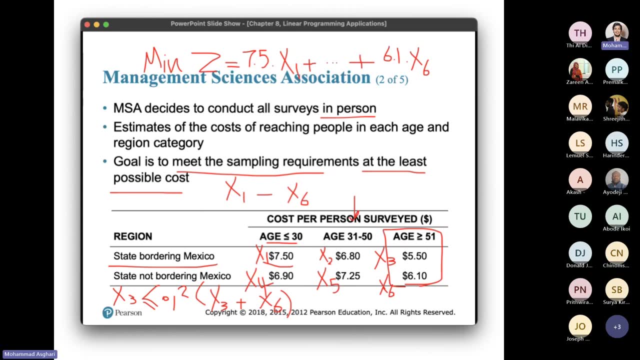 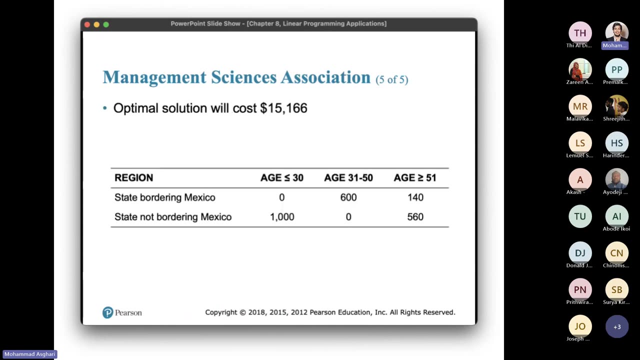 20 percent, 0.2 multiplied the number of people have this age and, uh, they are living close to mexico, or not? okay, yes, thank you, for you're welcome. thank you so much for your question. so, uh, if you have not any question, we can see what is the optimal solution. 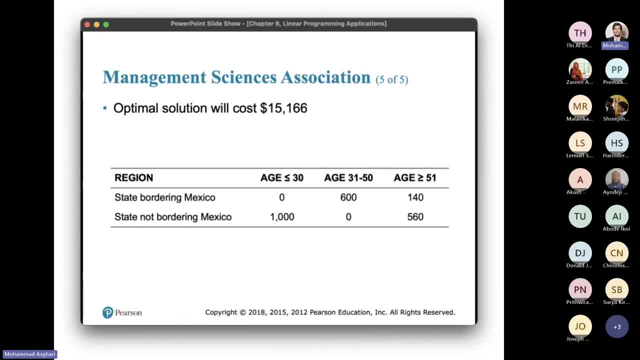 so this is the after solving, the model we can reach to this solution. this is the optimal solution. the value of z and this is the value of x1 to x6- optimal solution. so this uh shows us that you don't need to uh consider any people in this age and 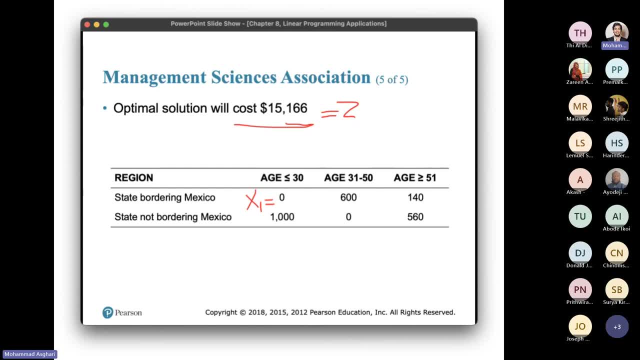 they are living close to mexico, and the number of people, uh, who have age more than 51 years old and, um, they are not living close to mexico must be equal to 460. so this is the optimal value of decision variables and objective function. so you can find. 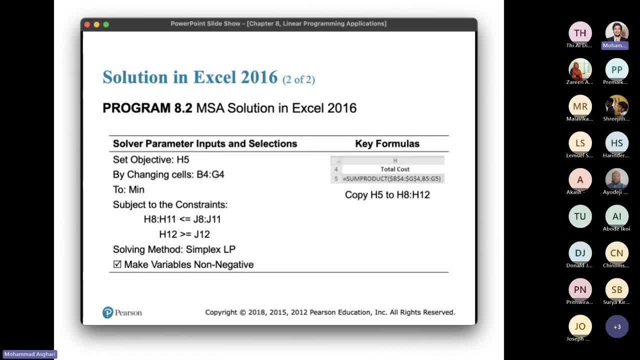 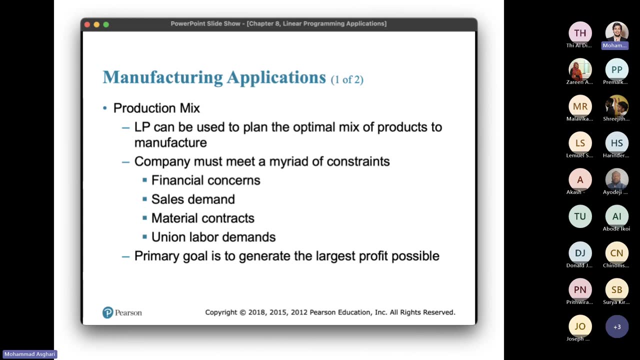 excel file here, but this is optional. you can use excel or any other software to solve it. uh, we are not looking for the solution. uh, the focus here is, uh, how you can write the model. this is the art, um. so, uh, we should skip this one. manufacturing. 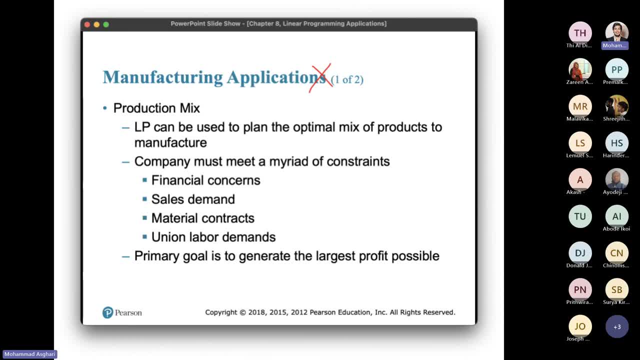 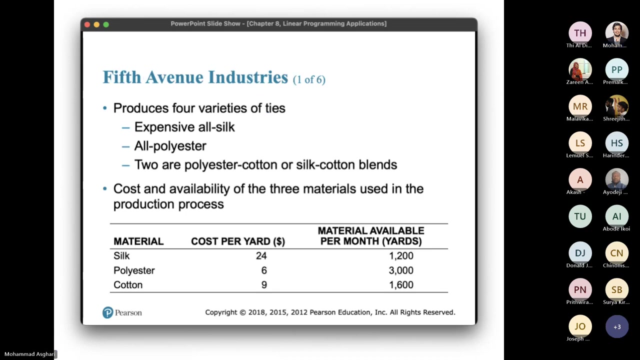 why? because we, um, um, previously, uh, uh, uh, read something um like this one. if you remember, uh, that example, um, was it about tables and chairs? this is exactly the same as uh, that's one. so so you don't need to to, we don't need to spend um more time. 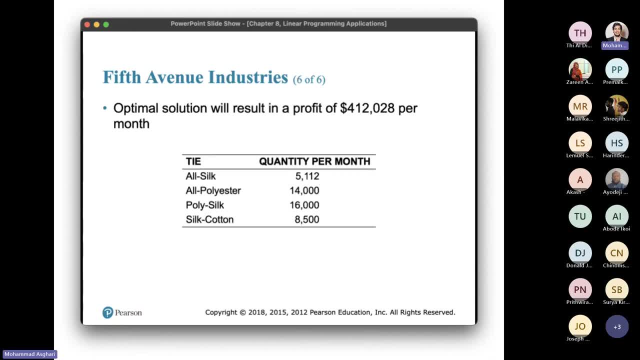 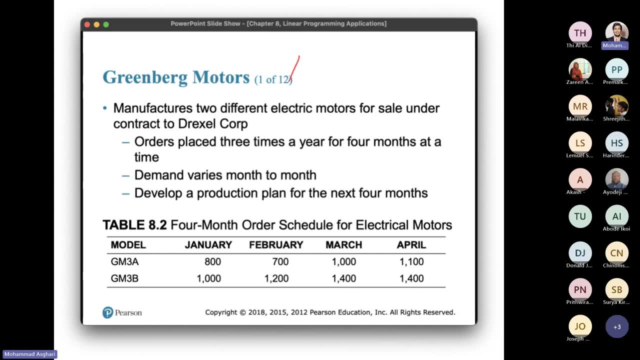 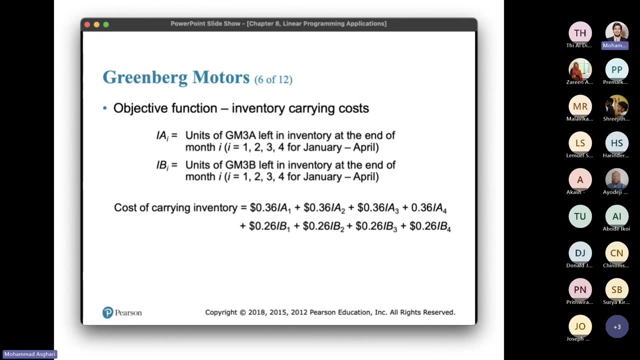 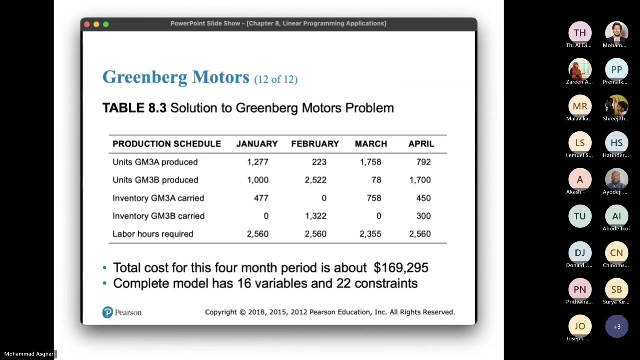 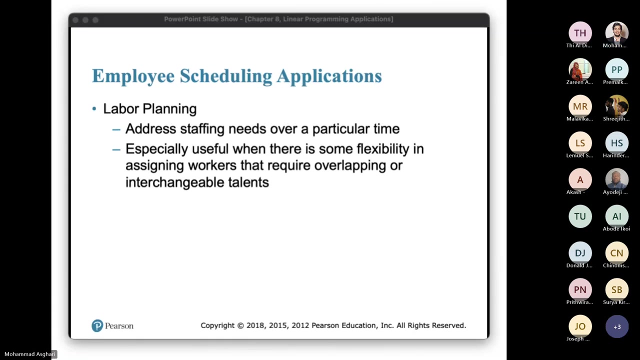 on this example and we just uh practice some complex uh models. this one is so easy, uh, as you can see, the object function constraint is so easy, um, and we skip this one as well. so so, employee scheduling uh applications. now we want to focus on the third category of problems. 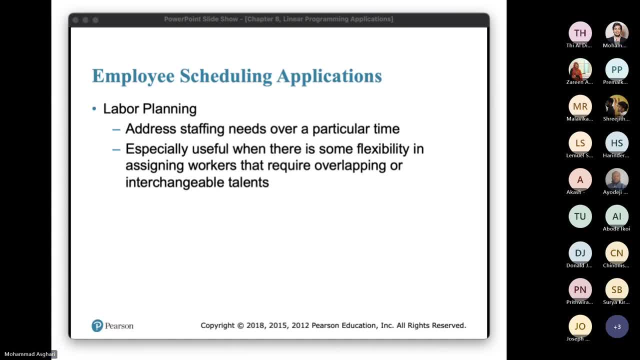 related to applications of linear program. uh, and this is also very interesting because you can use linear programming to schedule how many people uh to hire when they should work and how many um full-time you need, how many part-time you need and how not. much of the 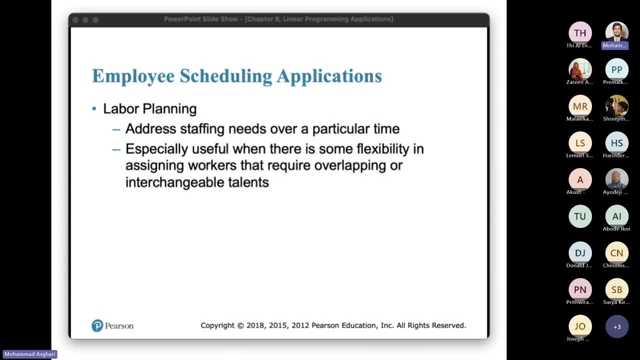 overtime. uh, you need to expand, expand. so these are the typical problems related to employee scheduling. okay, so for uh labor, uh planning, we need to address uh the staffing um needs over a particular time, especially um, it is useful when there is some flexibility in assigning workers. that 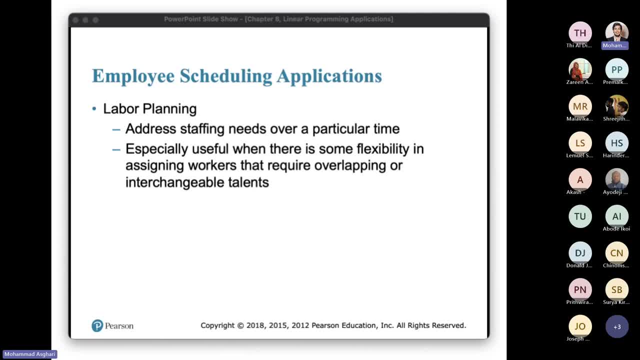 requires overlapping or interchangeable um, talents, or uh. in other words, if there is no limitation, you can hire as many as people you like, but science of operational research and mathematical modeling and quantitative methods are useful, uh, when you have limitations. so it means that you have limited workers. 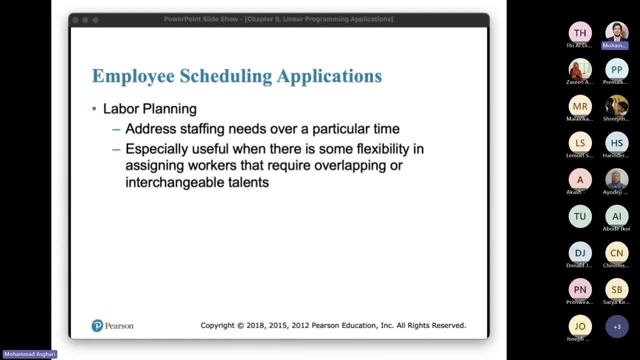 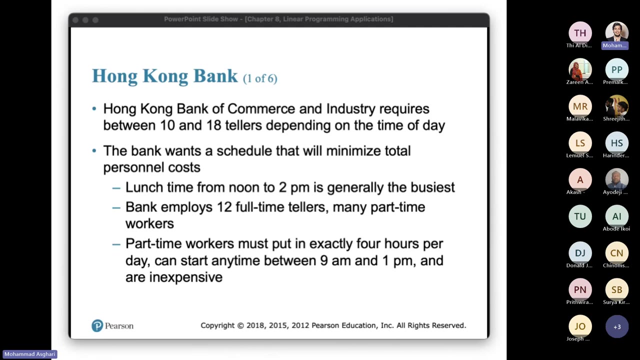 uh limited full-time um or limited um part-time uh workers and you have limited budget as well and you want to minimize your cost when you have limitation, and that's the time that operational research is gonna help you um this uh. give you one example. that's very. 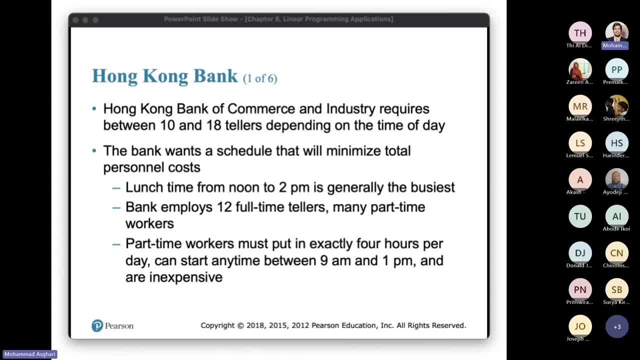 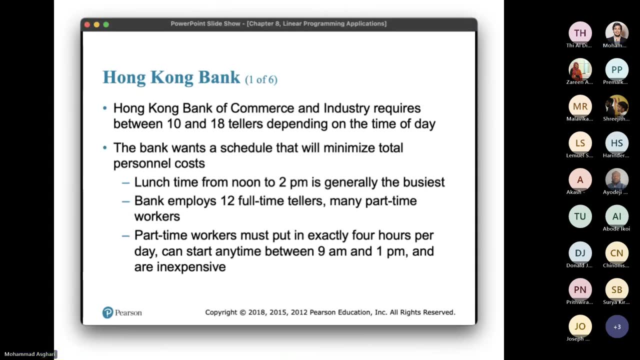 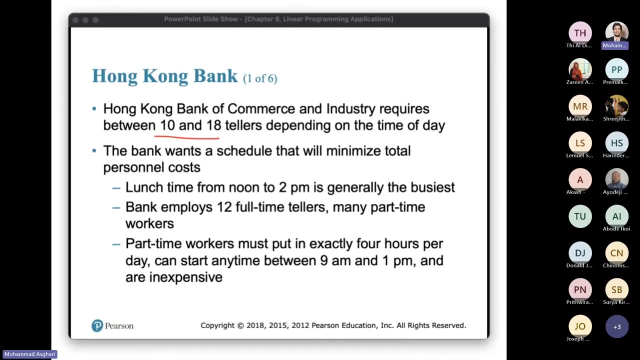 interesting problem. so this is called hong kong uh bank. so this is uh um uh. this bank has uh um between 10 and 18 tellers, depending on the time of days. okay, so you know um in order to manage different hours of day sometimes they have. 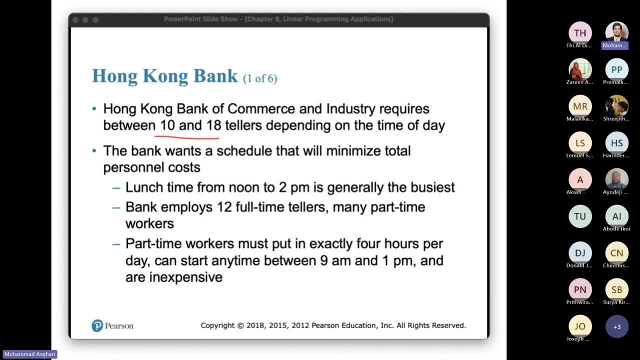 many customers. sometimes they don't have um, so the bank wants to schedule that uh to minimize the total personal costs. so it is clear that what are they are looking for? they are looking for to minimize their cost. okay, so we have um, um, some constraint, let's uh. 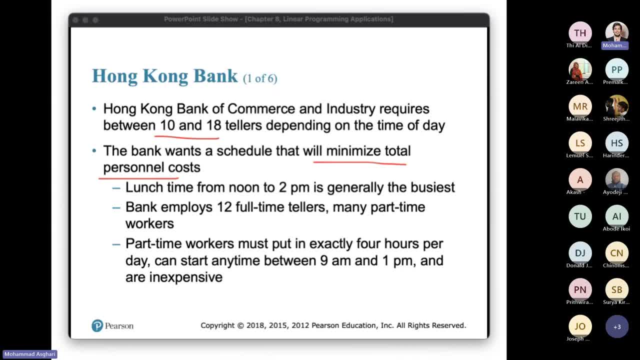 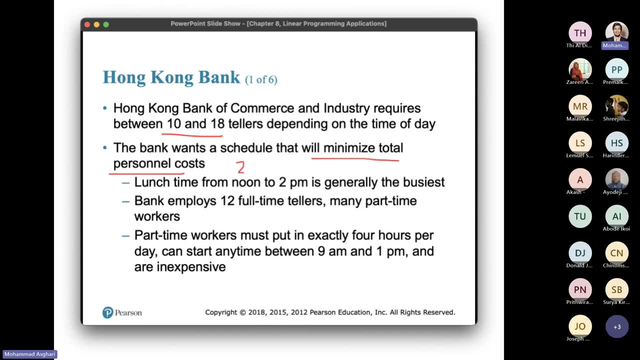 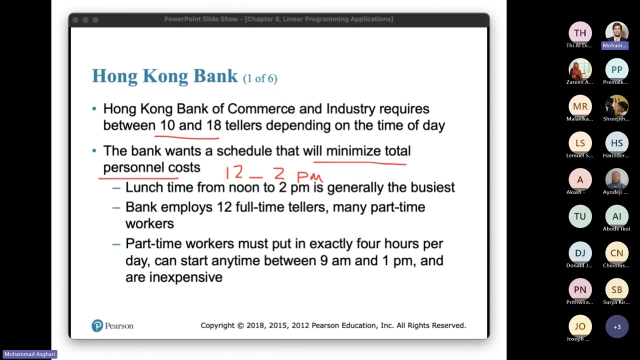 review. uh, what are the constraints? uh, the lunch time, um, from noon to 2 pm, is generally, uh, the busiest time, so we should expect 12 to 2 pm as uh lunch time. so that's the, the, the, the, the, the time that we should make sure that. 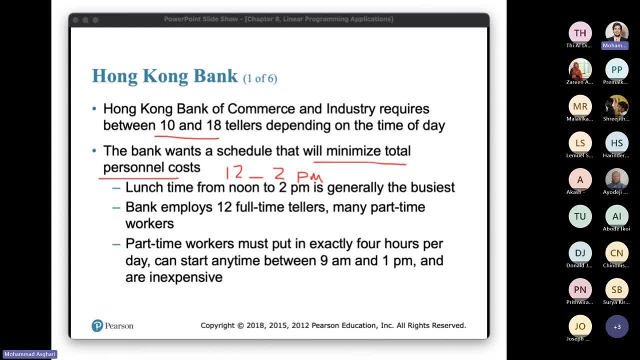 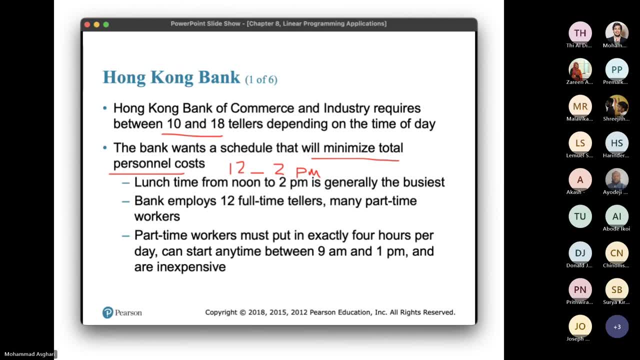 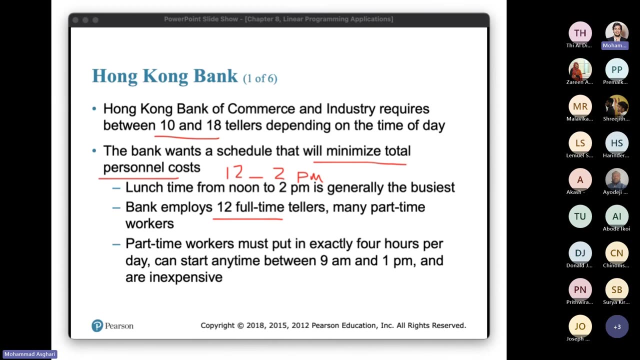 many people are available and the next one back employees employees- two uh full-time tellers at maximum. this is the number of full-time workers and as many as part-time workers they need. they have not any limitation on um hiring part-time workers and part-time workers must. 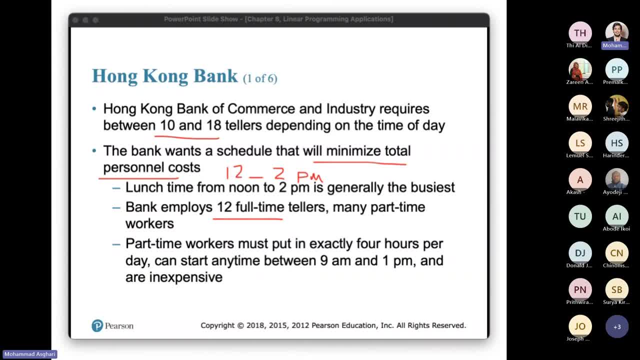 uh work, uh must put in exactly four hours per day. exactly four hours per day, uh, so we don't have very flexible hours, okay, so it means that they uh, that all part-time people that we are hiring, they should work for four hours. okay, they have to. 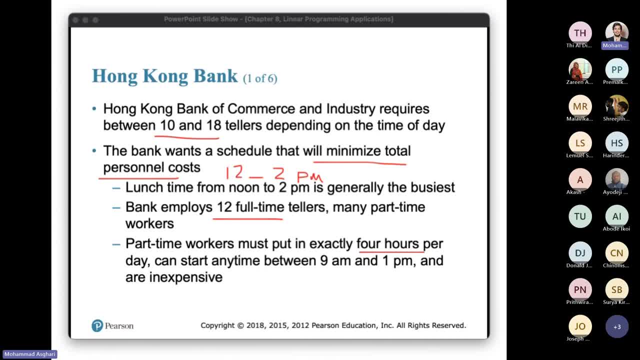 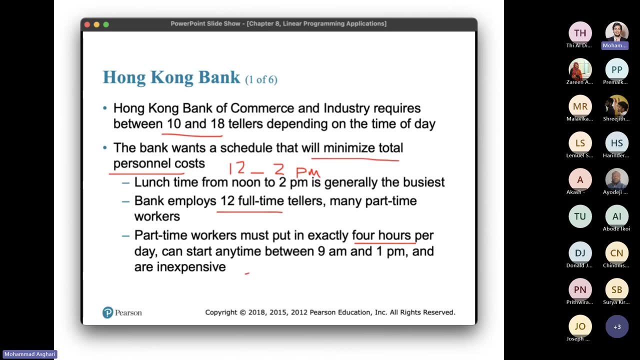 they have no choice uh. the only choice that uh they have uh is when they start uh their work and after they start um their work. so, for example, if they a part-time worker, uh starts from 9 am, so he or she must work for four hours and after four hours. 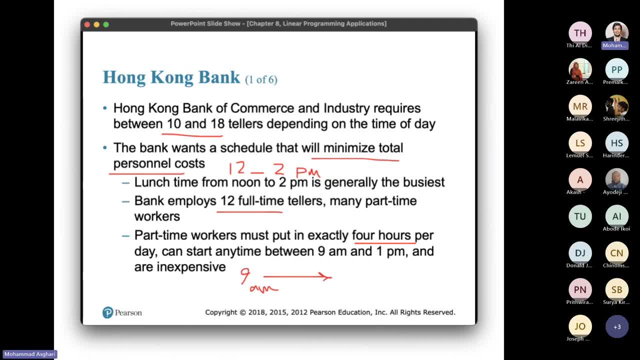 he or she finish uh uh, finish uh uh his job uh in uh 1 pm. okay, he or she uh leaves uh the bank uh at 1 pm, after four hours of working in the bank, for example, and as you can see, for example, if uh someone 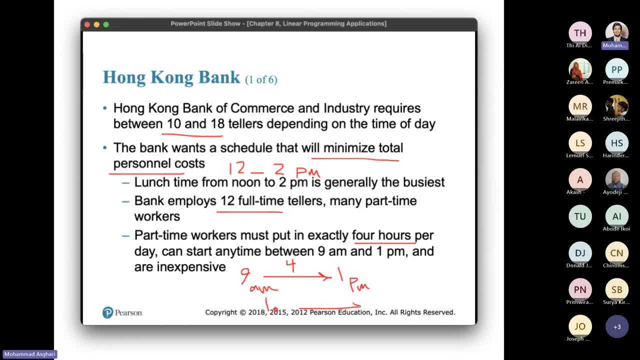 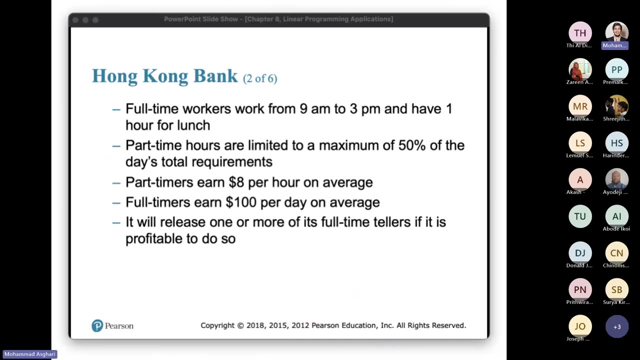 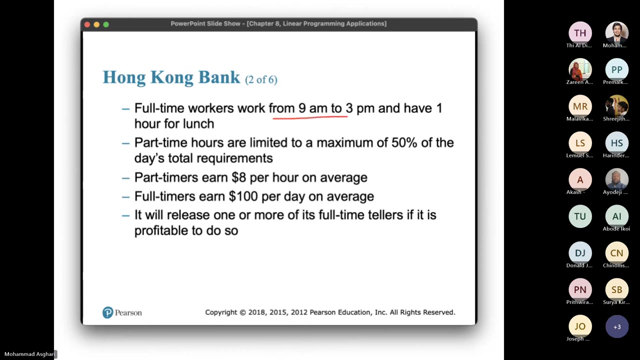 start from 10 again. he or she will uh finish um um his or her job um at 2 pm and must leave back, okay, so um full-time workers uh work from 9 am to 2 pm. so full-time workers um um work from 9 am to. 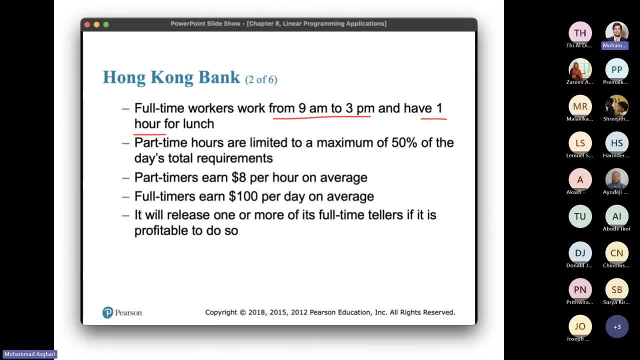 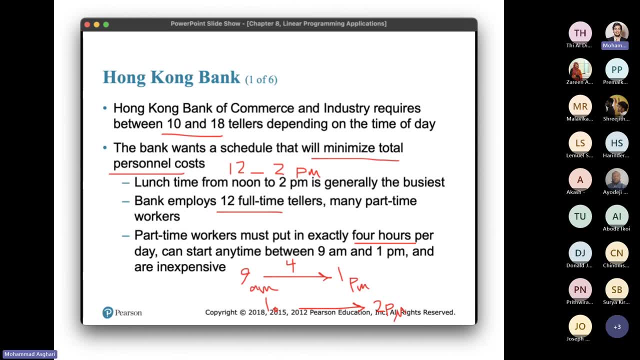 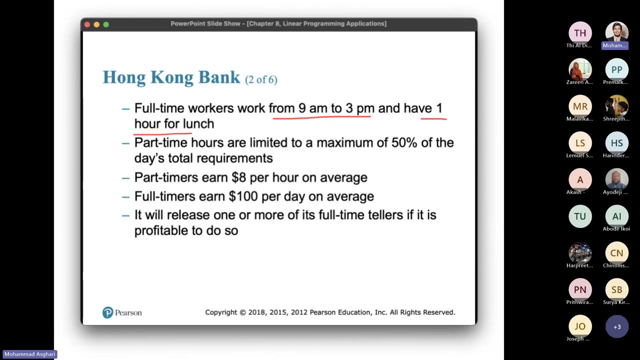 3 pm and they have one hours for lunch. as we can see here, we have uh two hours uh uh period for lunch. uh, it starts from 12 to 2 pm, but each full-time worker have just one hours. uh he, they just um allowed to. 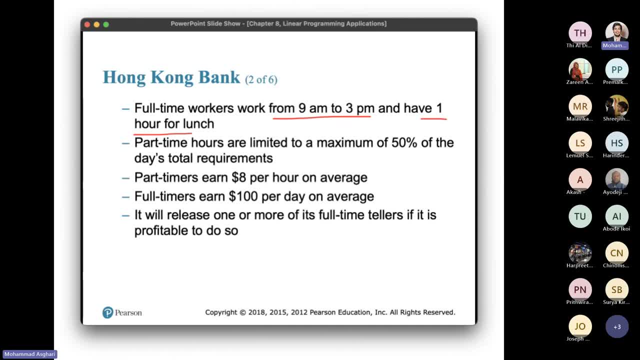 uh leave the work, uh the bank, for one hours or eating um their lunch? okay, and we have not any um uh lunch time for uh part-time workers. so part-time uh hours are limited to a maximum of 50 percent of these total requirements and uh so uh they cannot exceed. 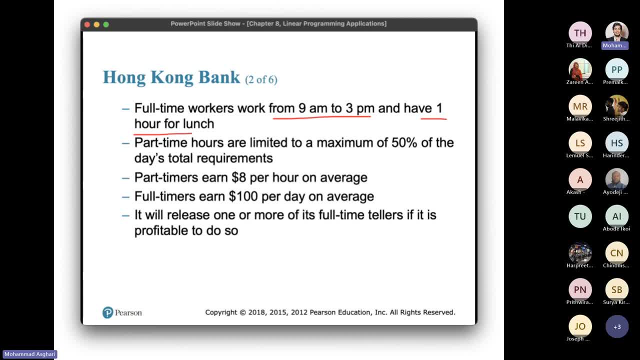 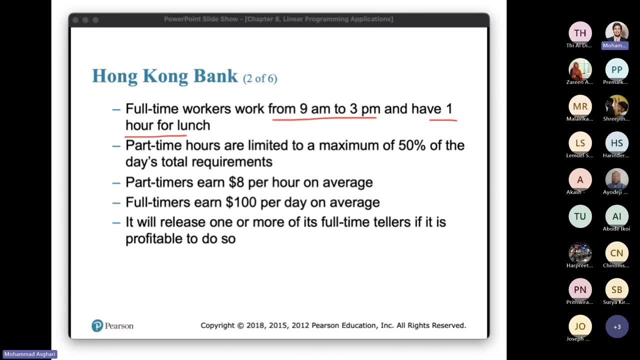 50 percent of uh the uh employee. um uh, so that means that you cannot hire part-time people more than 50 percent of total available time. you should be very careful, because we know that, uh, they are cheaper. we cannot use them more than half. okay, maximum is. 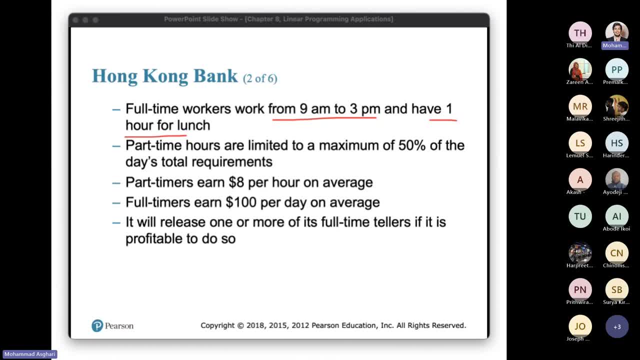 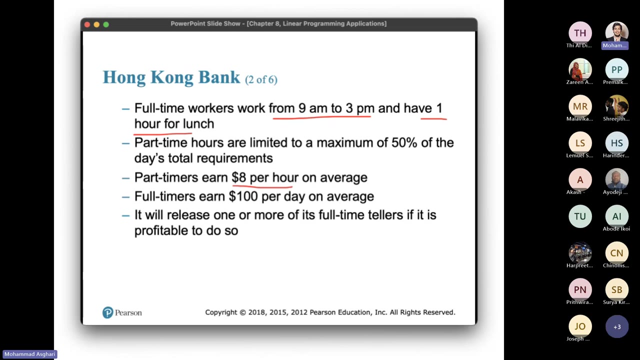 uh is half 50 percent of the personnel. so look at the cost. um part-time earn eight dollar per hours on average and uh full-time personnel, uh earn one hundred dollar per day on average. so huge gap. but uh, you can see here, eight dollar per hour and 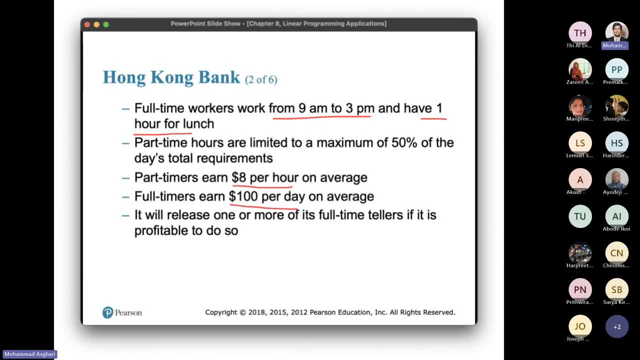 one hundred per day. we know that each part-time worker works for um four hours. we can um convert this, the cost to per day. how we can do that to have the same cost? uh, eight dollar for each hour, and each part-time worker works for four hours. 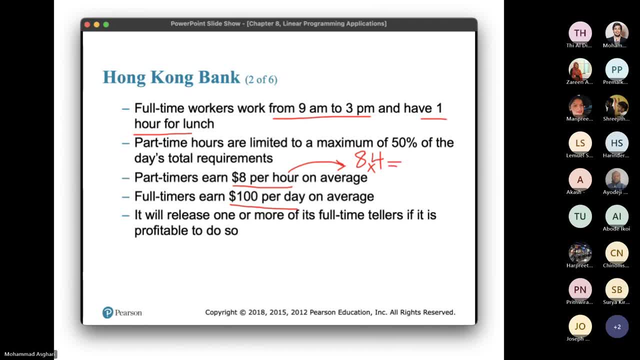 so, so this is the cost of um each part-time workers per day in this way. we we know that uh, the cost per day for both of them, part-time workers and full-time workers, okay, thirty two dollar for each part-time worker and uh, one hundred dollar for each. 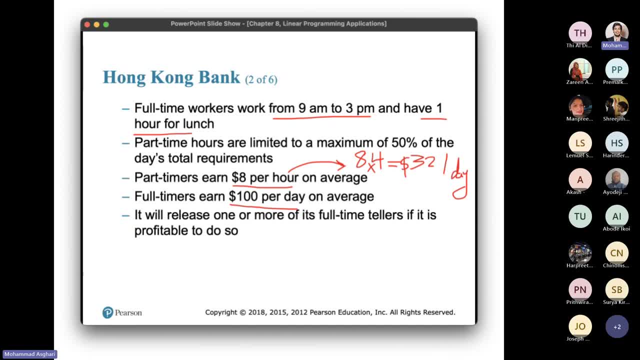 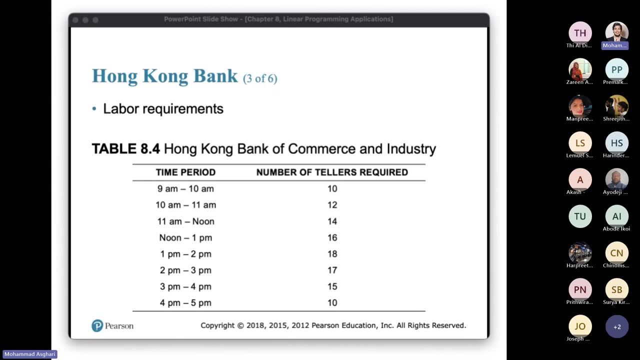 full-time worker. so the last one. it will release one or more of its full-time tellers if it is profitable to do. okay, let's see, uh the table, how many people are needed in different hours so you can see different hours of day. the bank starts. 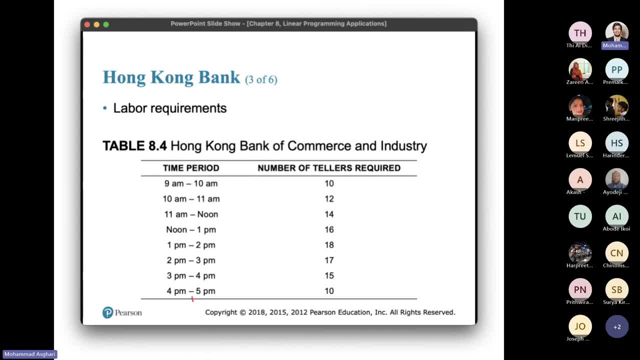 from nine am and uh, the bank will be closed at five pm and in each hours between, for example, nine am to two uh, ten pm, ten am uh, they need um at least ten people in bank and in these uh hours you can see the busiest. 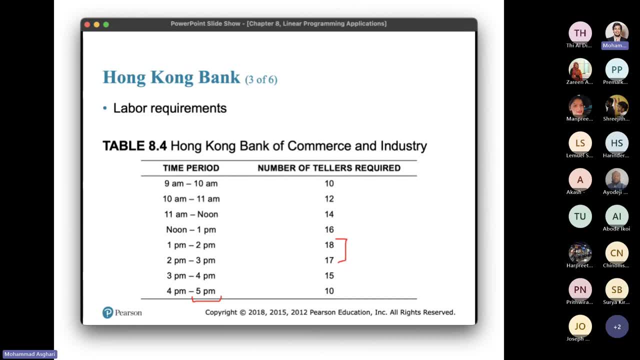 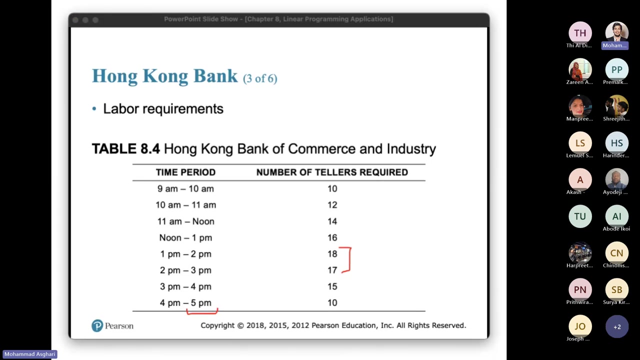 time of a day. they uh need um much more people: eighty workers and seventy tellers between one pm and two pm. so, uh, uh, uh, this is the requirements uh in different hours. so, uh, the first step is to define into uh um decision variables, um. 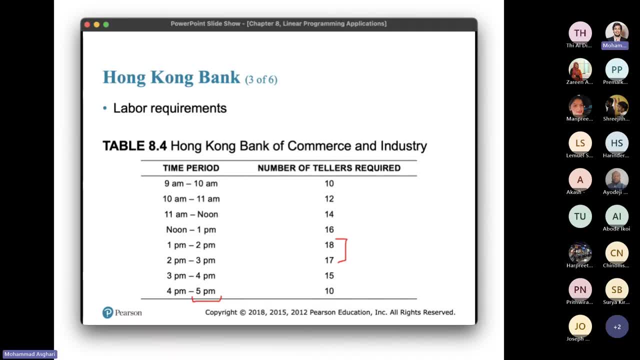 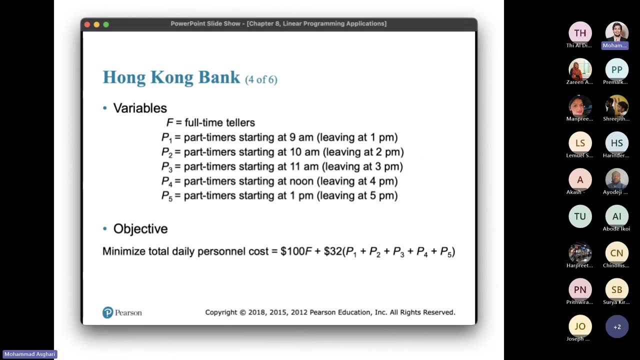 so, um, let me show you how you can decision define. decision variable here is a little bit tricky. you miss. you must be careful in defining that again. uh, you can see the variables here. we can define all full time workers we need in this way, the number of. 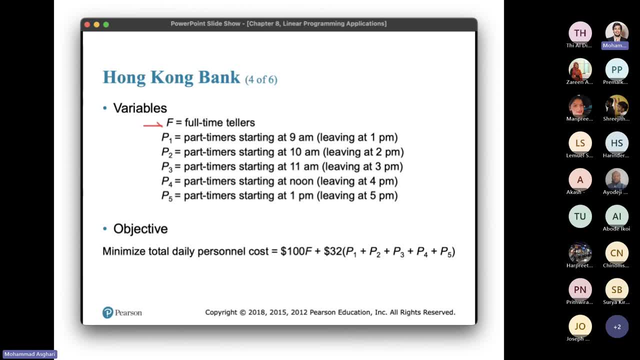 full-time workers. we uh indicate it, then uh with f, the number of the full-time workers, and for each uh part-time workers. in different hours, we defined different decision variables, as you can see, for example, p1 shows us the part-time workers, the number of part-time workers. 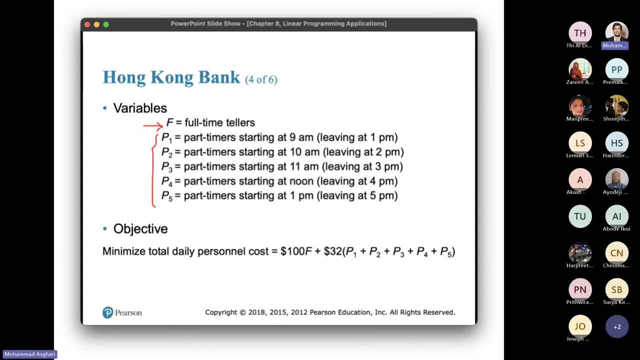 uh who start they work at 9 am and after four hours uh they uh leave at 1 pm. okay, and, as you can see, uh p2 shows us the number of one part-time workers, uh who um starting at 10 am and leaving at 2 pm. 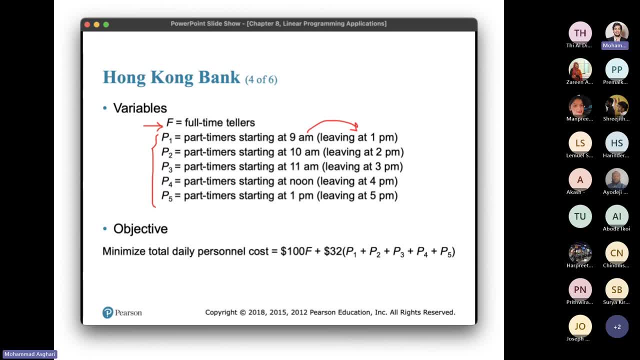 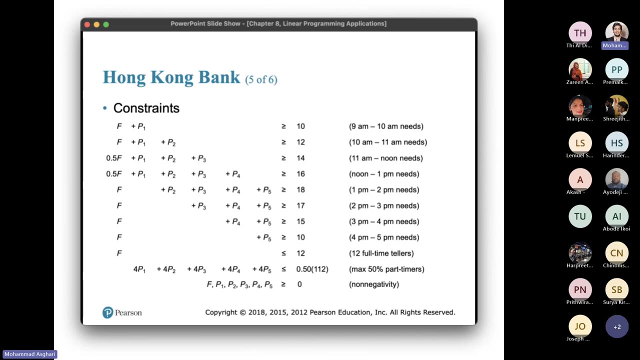 after four hours of working. and the last one that was interesting: p5 shows us the part-time workers starting at 1 pm and leaving at 5 pm. why we have not any part-time workers that start from 2 pm or 3 pm or 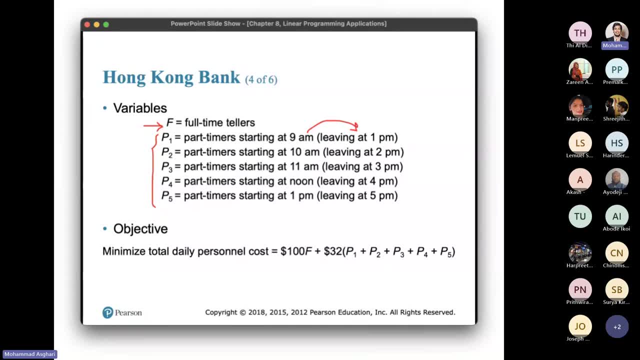 4 pm. why? because they have to work for four hours. if someone, for example, it starts from 3 pm after, uh, four hours of working, uh, he or she must leave at 7 pm. but we know that the bank will be closed, uh, at 5 pm. 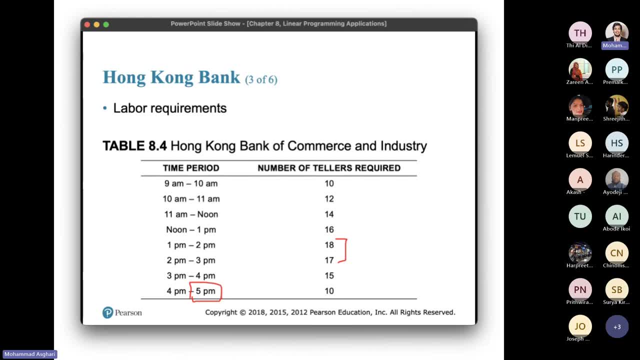 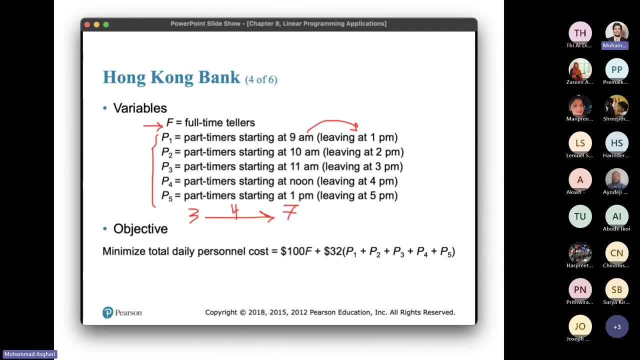 so, uh, if you did uh from this hours, this is the maximum time. that's 1 pm. this is the maximum time that one, a part-time worker, can start their work uh after five hours. uh, they must leave uh the bank at 5 pm. 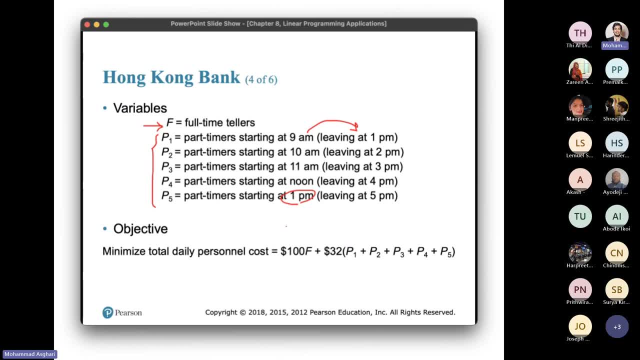 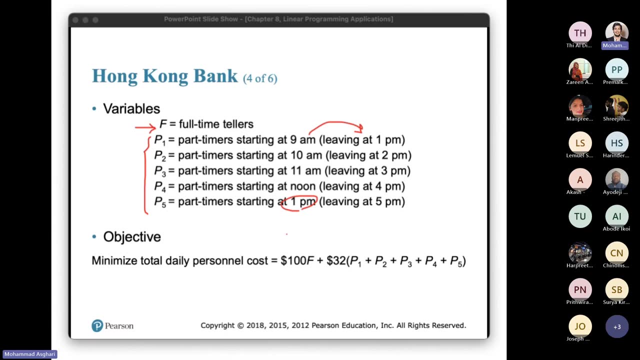 okay, this is uh definition of decision by. so, uh, let's uh consider a break a few minutes. we can start after two minutes break and came back at 10: 40. okay, i will answer your question after break. thank you so much. okay, thank you so much. 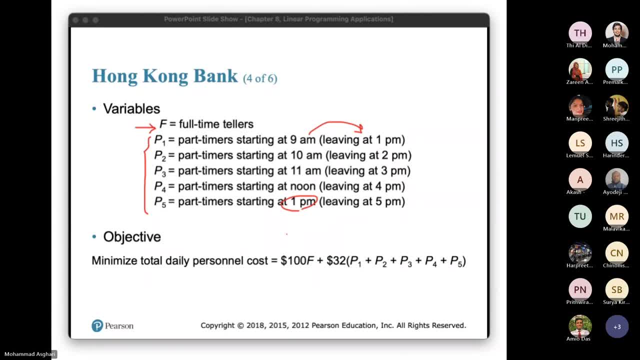 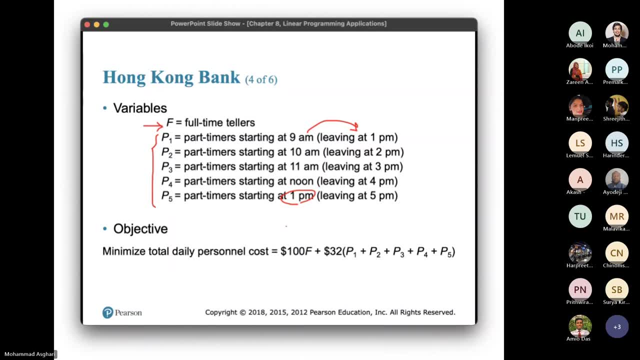 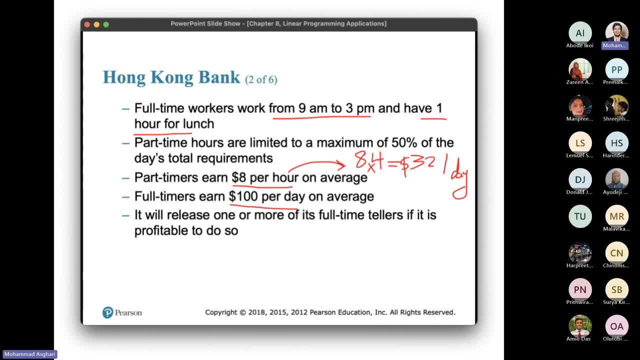 to write objective function. so what is the objective function? you can see here we are trying. the goal is minimize the total personal cost. so we know that the cost of each part-time workers 32 um dollars per day and 100 dollars per day for full-time. 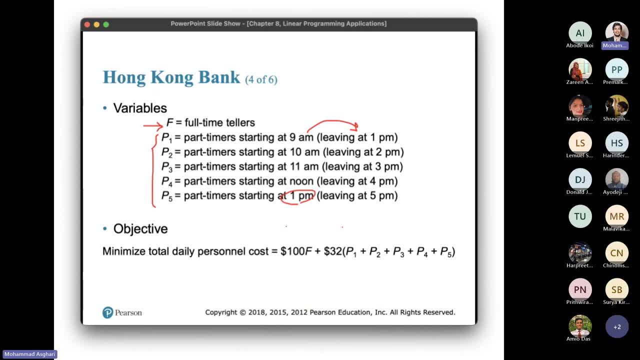 workers. okay, so this is the objective function. the number of full-time workers multiplied 100 dollars per day and the number of part-time workers multiplied the number of uh the uh, the cost you have to pay for uh part-time workers: uh per day: 32 dollars. 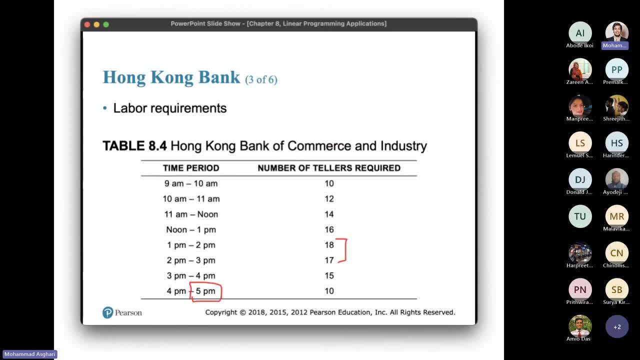 okay, so we should uh now write uh the constraints. uh. so, first of all, in each hours, uh, we need different number of uh tellers and uh, let me um show you how we can write the um the constraints for this one. uh. so, from 9 am to 2 pm, 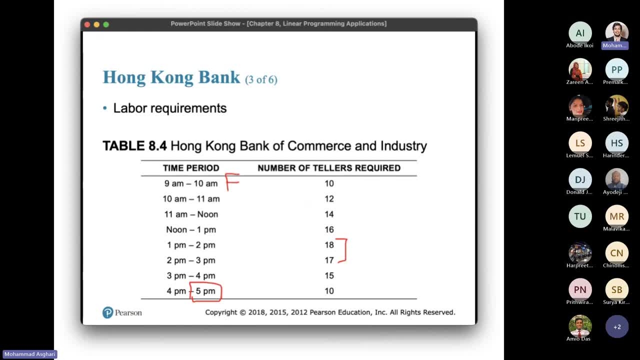 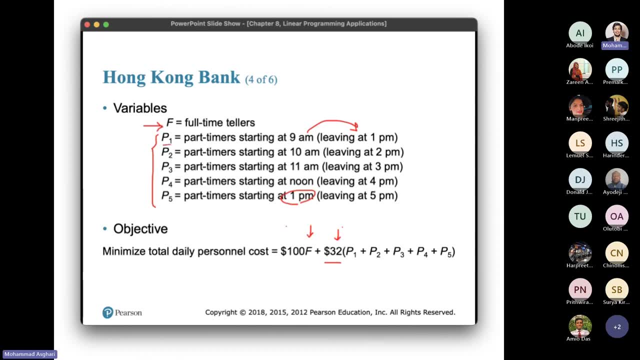 we have full-time workers. okay, and which one of these part-time workers? as you can see, we have only p1 here. uh, who? uh is starting from at 9 am. p2, uh starts. uh starts from 10 pm. we have not them, we have just people here. 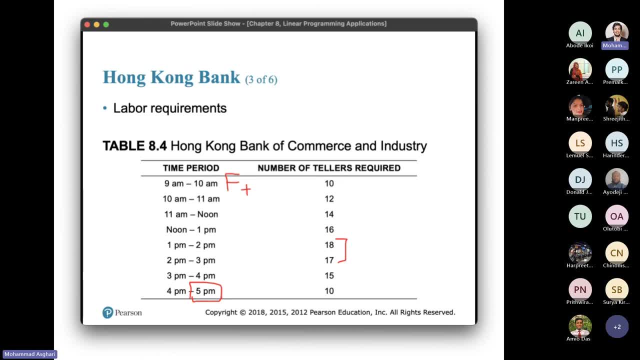 and between 9 am to 2 pm in this period. uh, we have full-time workers and people. they must be greater than or equal to 10 for uh this period. so, uh, we have full-time workers. uh, we have a part-time workers. that uh. 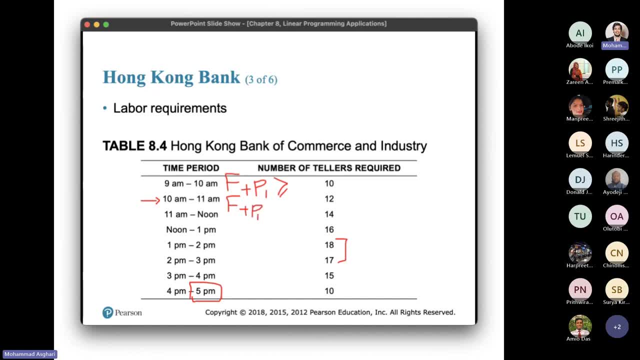 join us. p1, that join us one hour uh sooner, between 9 am to 2 pm, and p2, who is starting at 10 pm. that must be greater than or equal to 12. okay, so we know that p1 starts from. 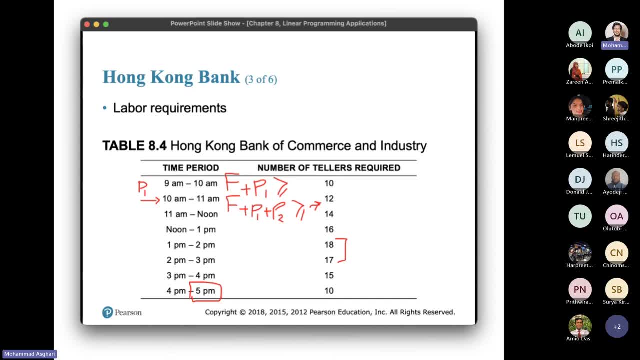 nine uh, again uh, and after four hours they finish. they work uh in 1 pm and here in 1 pm we have not them. so here in 1 pm we have just uh full-time workers, p2, p3 and others. okay, uh, let me um. 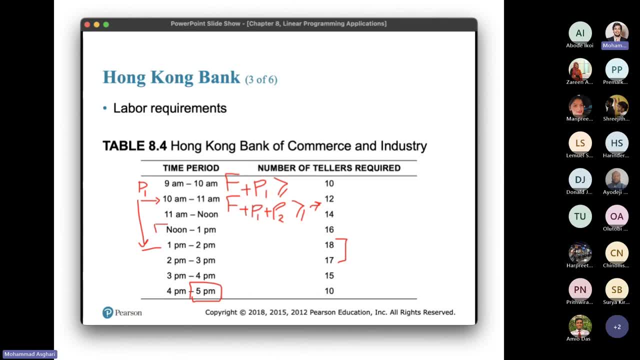 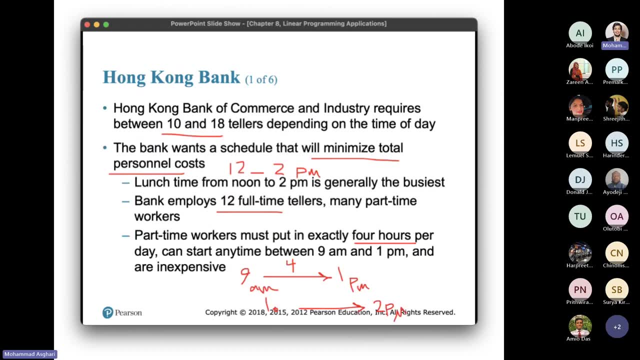 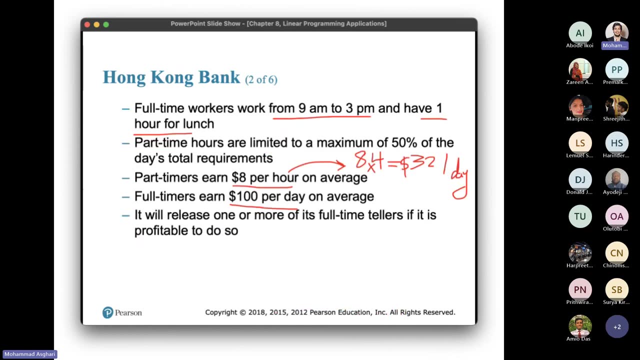 write, uh, one by one- is here between noon and 2 pm that we have a lunch time. so we know that the lunch time is between 12 and noon to 2 pm and each full-time workers have just one hour for lunch. so how we can formulate? 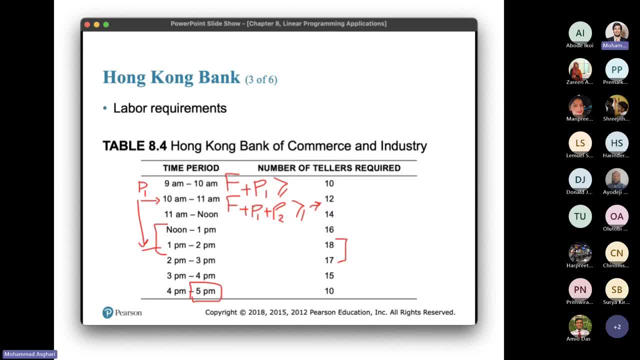 uh this. so we can just consider half of full-time workers, for example, um eat their lunch. uh, full-time workers eat their lunch in between noon and 1 pm and other half eat their lunch between 1 pm and 2 pm. in this way, 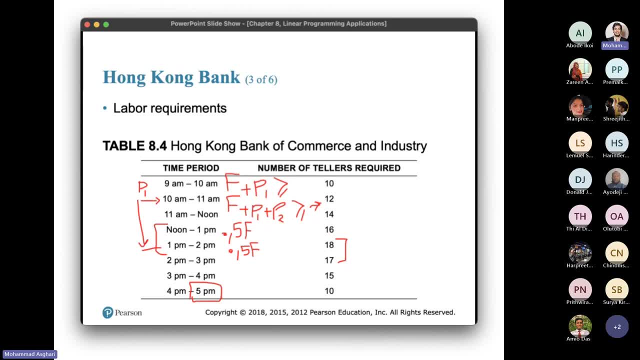 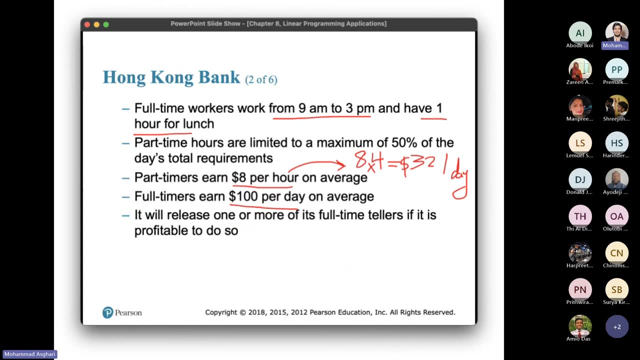 uh. so we just imagine that, uh, 50 percent of them eat their lunch between noon and 1 pm and um other 50 percent, uh, eat the lunch between 1 pm and 2 pm. okay, so for example, you can imagine that in the question. 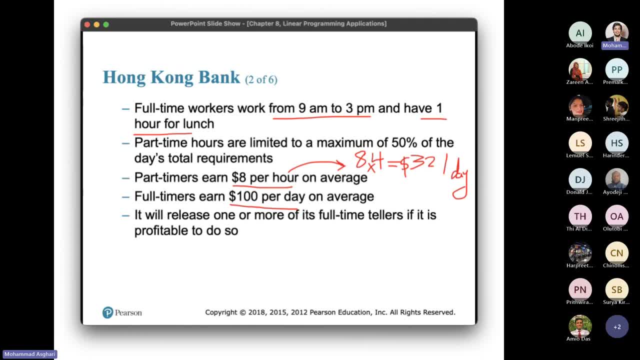 uh. uh brings us that 70 percent, for example, of people eat their lunch between um noon uh and uh 1 pm, and 30 percent of people eat their lunch between 1 pm and 2 pm, if uh in the question um this uh. 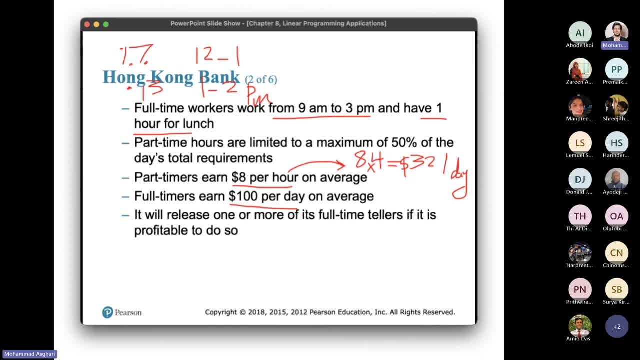 condition uh has been mentioned. we should uh uh write in this way: when we have uh, when 70 percent of employees- full-time uh workers- uh leave the bank for lunch, we have access to 30 percent of them between 12 and 1 pm, so we should. 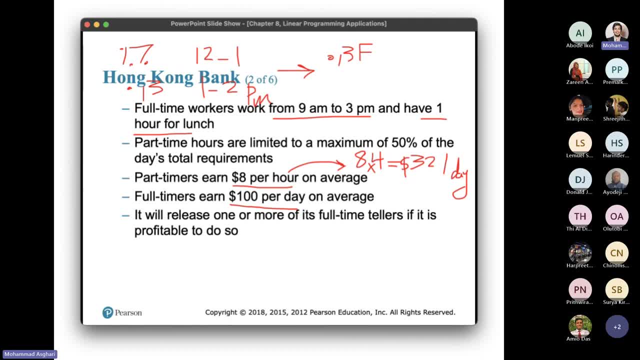 uh multiply 30 percent, or 0.3 to f, and uh we have 30 percent. when 30 percent of full-time workers uh leave the bank for uh eating the lunch between 1 pm and 2 pm. so we have just uh. 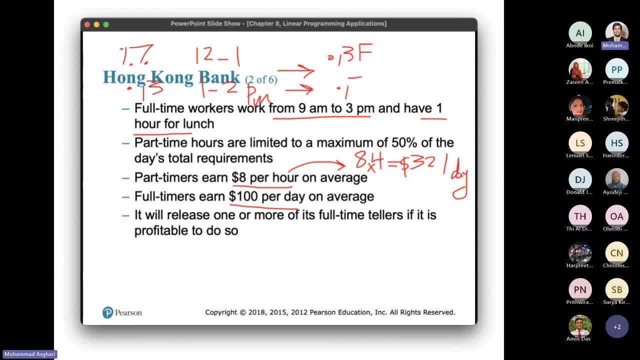 we have access to 70 percent of full-time workers in these hours and we should multiply uh points seven to f, but you can see that there is a, not any condition and um details have not been uh mentioned in the question that how many people of full-time workers. 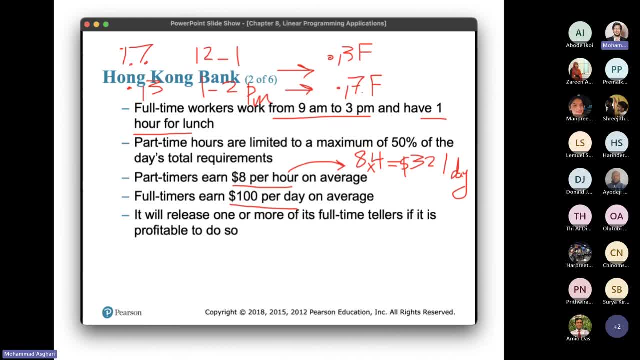 uh live uh between one noon and 1 pm, and how many of them live uh between 1 and 2 pm. so just mention that we have two hours for lunch and each full-time workers. uh. each for uh. each uh full-time workers allowed uh. 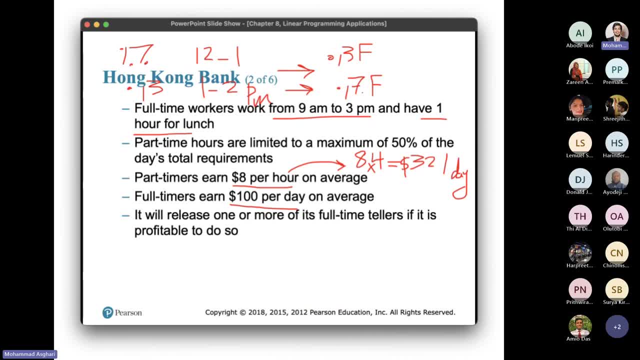 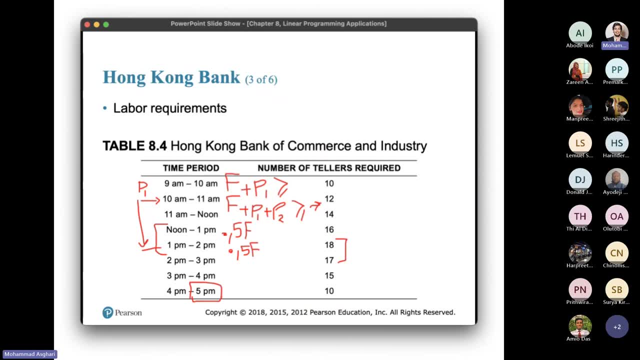 to uh live for one hours for lunch. okay, so in this way, i just imagine that half of them live uh for lunch between noon and 1 pm and other half live between 1 pm and 2 pm. so in this two uh, in this. 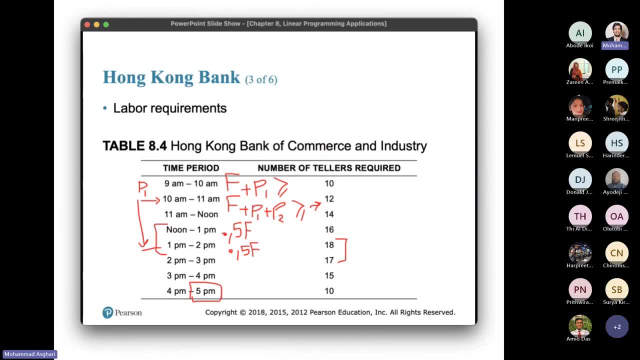 period between noon and 2 pm we have just uh half of full-time workers, and between 2 pm and 30 pm we have all of full-time workers, but after 30 pm we have not any full-time workers. why? because they are. 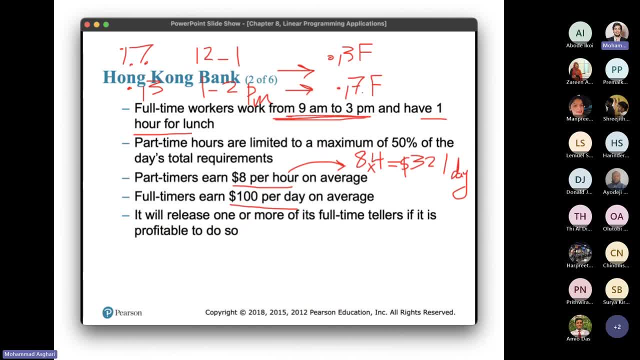 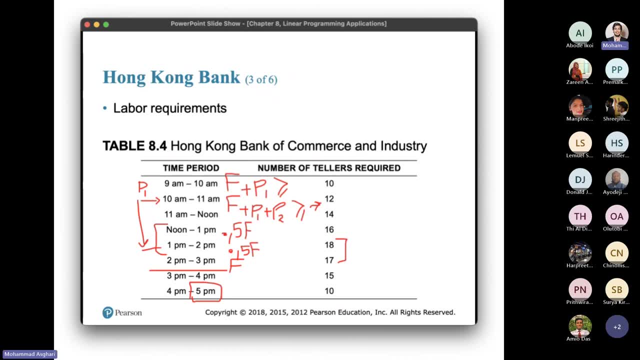 just working between 9 uh am uh to 3 pm. so, um, let me write for noon uh to 1 pm. we have uh- full-time workers, um and uh, we have uh p1. this is the last hour. p1 uh or part-time. 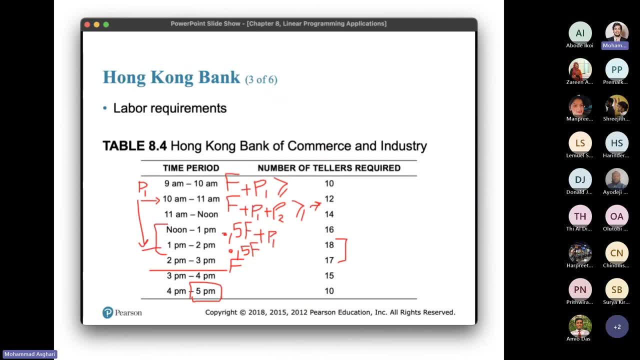 workers, the first part-time workers. uh work for us and after 1 pm they must leave the bank. p2, tell us three, and uh before that must be greater than or equal to this number, 16. so here for uh between 1 pm and 2 pm. 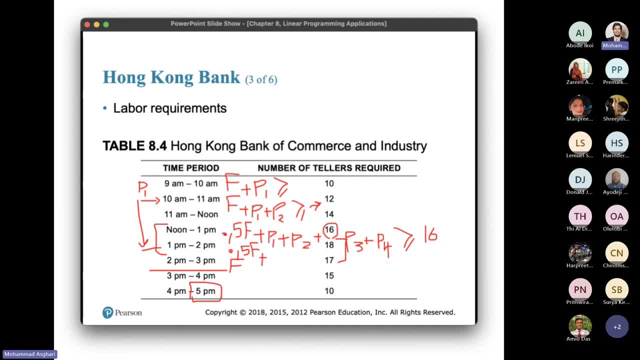 we have not any. this one leaves, um, this type of- uh, these part-time workers leave the bank, so we have just p2, okay, and p2 and others. and for 4 pm let me write for this one. here we have just one type of we. 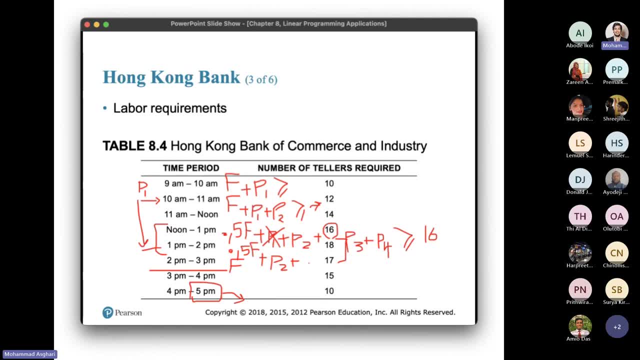 have not full-time workers and all part-time workers, uh, except this one. the last part-time workers before left the bank. so we have just p1- p5. okay, that must be greater than or equal to uh 10, but for this one we have um, p4 and p5. 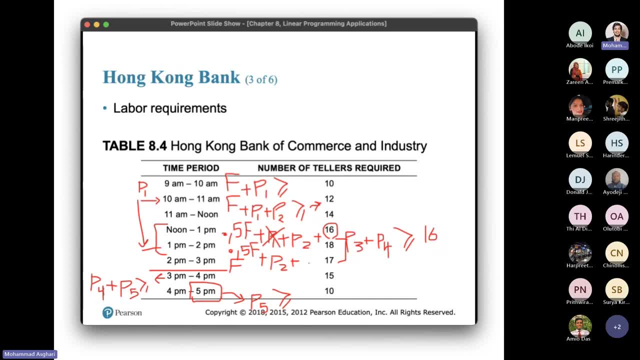 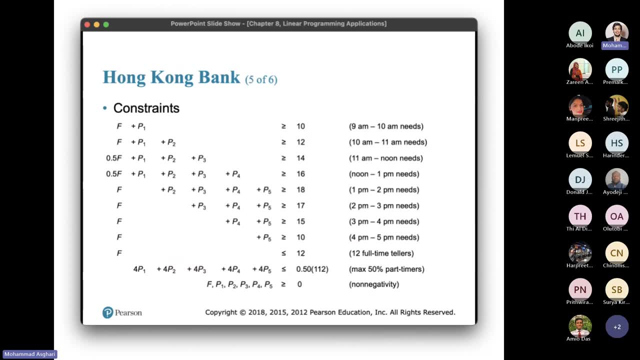 that must be greater than or equal to 15.. so you can see all constraints, all of these constraints here. the first part, okay, but there is some um, um, uh mistakes in these constraints. first of all, uh, we have not any full-time workers after 10. 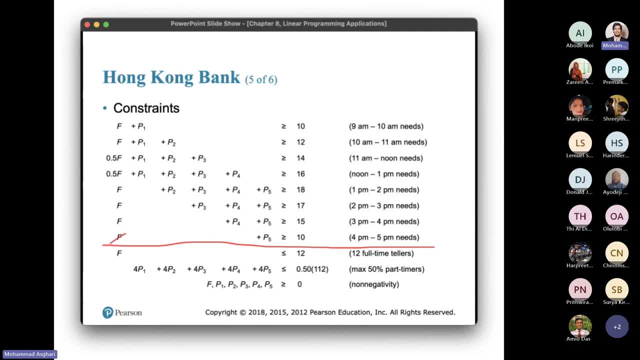 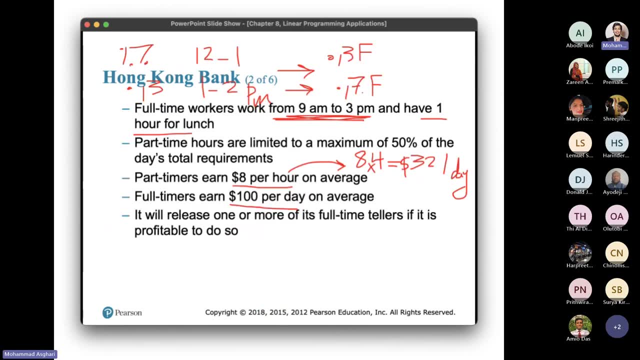 uh, 3 pm. so as you can see in the question, they all work just from 9 am to 3 pm. so you can see in the question, they all work just from 9 am to 3 pm. so we have not them. 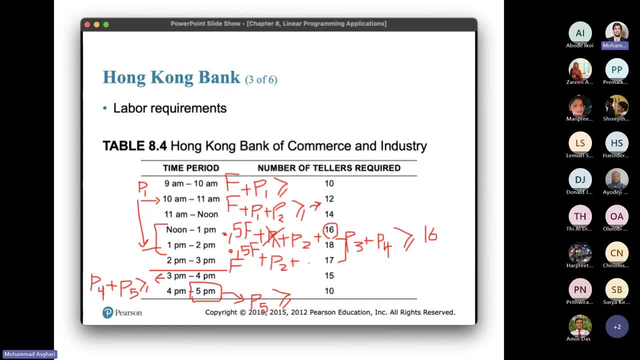 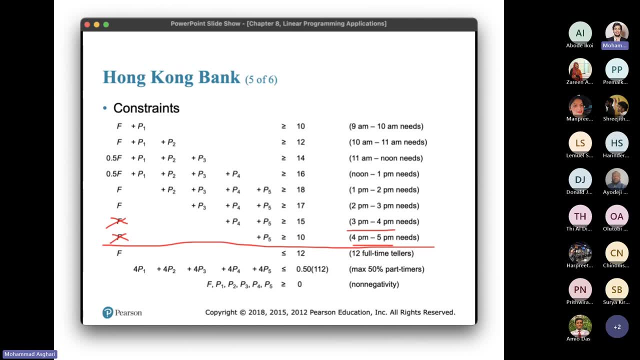 uh after 3 pm, so after 3 pm, between 3 pm and 4 pm, 4 pm and 5 pm. we have just uh part-time workers, not full-time workers. this is the first uh mistake here and um. 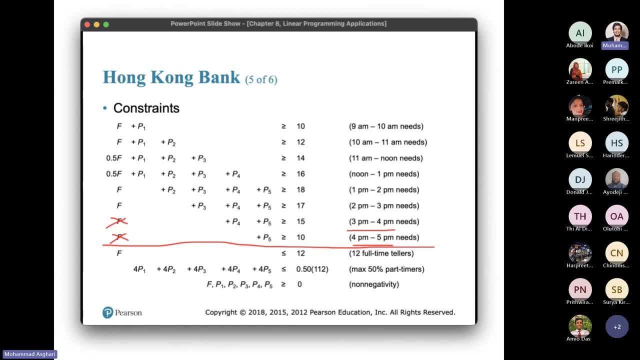 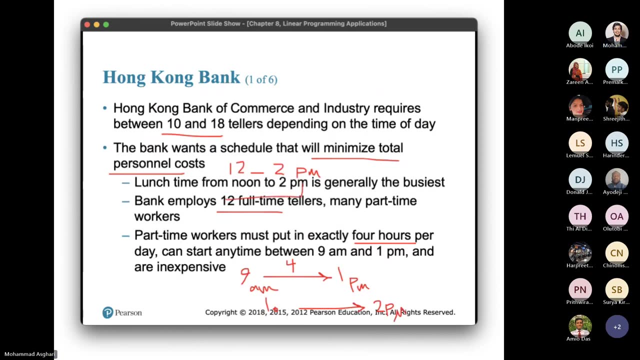 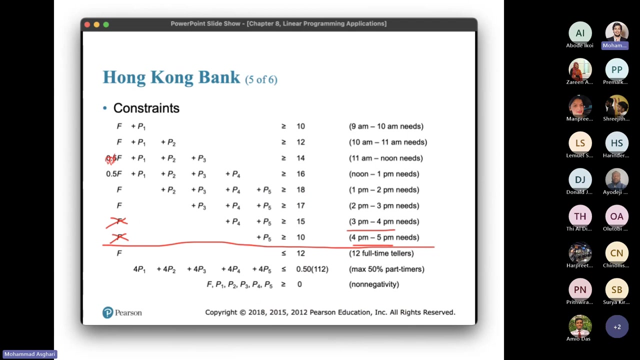 um, um, um, um, and the next one is uh here. and the next one is uh here. lunch time starts from noon to 2 pm. okay, so we have half of these full-time workers here, not in this part between 11 am and noon, we should. 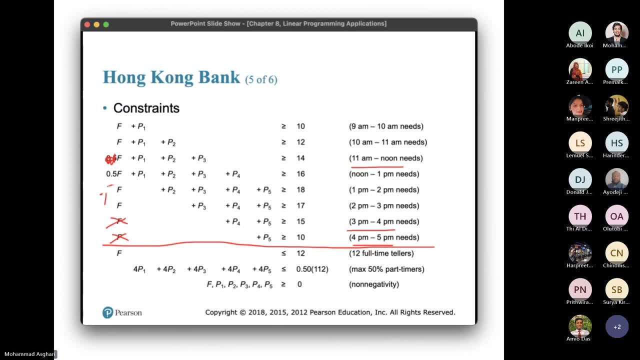 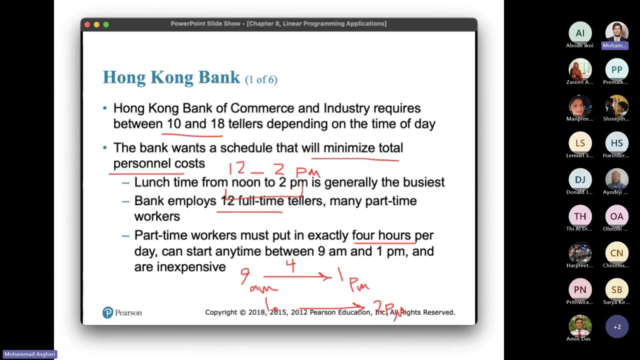 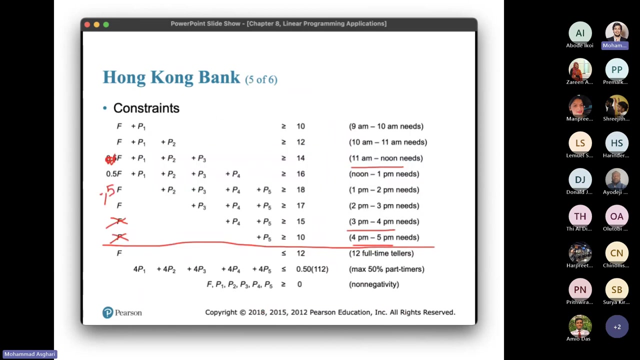 multiply half here. and, and this is the second, mistakes um in the constraints, so um, uh, we have, uh, some other constraints mentioned in the question, so we should, um, um, hire at maximum 12 full-time workers tellers. so we should uh, uh, uh, uh, uh, uh. 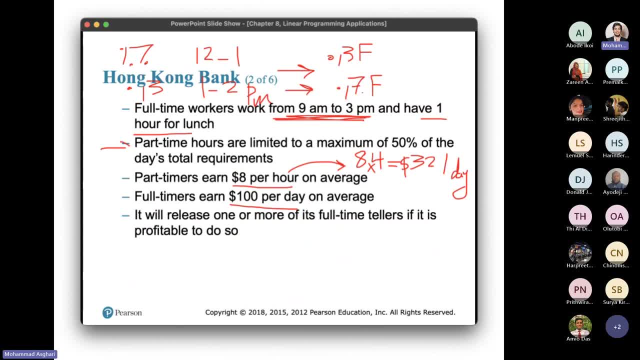 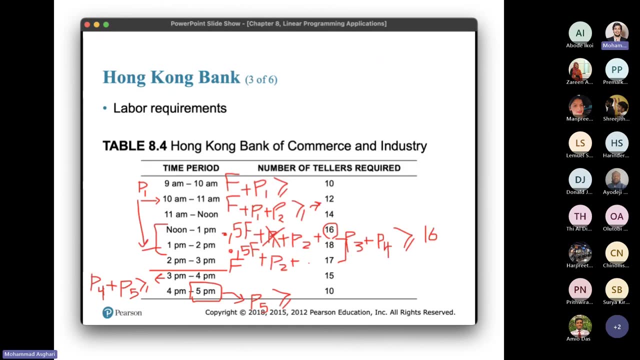 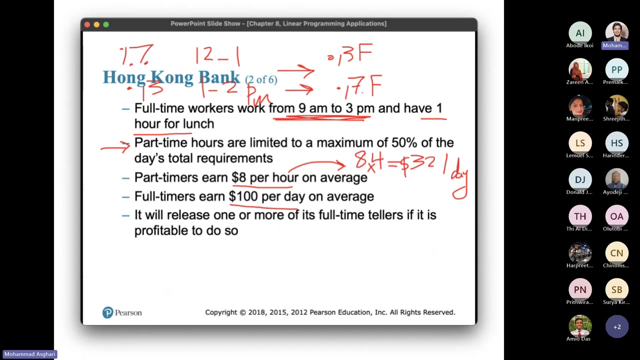 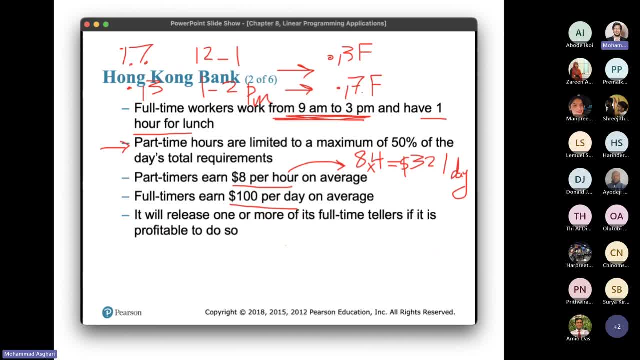 are limited to a maximum That must be less than or equal to: Uh, go on. If you have any question, go on. That must be OK, OK. so why is the number of employees, the number of people that we need in a day? 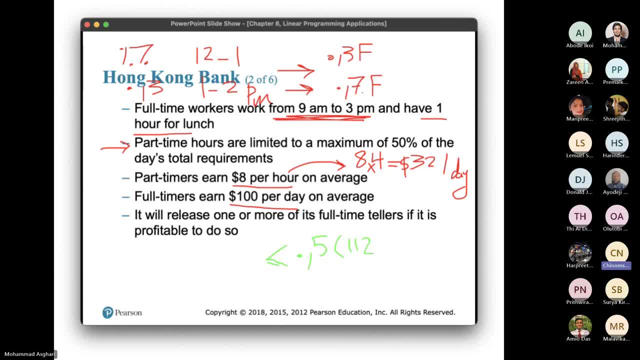 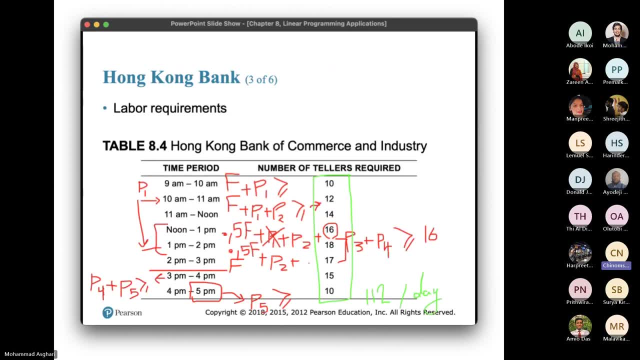 Why is it not just 18?? Why do we have to add up everything? I could you, could you question. I couldn't understand what is exactly your question. No, isn't the total requirements per day? Why do we have to add up everything? 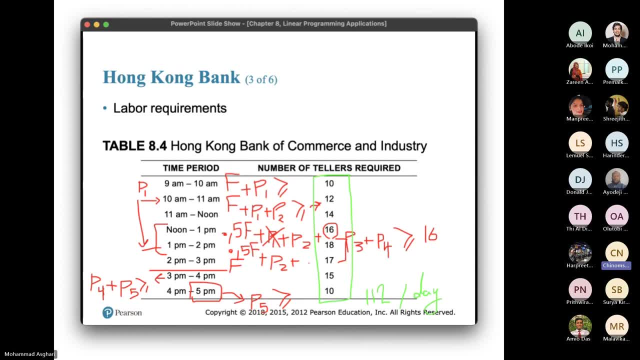 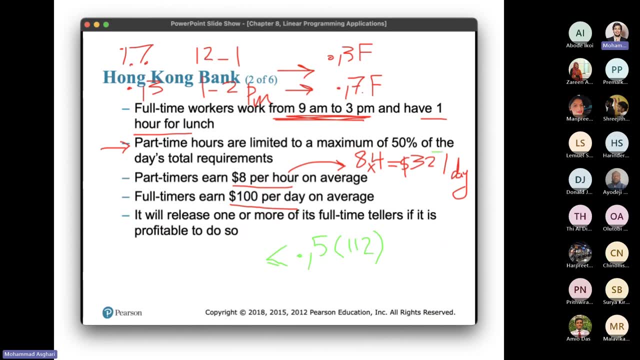 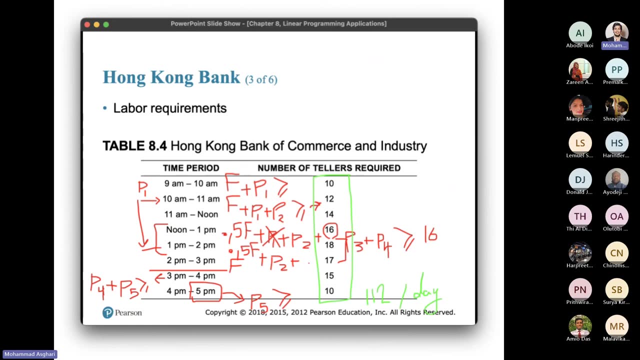 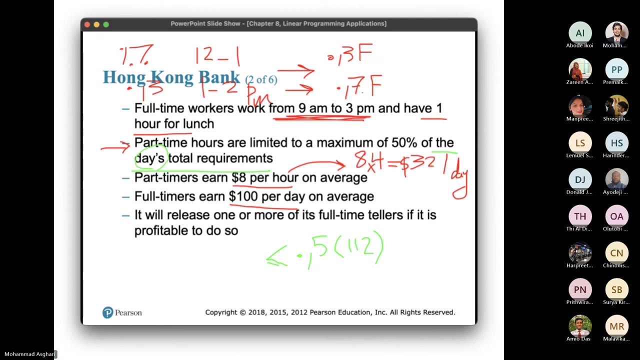 Why is not just the the maximum number 18?? Yes, so this is, as you can see here, the days total requirements. So in each, this is the requirement per hours, But that's mentioned that per day. What is the requirement in day? 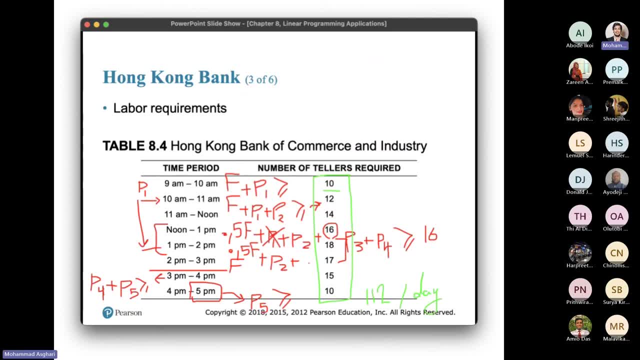 If you want to calculate all requirements per day, you can. you should get a description of all of these numbers here. OK, between 9 AM to 5 PM. Does it mean that these people are not repeated? This? tell us the the ones in 9 AM to 10 AM. 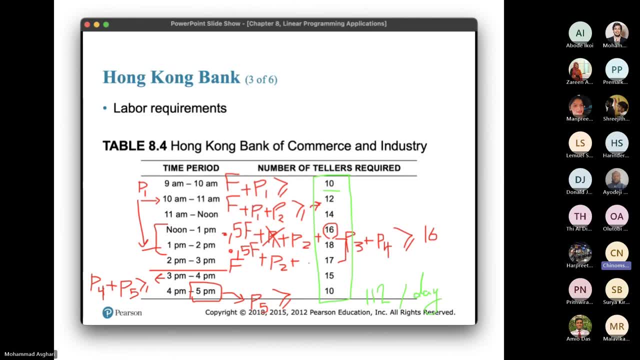 will not be the same ones in 10 AM to 11 AM. They are not repeated. Yes, this is all requirements per hours. For example, when someone pays to you that mentioned that you won't, You work for the, for example, 20 hours per week. 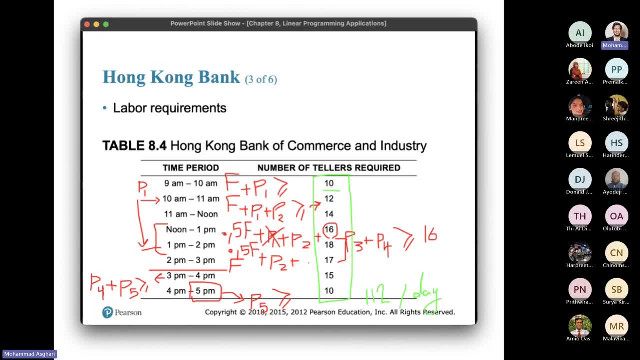 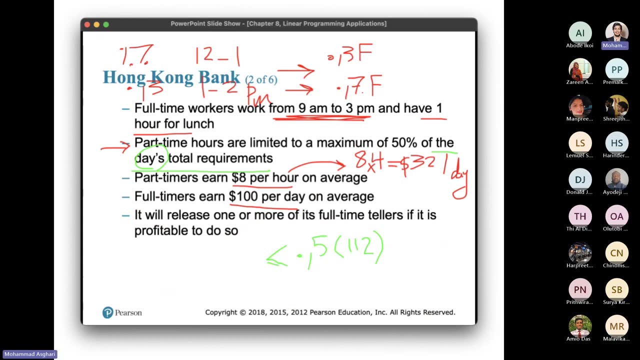 So this is the hours of working. So you just imagine that all requirements per day, that How many number per hours we need per day. OK, so, thank you. OK, you're gone. So the number of part time workers must be less than when we are talking. 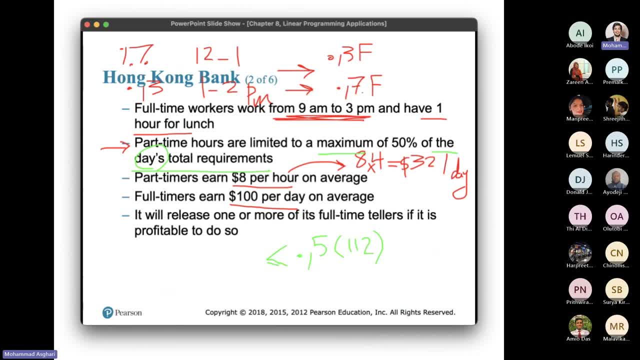 A maximum Of 50% of a total requirement. This is the right hand side of this constant and equation. and when we are talking about the part time hours, we know that each part time workers work for us for hours. For example, P1 works for. 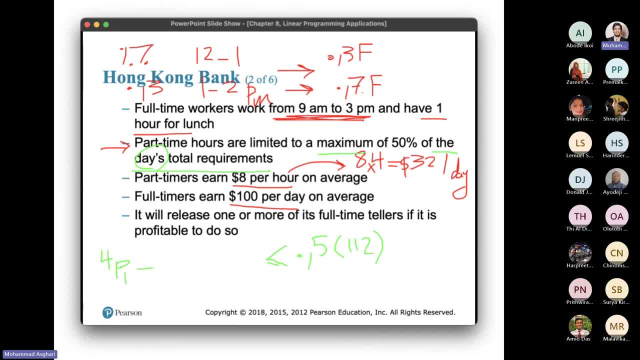 For us for four hours and P2. Works for us for Four hours and all of them You. if you get a summation of all of them, That must be less than or equal to 50% of all requirements. This is the last time of. 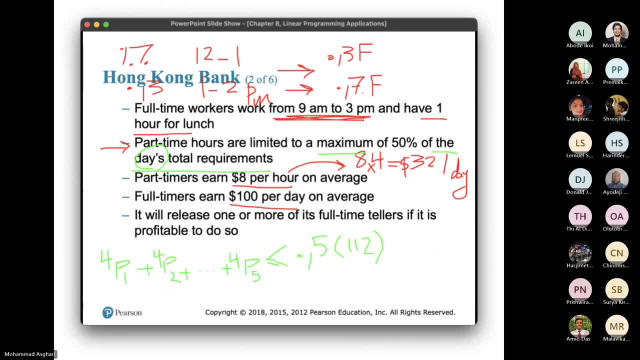 Uh, part time workers P5.. OK, each one works for four hours, So when we are talking about the time part time hours, we need to multiply Part time workers in each house to the number of hours they are working for us. 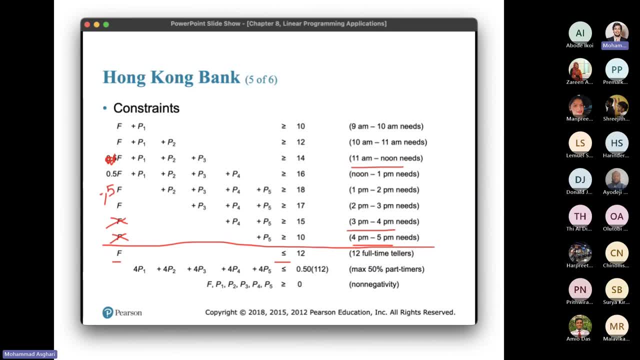 OK, so in this way, You are the last concern. This is the most tricky concern. OK, if you? I know that it looks a little bit complex, uh, um, but you have a, an example here. OK, if you understand this example. 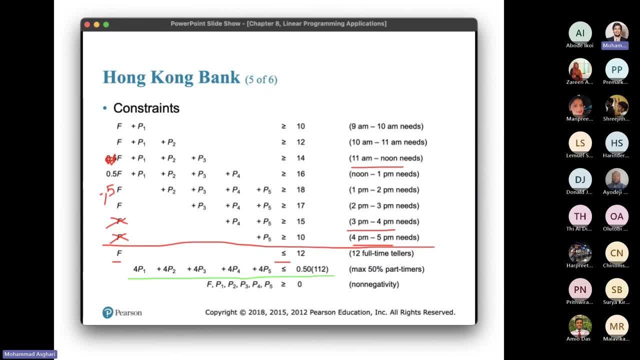 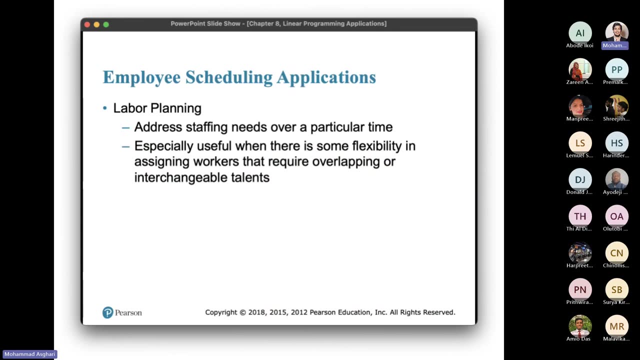 you can easily answer any similar question, So you know that how you can write the constraints and objective function for this type of problem. Employee scheduling application. This is the aim of this class. We are trying to cover all type of linear programs so we can use linear programming applications. 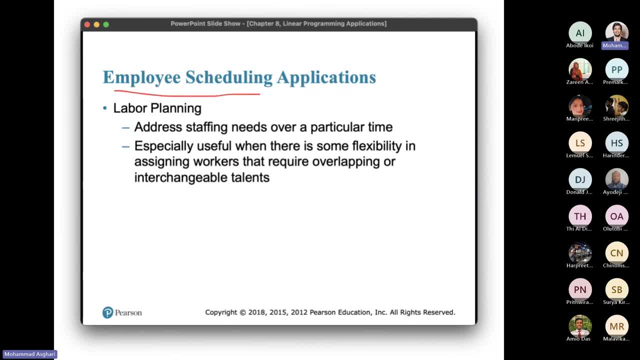 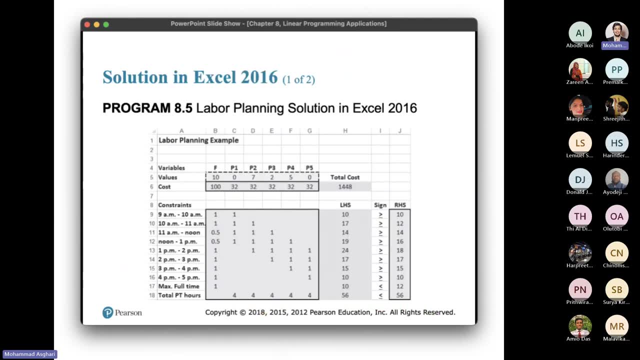 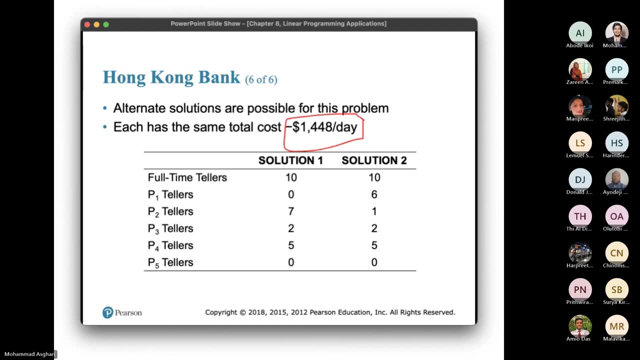 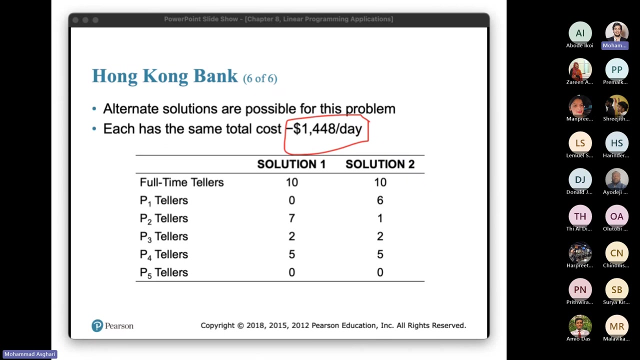 This is one type of problems. You can use linear programming to model this type of problems and find the answer. after solving you, You will reach this solution. This is optimal solution, And so we have. There is an interesting Point here. Now you find that two solution. 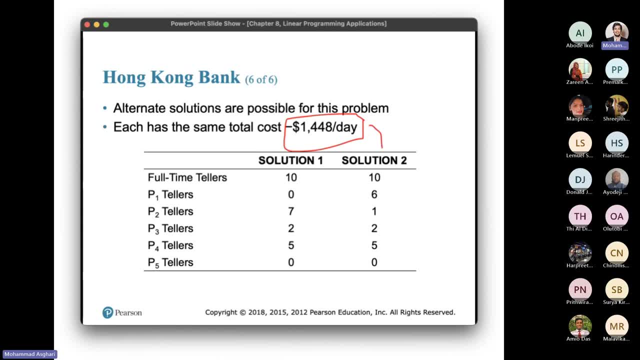 Both of them have the same objective function. This one and this one have the same objective function- Both of them. if you consider, for example, 10 full time workers and zero partial workers, P1 and this number, you will reach the same objective function. 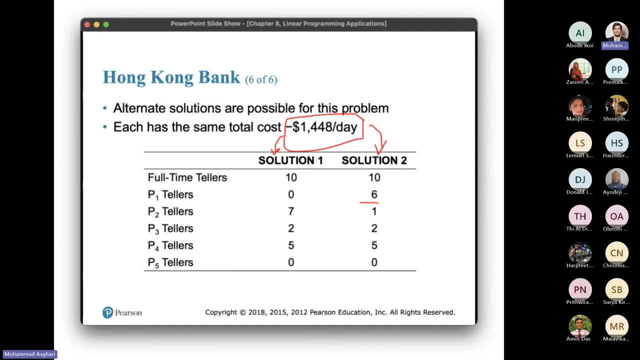 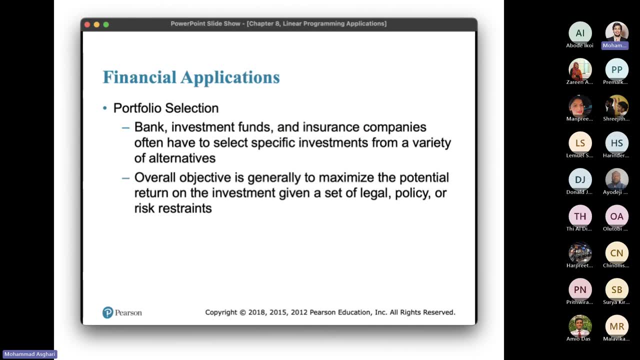 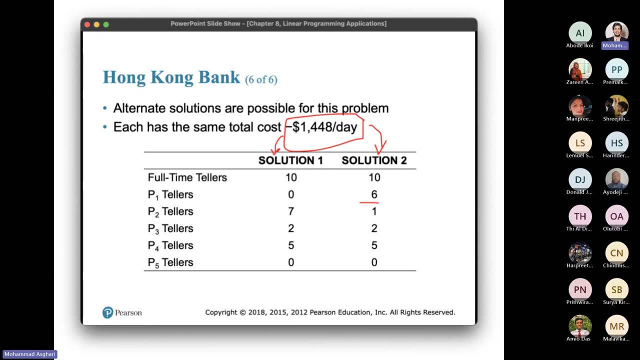 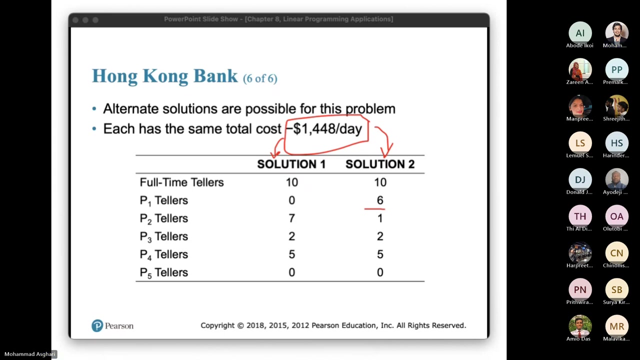 So there is no difference between them. We can use Any well? so Uh, this is optimal solution and uh, If you have any question, please ask. Uh, if not, we can continue. After solving, you will find that how many people you need, OK. 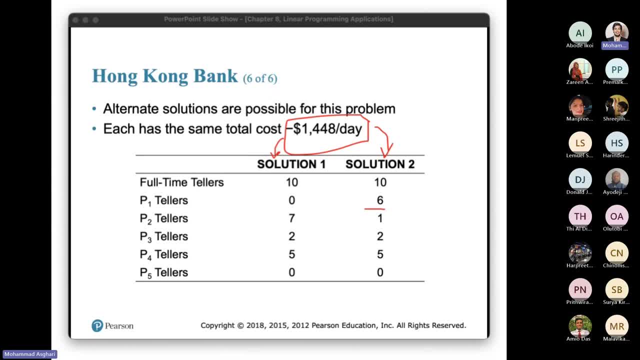 Uh. sometimes you may reach a different solution with the same objective function. Both of them are optimal, so you can go with this number of people or this number of people. solution to and Uh, The Both of them are- provides you with the same results, so you can. 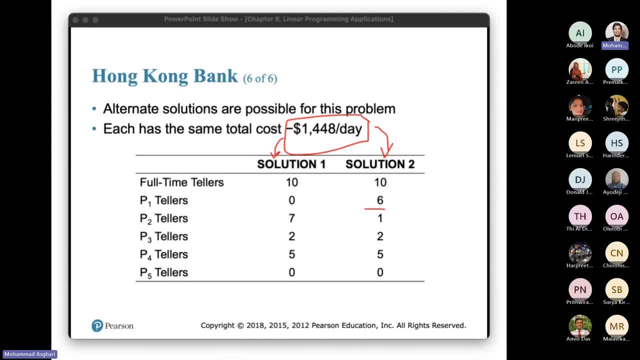 not implement both of them. So either this one or this one, You will take one of them. I believe that this, this type of this problem, is the most complicated problems, and so for final exam, I don't expect the problem Uh, to bring you a very complicated problem If you. 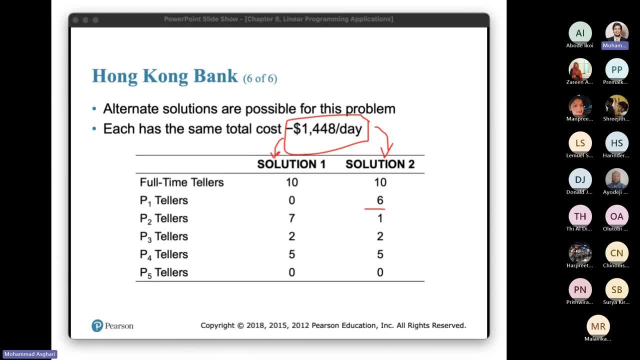 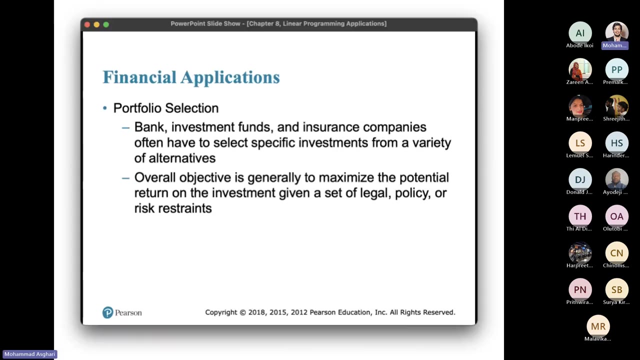 understand this problem. let's stop. Uh, it should be very easy. Uh, any questions from this category of problems? No, Sir, OK Garrett, thank you so much, So let's move on. Uh, this is Very easy. Uhm, so I'll just briefly explain it. Uh, we just. 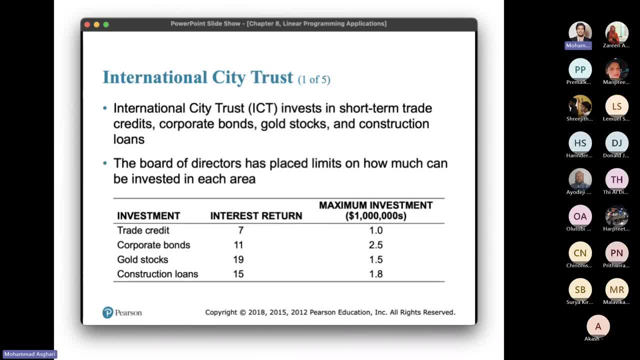 escape this one. Uh, so you have, for example, for options for investments in different areas, for example, three credit, corporate bonds, Gold Sox and construction loans. So each one have one has its own interest. Uh are will turn. For example, if you invest your money in third credit, you will earn 7% more after one year. 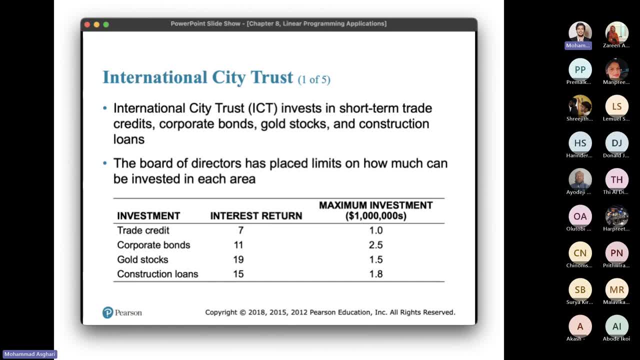 This is the maximum money that you can put in different investment options. All of them have been written in this unit: $1 million. You can just put $1 million in third credit, for example, $1.8 million in construction loans. 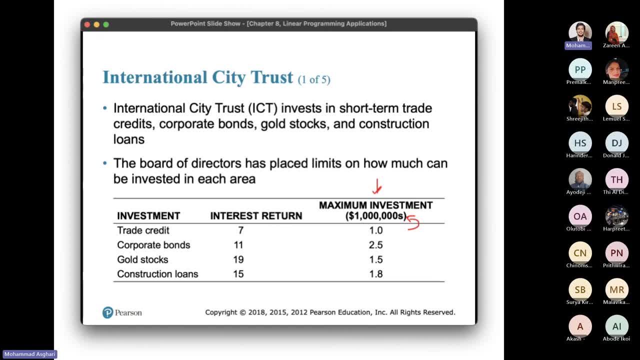 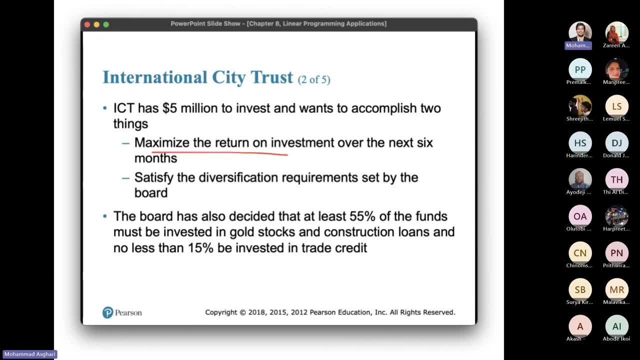 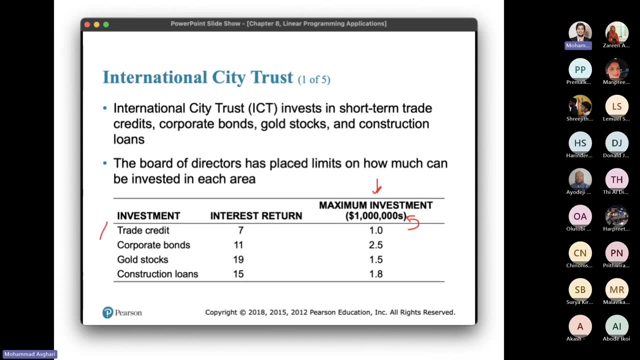 What is the objective function? We are trying to maximize the return on investment. We are trying to maximize the return on investment. That is easy. You just need to define the decision variable first- The amounts you invest in total credit- and call different options. 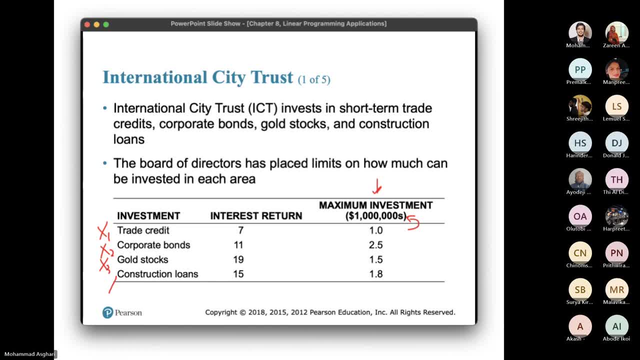 X3 and X4.. You can accelerate the objective function in this way. You just need to maximize the return on investment. Z. that is equal to 7% x1.. This is the maximum amount that you get after one year And 50%. 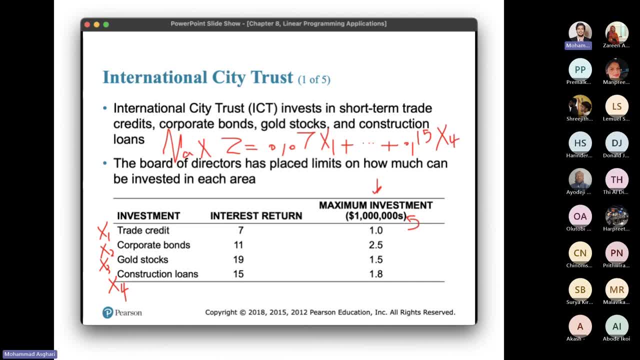 And there is a constraint. that was so. you just need to consider that x1 must be less than or equal to, $1,000,000. And x4 must be less than this amount. Okay, so we have a budget. This is the total money that we have. 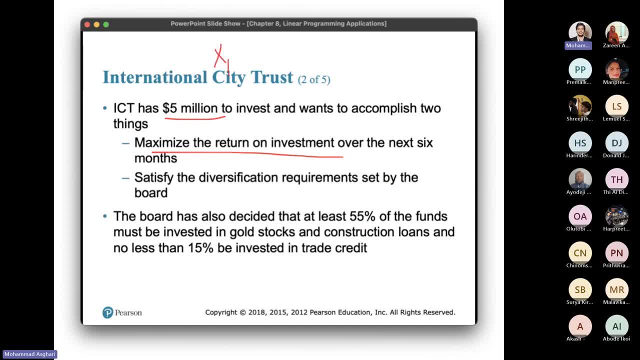 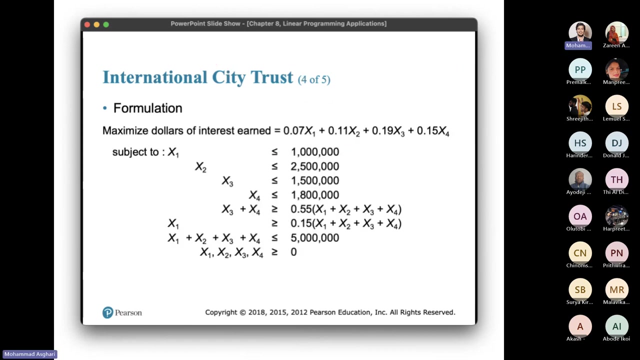 And we should get a summation of all money We are investing in different options. that must be less than or equal to $5,000,000.. This is the maximum budget that we have. This is the maximum money we have, So it is so easy. 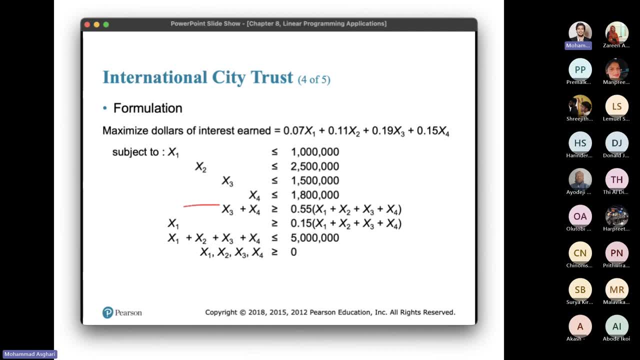 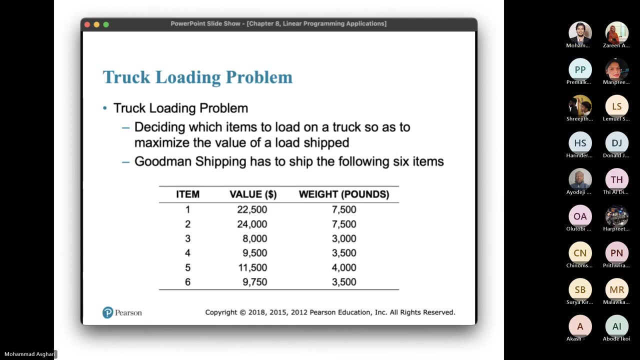 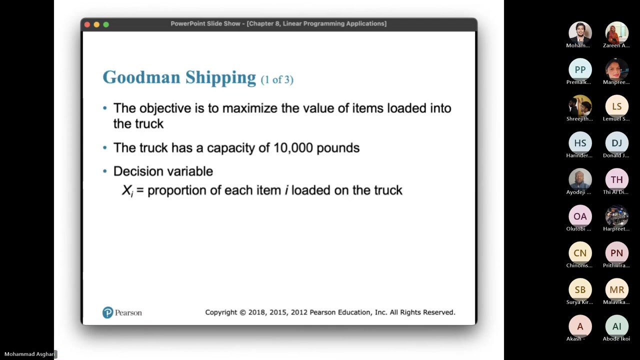 And we have two other constraints, So you can see them in the question here. This is so easy. Exactly the same as the previous ones. This is the optimal solution, So we don't need to This one, This one and shipping. 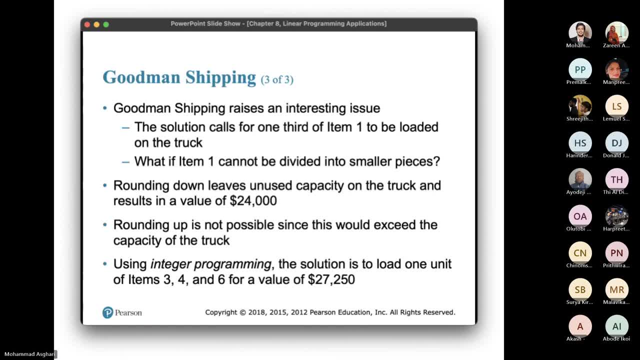 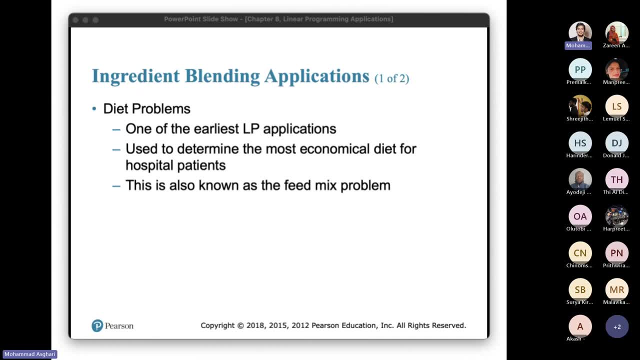 That is so easy: Ingredient blending application. So we had something similar before, If you remember. so we are trying to maximize the nutrition in the food And we have different types of ingredients from different brands, So we want to select how much to buy from. 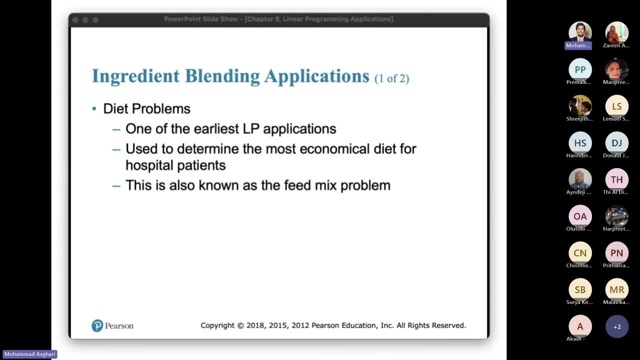 Or how much to add from different brands, So that we want to minimize all costs While ensuring that minimum amounts of items or minerals, vitamins, everything is included in the food. So very similar to this example. So, for example, for diet problem. 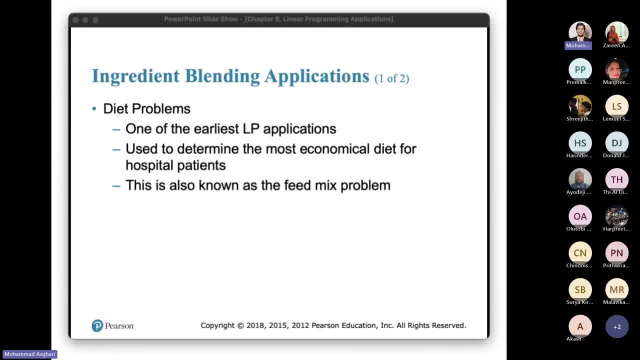 We want to make sure that we are eating enough items in a daily life, While you know that we have Look at the cost. So let's see that. What does this problem? talking about One of the earliest linear programming application used to determine the most economic diet for hospital patients? 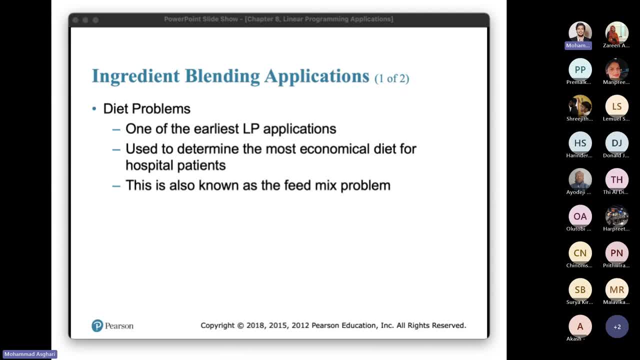 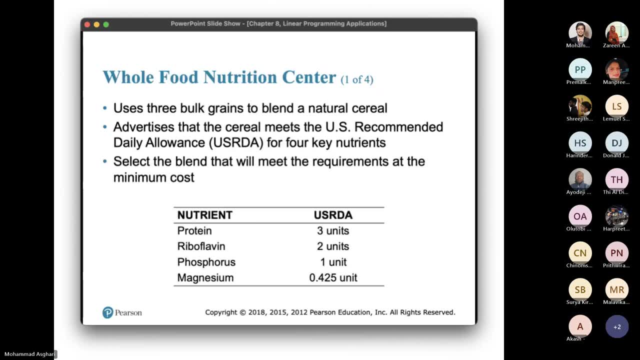 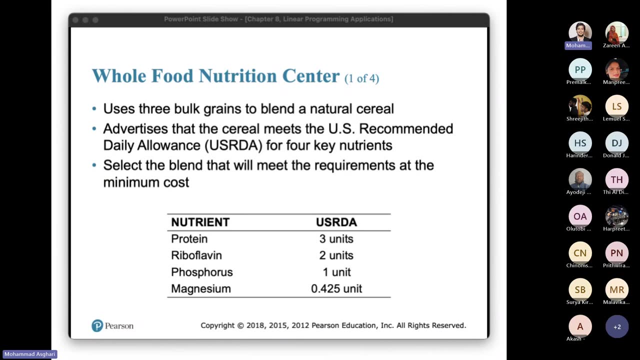 And this is also known as a food mix problem. Let's see what is the problem. Uses three bulk grain to blend in natural cereals, So we have to mix three different items to bulk rate. So these are the something that we should select from advertisers. 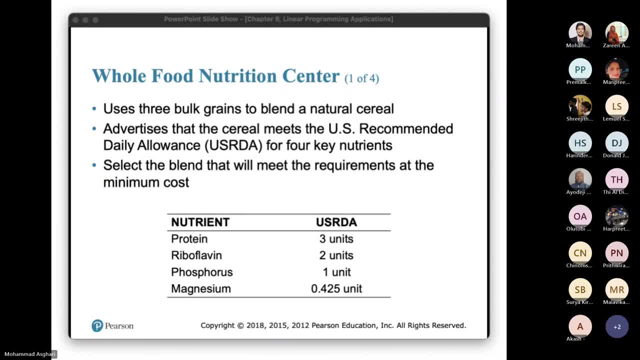 The first, it's the food mix. The second: we should add some crudes to the bulk. You see theін At cereal in meet the listed USA recommended daily a loners, As you can see here in this color. Your daily life needs protein, needs a riboflavin. 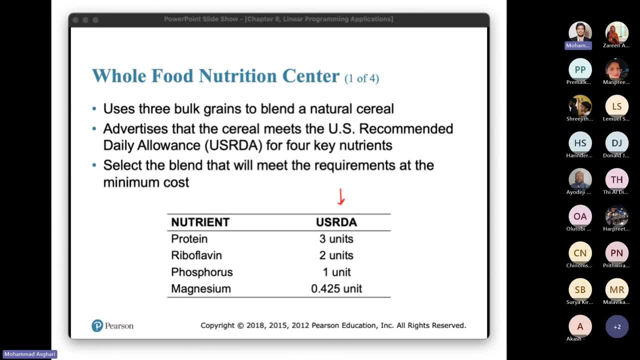 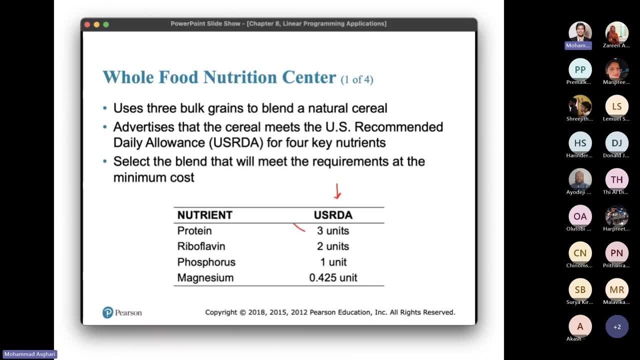 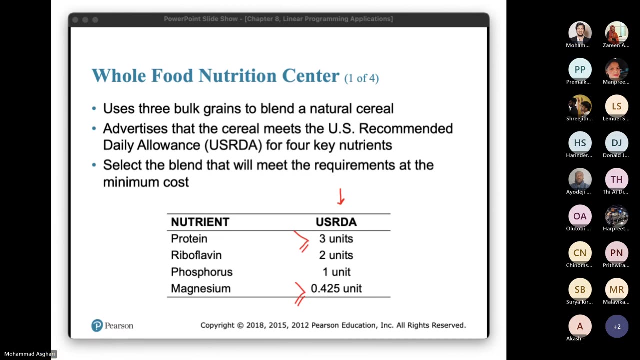 Phosphor magnesium. So so you should make sure that, every day, you are eating at least this amount, at least this amount. This is a requirement, So you should eat this amount of magnesium, more than this amount your body needs. Okay, Whatever You're going to write, it should be greater than or equal to this amount. All of items that you are eating per day, they should have at least this amount. 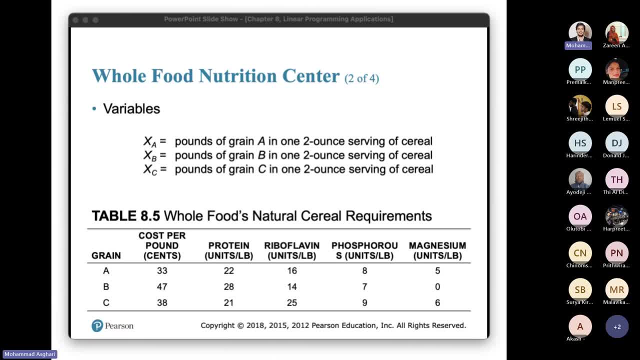 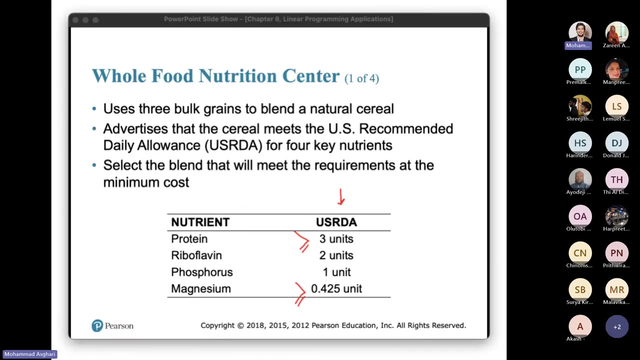 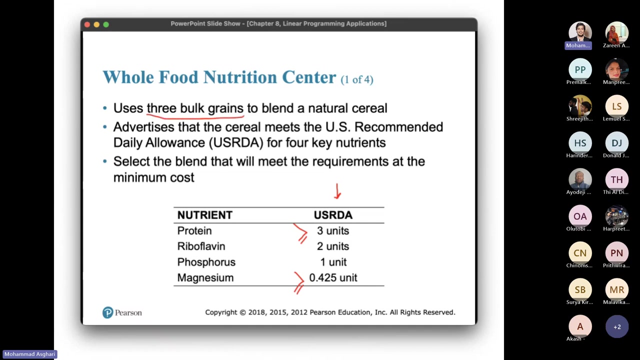 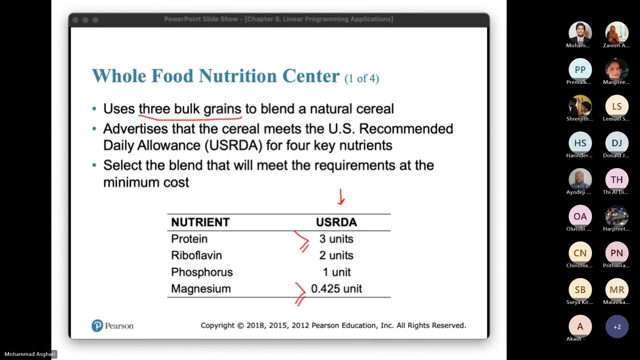 So first we have to decide about variables. So this problem includes two different types of variables. Okay, So each of these variables will be referred to the amount of pound that each ball going As in order to save the the cereal. So, if you remember, here we have two different bulk goings, So there are two different that you know bags, for example. you should select one from each of these bags. 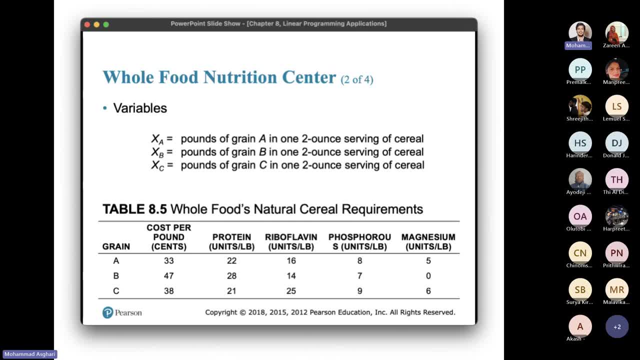 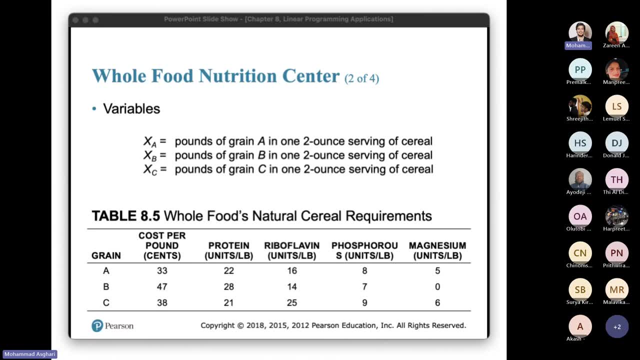 Each of these three bags, For example, bags A, bag B, bag C- How much you want to buy. Some people sometimes do mistake and consider variables for the amount of protein and others. For example, they say X1 for the amount of protein, X2 for other items. 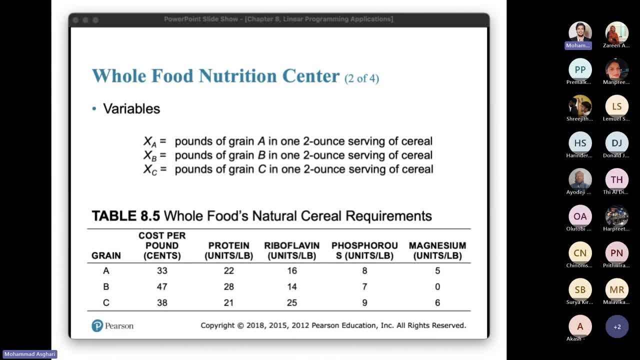 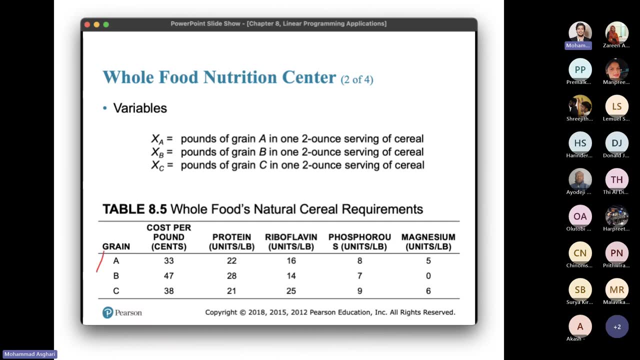 So be careful, As I told you, if you do mistake in the first step, the rest of your work will be, you know, useless. Your variable will be how much you will pick from this bag. Define the X8. How much you will. 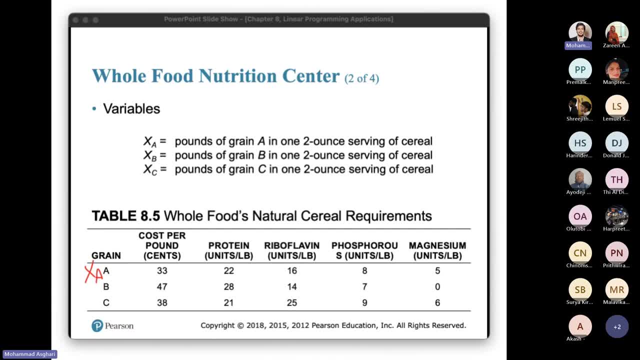 pick from this bag Number one, bag A, What can go in number one and how much you want to get from this. bag number two is B, So we have two different bags. Okay, each of these bags have certain amounts of ingredient. for example, 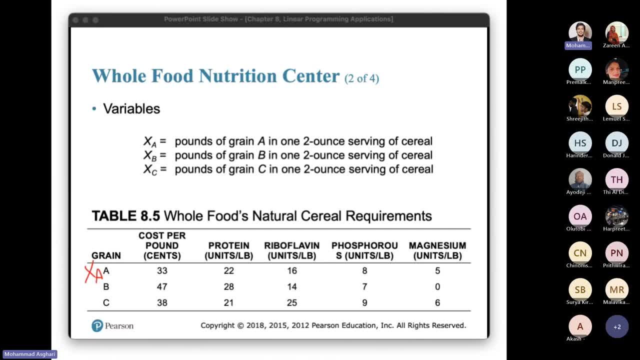 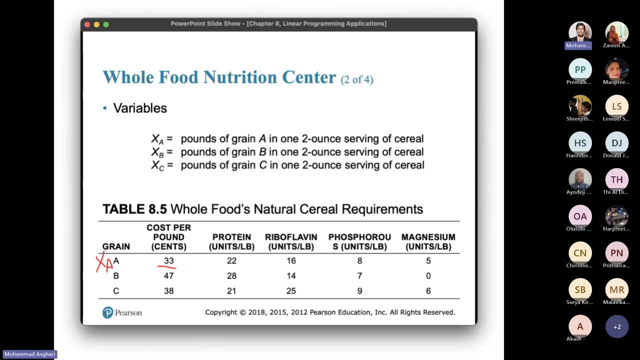 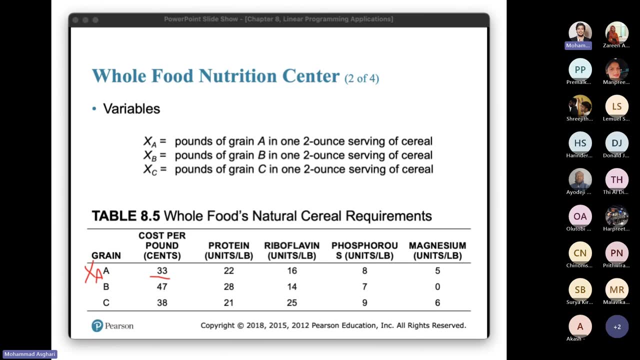 For example, bag A, which costs you 32. Cents per pound, Whatever. So it has 22 units per pound from protein, Let's see. And also for other items. So, each of these, each of them, each of these, 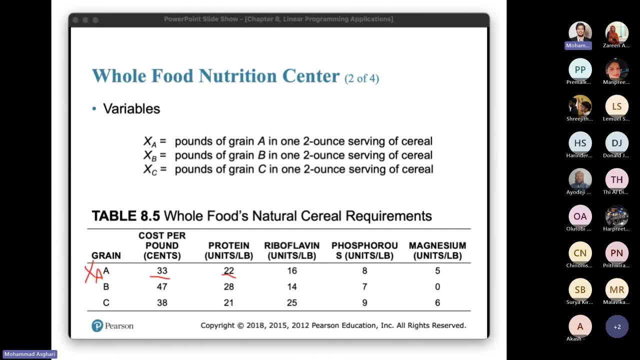 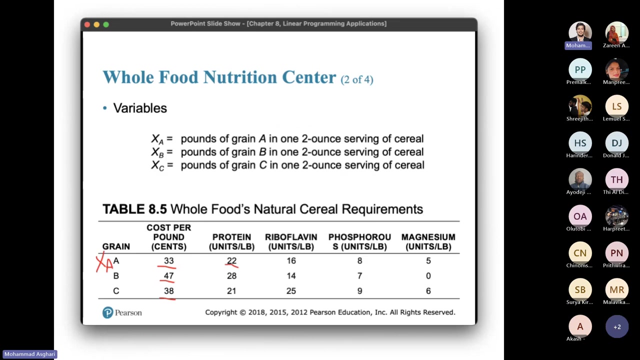 grains are are coming from a certain price. You can see the price in this column. So so price is good to use in the objective function or in the constraint objective function. So how should I write the objective function? It is so we are trying to minimize our cost. 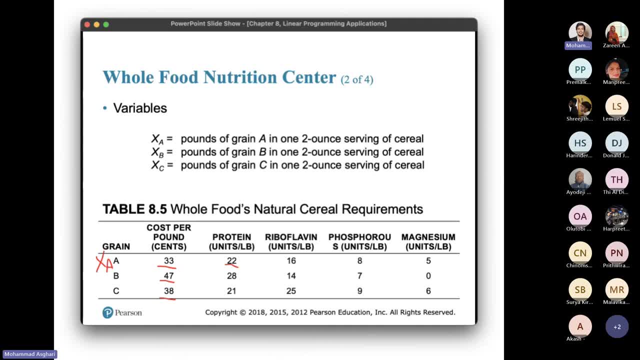 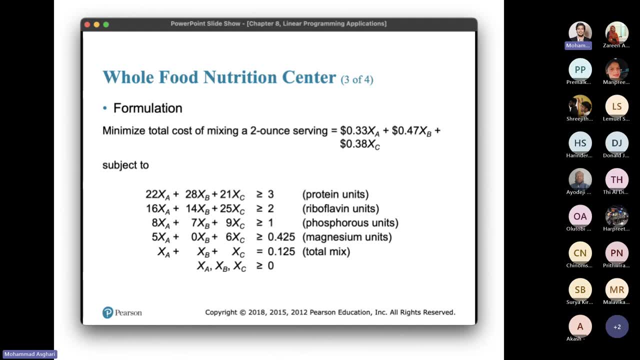 And what is the cost of each grain. So this is the amount of a grain A. You just need to multiply it to the cost of a grain A And get a summation of them. This is the minimum. this minimizes total cost and we have some constraints. 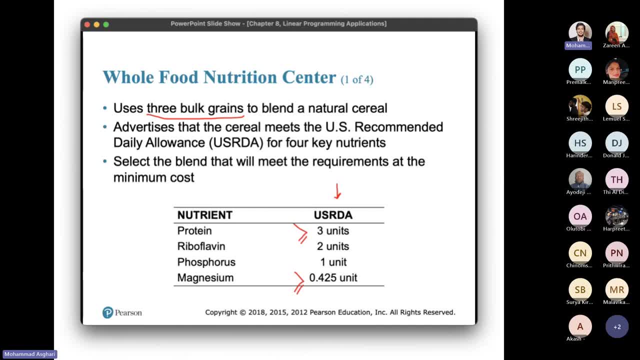 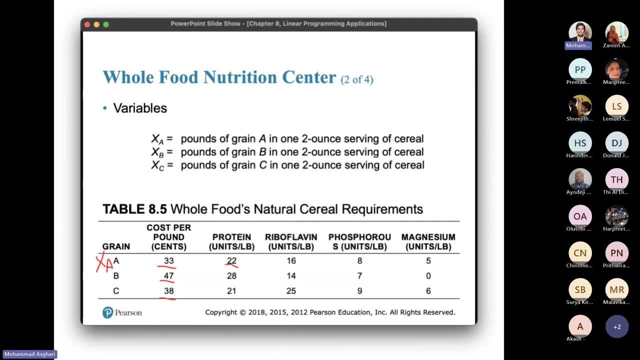 So, for example, we need this amount of protein- Protein Um- per day. So, uh, we know that each grain has a certain amount of protein: XA Multiply 22 units per pound, and XB Multiply 28.. 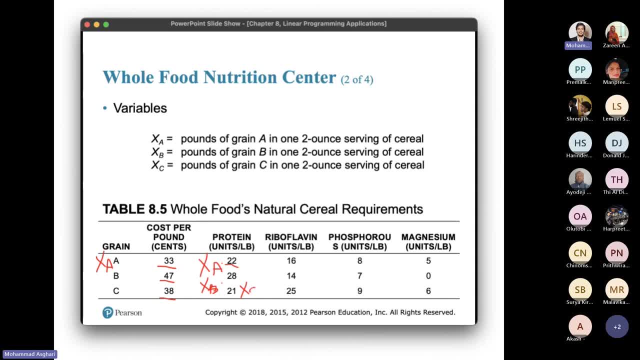 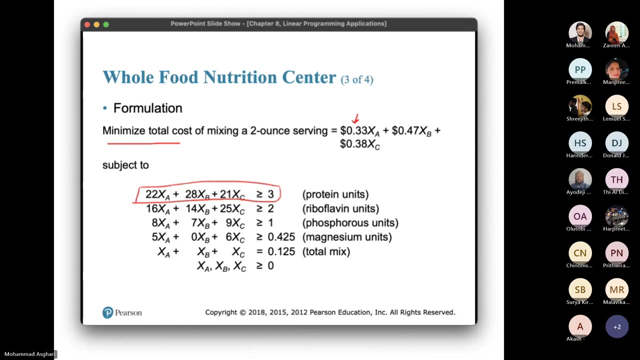 And XC, Uh, uh, C, Multiply 20.. One, If you get a summation of them, they must be greater than or equal to these numbers. Uh, three units, As you can see here. So we just multiply the amounts of protein in each grain, uh, and the amount of uh. 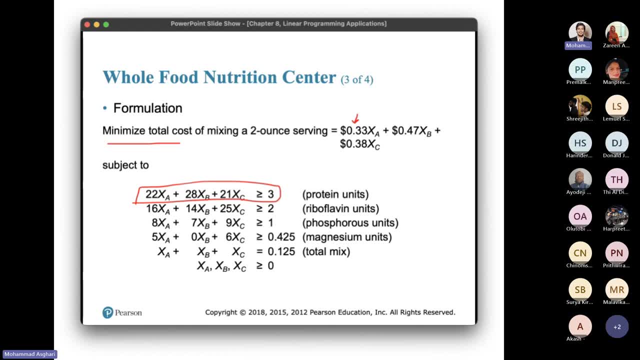 the amount of grain, the pound of grain, if you get a summation of them, that must be greater than or equal to three units of protein. So this is all we have in this table for different nutritions. But we have another constraint here that has not been mentioned in the question, this one: